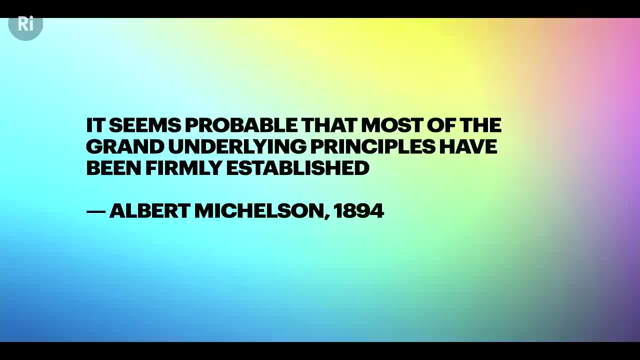 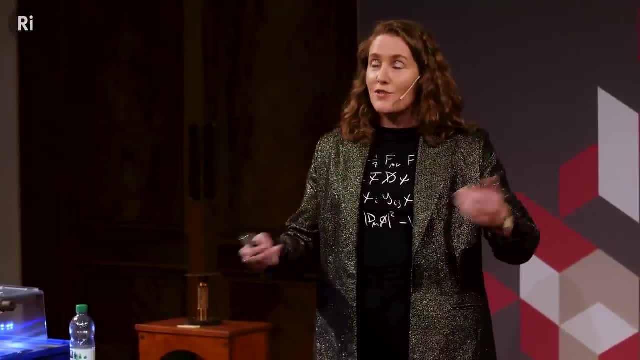 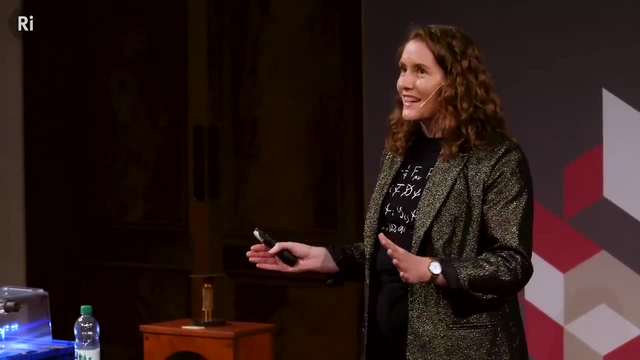 well, we can just take our theories of physics, so Newton's gravity, the idea of atoms, the chemistry that they knew about and the equations they had that described, that turn the handle on some maths and predict the future forever. Now I don't think it's giving away any spoilers that happen in the. 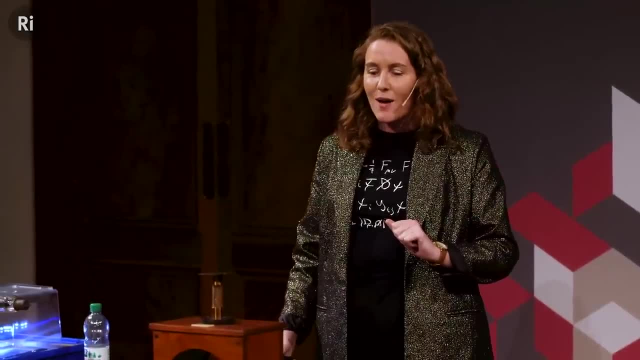 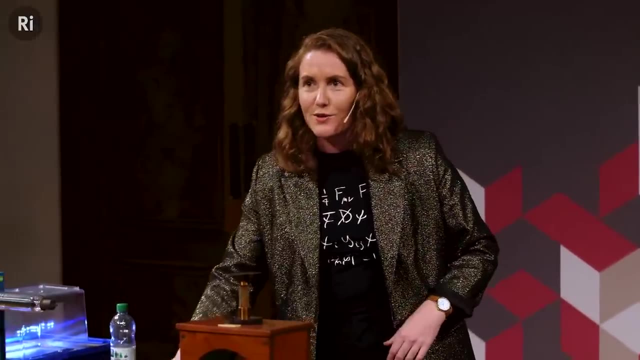 book to say that that's clearly not how things turned out, And so the 20th century in physics was an enormous decade of change. Now, as we go through the story today, I'm going to try and share with you some of the stories and some of the things that I learned. 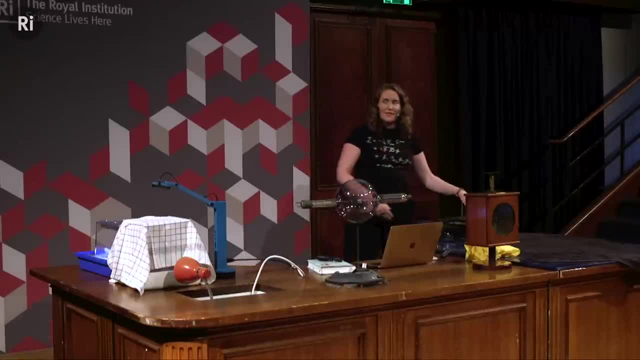 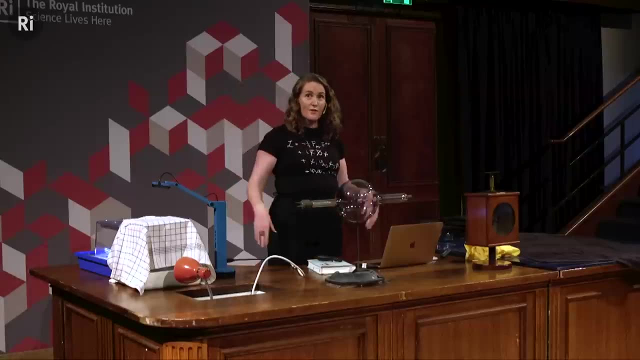 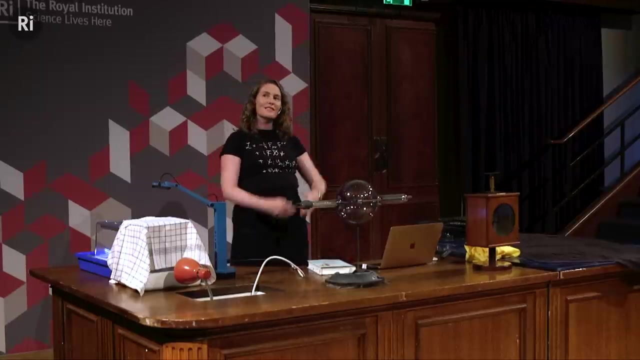 as I went through and wrote this book And I feel like we often treat scientists and physicists especially as like putting them up on a pedestal, especially the theoretical physicists, who I'll mention none of tonight. So the reason I've just taken off my jacket is because I want to just 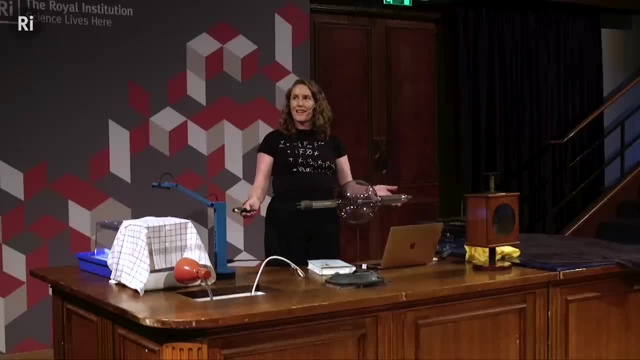 chill out a little bit and bring physics down to earth, down to the human level and down to this how it is. we walk into a room, into a laboratory and discover new things about the universe, And I hope you'll enjoy coming on that journey with me tonight. Right, so in 1900, actually maybe. 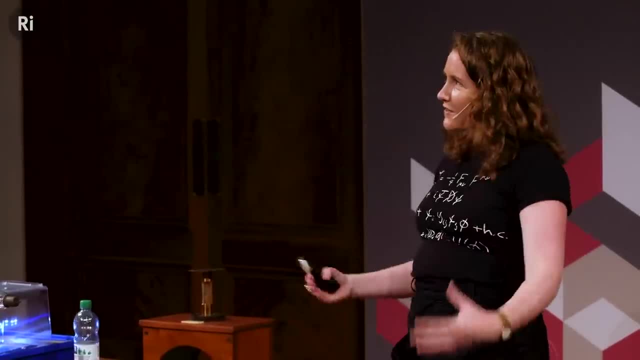 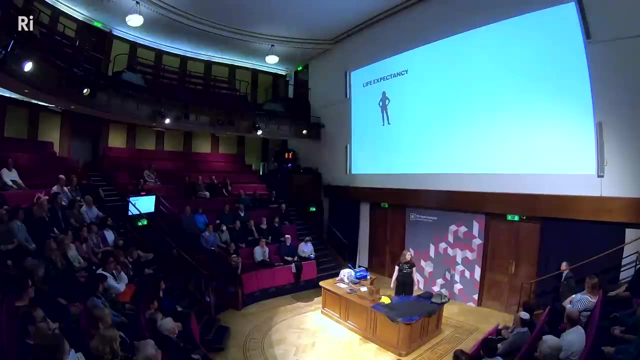 I'll ask you this question because this is, you know, an interactive kind of venue. Does anyone know what the life expectancy was of people in 1900, roughly? Someone's saying 50.. Someone's saying 50. Yeah, yeah, 35.. So about 46.. Hopefully that's that's in the UK actually, you know, obviously a. 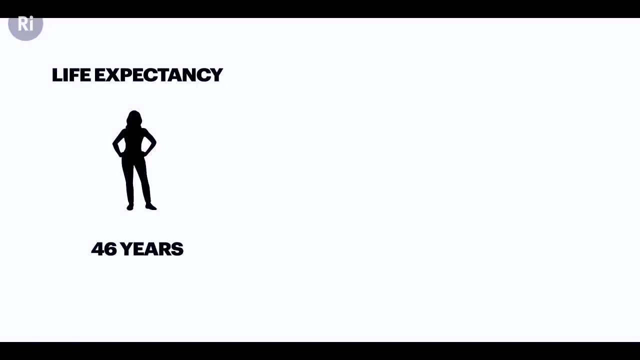 well-developed nation at that point in time. Fast forward to today and the average life expectancy is 81 years. The UK population in around 1900 was 30, yep 38 million. We're currently sitting at about 67 million. That's not such a huge increase, right? They're pretty. you know they go with each. 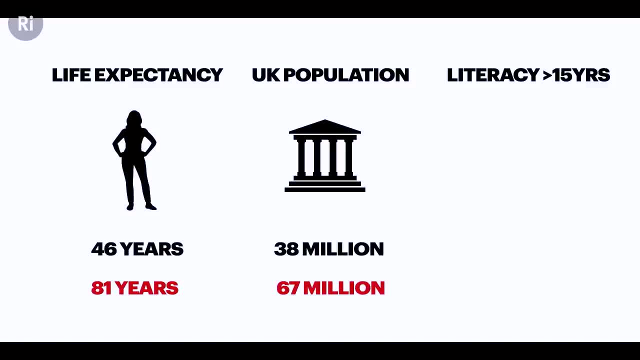 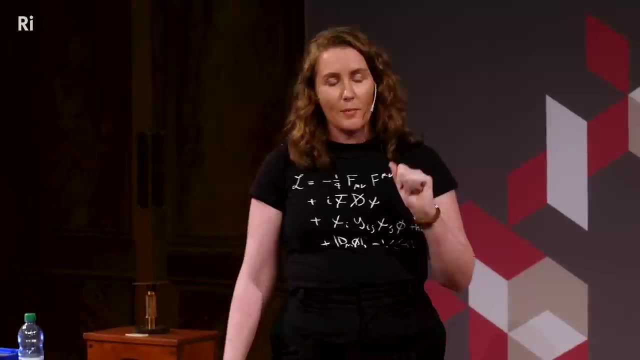 other. One of the other markers of change that's happened in the last century is in the area of literacy, So the literacy of people over the age of 15 years old. Now I'm going to give a global statistic that at the start of- at around 1900, literacy was at about 21% globally And that 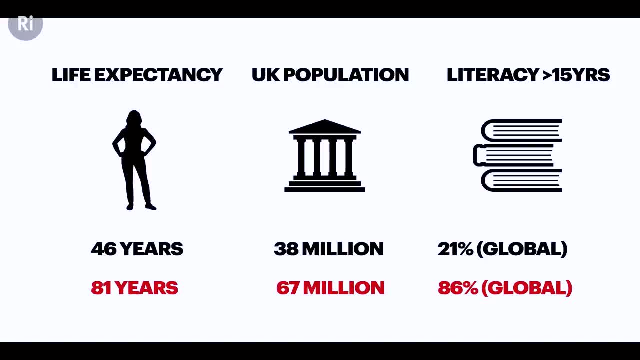 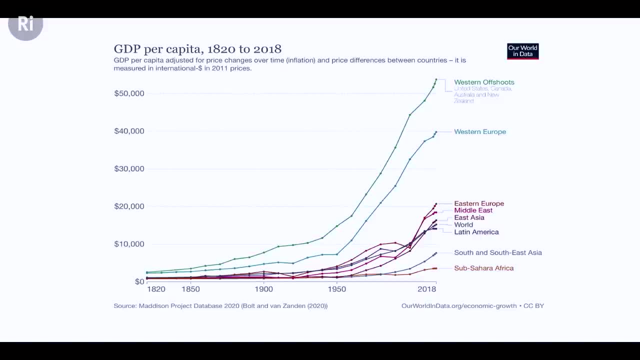 number is now at 86% globally, which is an enormous change, And so I'm setting the scene here a little bit to tell you how much our society and our world has changed in the last century, And I'm going to talk a little bit more about that in just a few minutes. So I'm going to talk a little bit more about 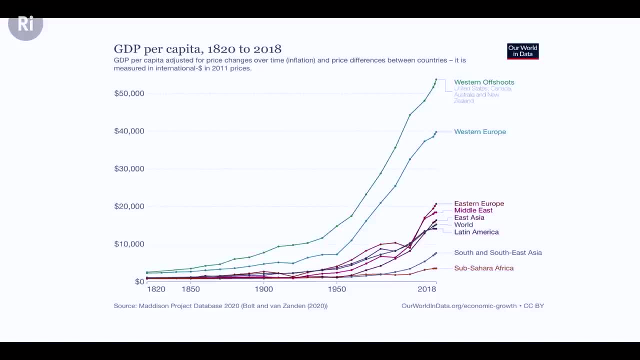 what's happened in the last 100 years And one of the reflections of that is in the GDP per capita, which has sort of been normalised, and et cetera, et cetera, to create this plot just showing the enormous change and growth that we've had over time. Now this, this is easy to 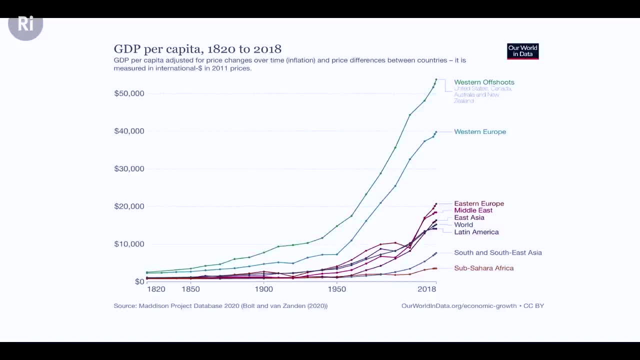 sort of look at and say, okay, well, clearly, you know, obviously that was going to happen, right, And we tell this story and we talk about innovation and we talk about businesses and we talk about- we don't normally talk about- physics alongside it, right, But tonight I'm going to try and do that. 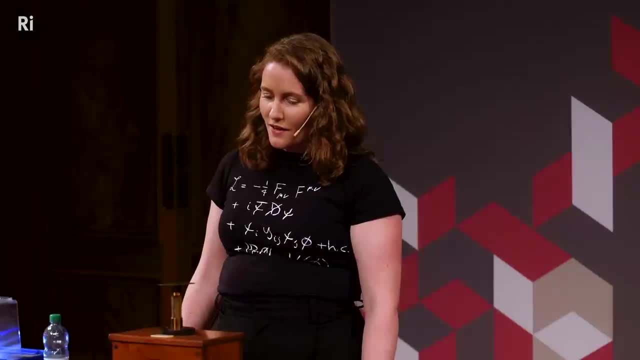 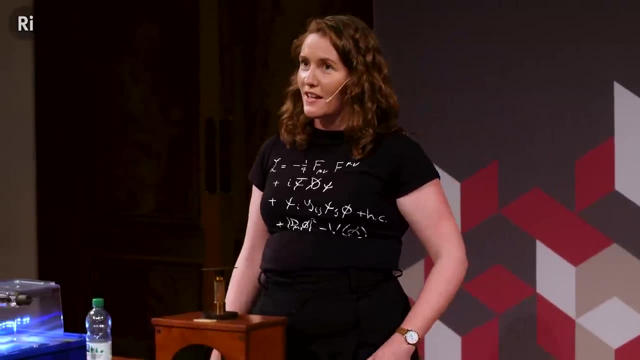 and connect these two things together. Now, if I was to ask you in 1900 what the future would look like, it would be very hard to predict, And even cutting edge physicists at the time found it difficult to predict. So this is a quote from Lord Kelvin, who was a famous physicist at the time. 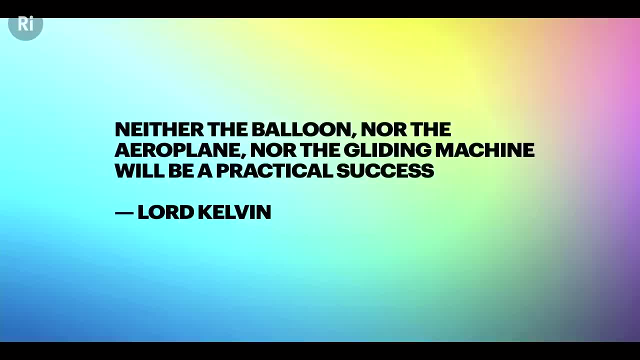 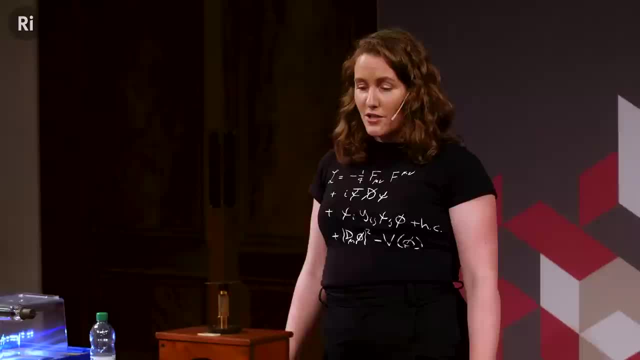 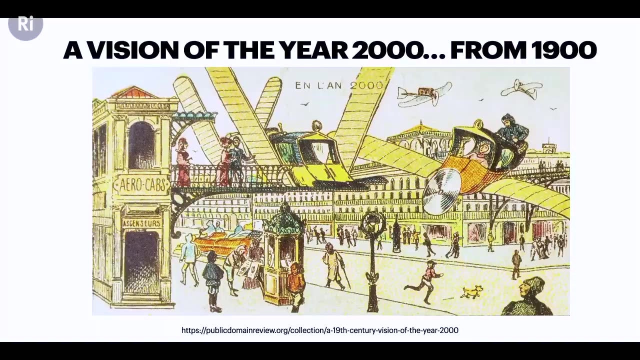 who thought that neither the balloon, nor the aeroplane, nor the gliding machine will be a practical success. Actually, in 1900, for the World Exhibition in Paris, someone did ask a bunch of artists actually to predict what the year 2000 might be like from that point in time, from 1900. 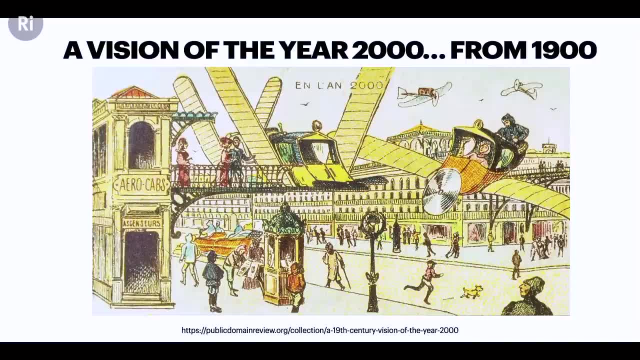 This is what they created. So you'll notice that there's flying vehicles, but propellers were sort of only recently invented And so everything had a propeller or maybe some flapping wings. People's outfits hadn't changed much. Architecture- there's at least one architect in the audience. Architecture hasn't changed much. 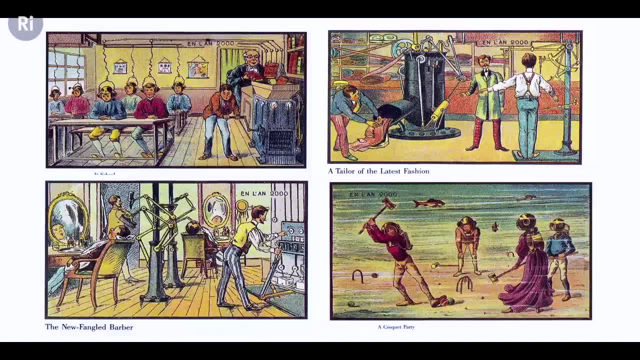 There's no vehicles. so clearly they predicted that incorrectly. Let's look at some other aspects of society. So let's think about information transfer. So information transfer was done electrically somehow, But the production of goods was an interesting one. So the prediction of the production of goods there was, of course, 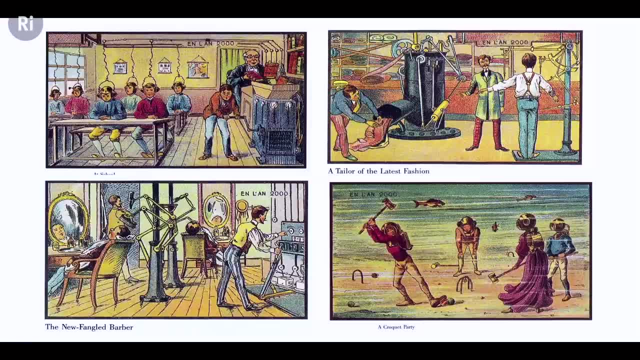 many factories at that time in horrible, horrible working conditions. But they sort of predicted that automation would come from like mechanical means. right, There was no prediction of electronic means of automation at that point in time. And that goes for the barber as well as the what's the person who? 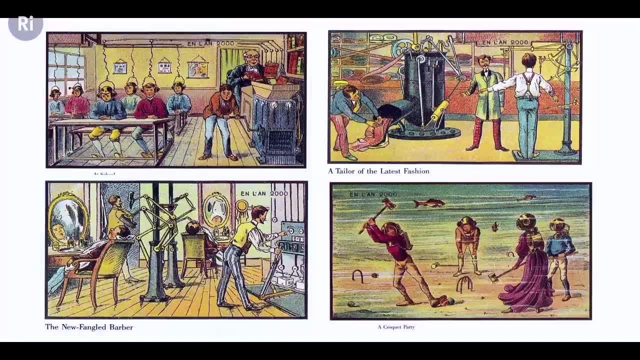 makes a suit. called Those people, Taylor. thank you whoever said that. One of the particular fascinations that just struck me as funny is lots of these postcards envisioned us living under the sea, And you could almost translate that to where we've ended up thinking about. 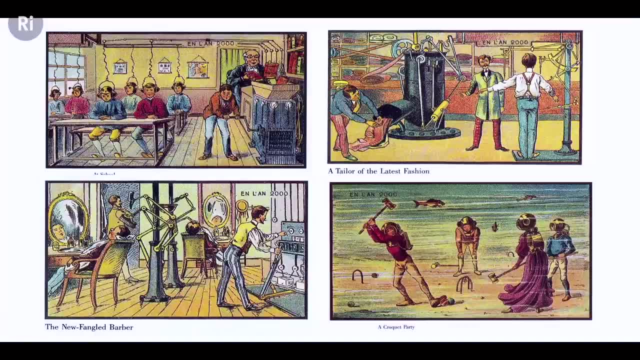 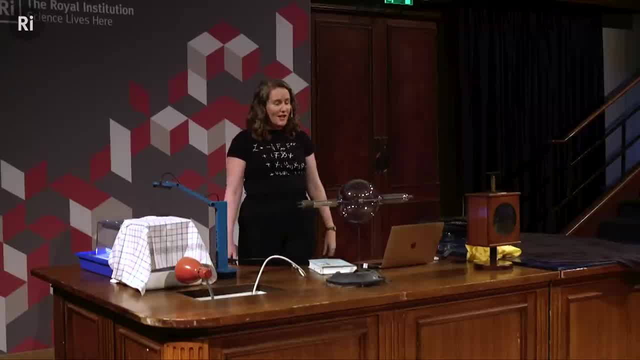 up in space. only we don't play croquet up in space, Anyway. so this was the prediction at that point in time, And I'm not going to embarrass you by trying to ask you what might happen in the next hundred years, right. But I think it's important to come back to this idea that at this point in 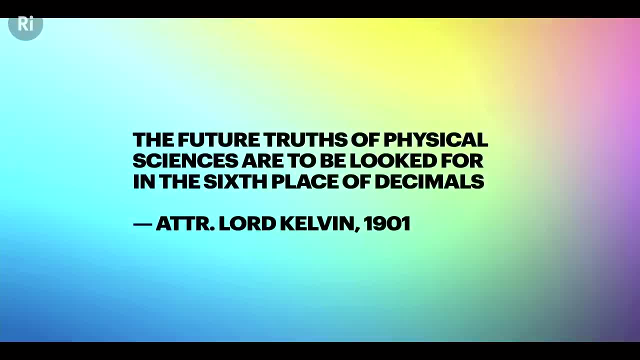 time physics looked like it was done. And again Lord Kelvin says the future truths of physical sciences are the future truths of physical sciences. And I think it's important to come back to this idea that at this point in time, physics looked like it was done. And again Lord Kelvin says the future truths of physical sciences are: 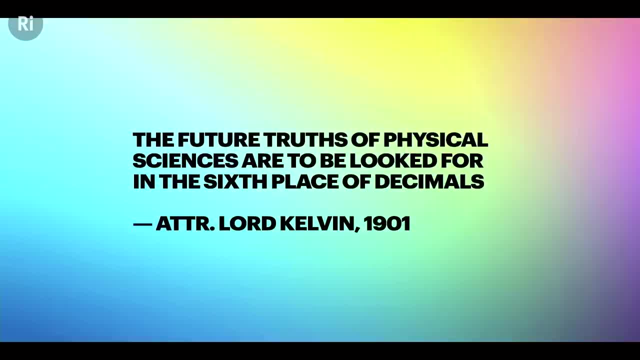 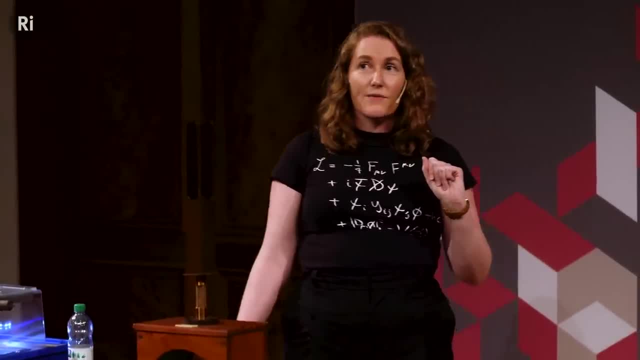 to be looked for in the sixth place of decimals. In other words, there's really nothing new to discover. Fast forward to 1895, 1896.. Now, in 1895, radioactivity was discovered accidentally by Becquerel. 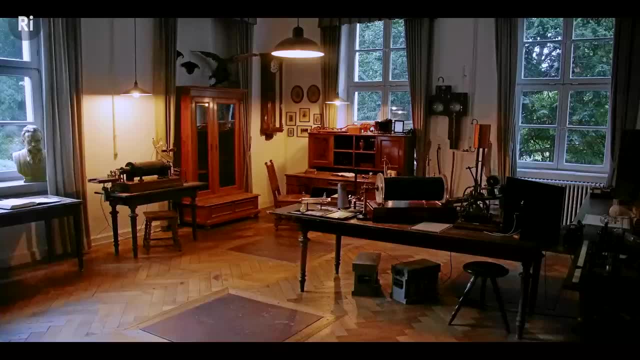 And then in 1896, this is what a lab looked like. This is Willem Roncken's lab in Germany, in Würzburg, And you'll notice- for those of you in the room- it looks awfully similar to this room. 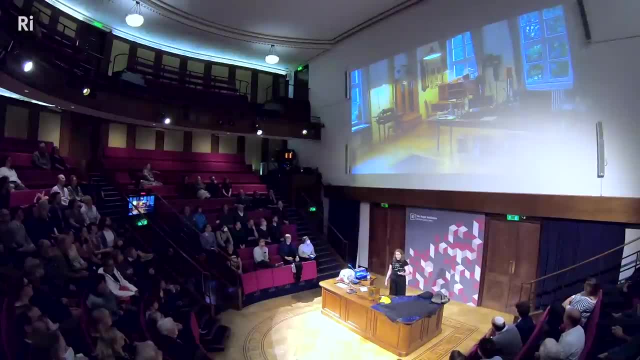 doesn't it Like I noticed that resonance when I was looking through my slides before? Phenomenal. This is a living financial mechanism. There's a beautiful highий flooring, the beautiful wanting windows. It's really a lovely environment. I think we should bring back labs that look like. 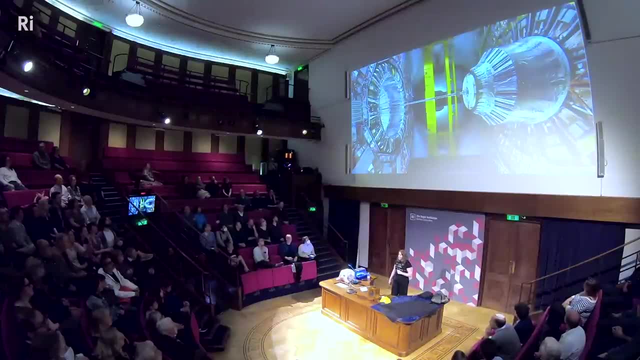 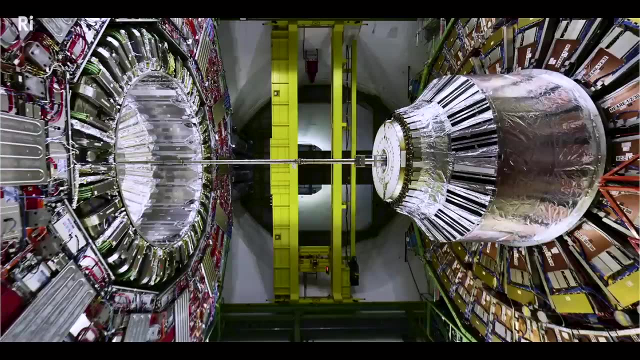 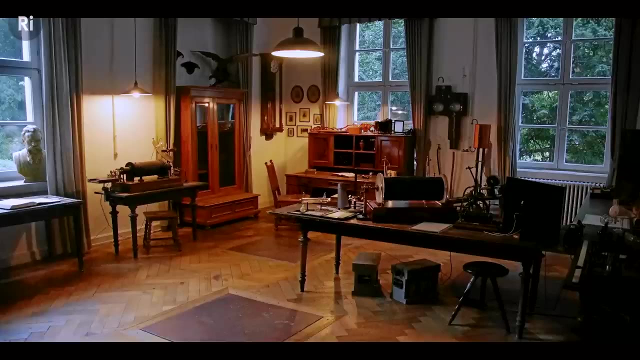 this personally. Now, today our labs looked like this: right, This is a compact muon solenoid, the CMS detector at CERN. It's an enormous experiment. I will talk a little bit more about this kind of thing later on. So how did we get from a lab in Würzburg to enormous machines? like the Large Hadron Collider. How does that relate to the question of you know, is it this big of an issue for the findings, Or is it huge because this is so small? It was so out of the blue And you'd not be able to see it until still And you'd have people just trying to help out. you know, It was a really nice environment, But maybe there were a little bit of photographed. 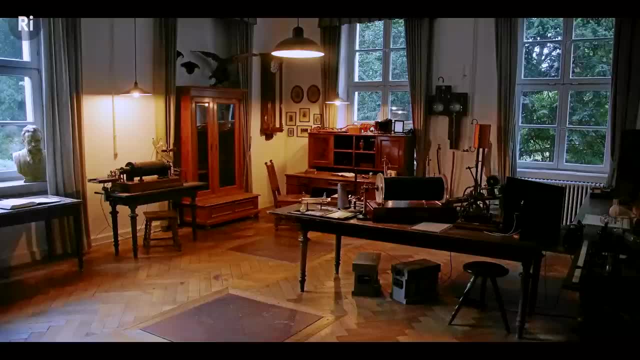 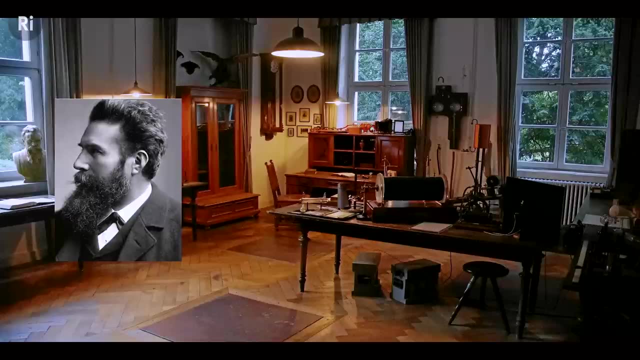 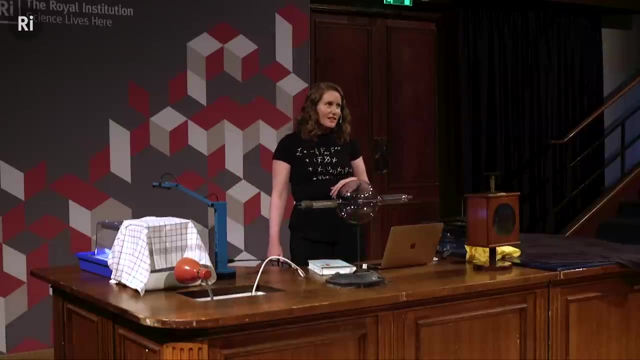 relate to this question of societal change in that time. Well, let me start with this person. This is Willem Roncken. I hope he's up on the screen. Yep, He was a very shy man but he was good at building things with his hands And he was a bit. he wasn't a very nice lecturer actually. 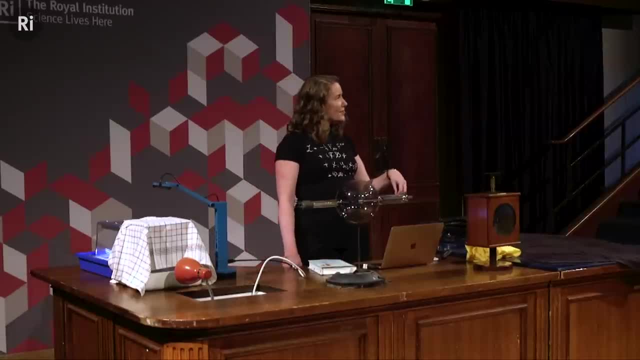 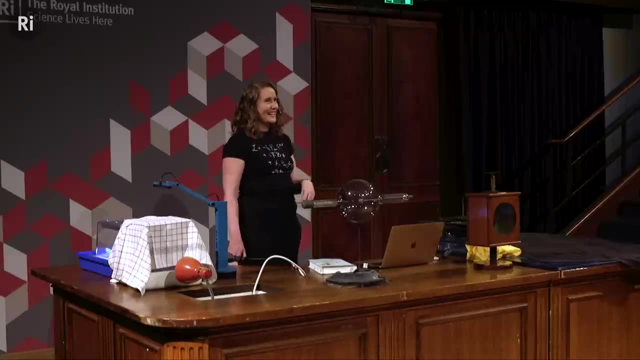 He used to speak in a really quiet voice so that all of his students had to sit in the front row and listen really carefully. It's really annoying, isn't it? That's how he used to speak, so that he had the full attention of his audience. When he was in 1896, he was playing with a tube. 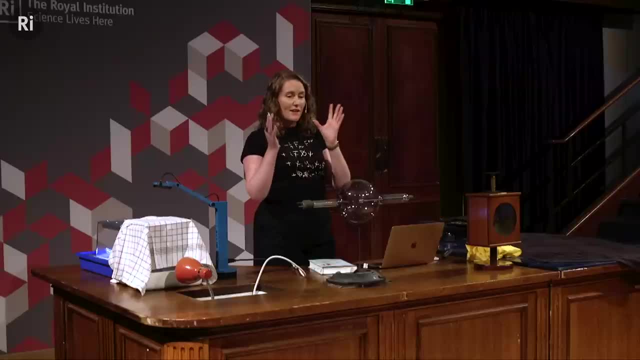 that looked something like this And this is a Crookes tube from the collection here at the Royal Institution. And at this point in time- around the turn of 1900, they were very common objects. Now this one has a particular use, But around that time they were used to study. 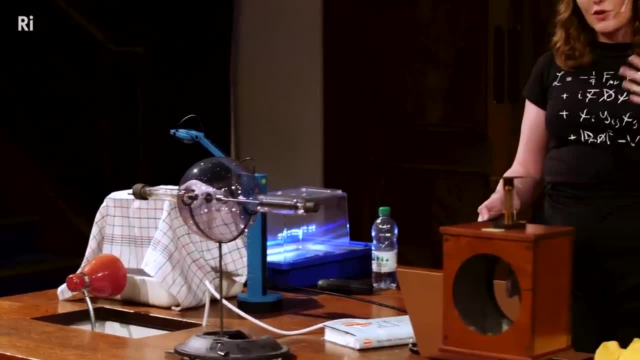 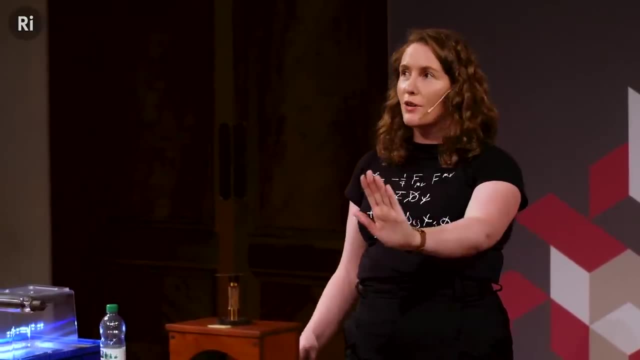 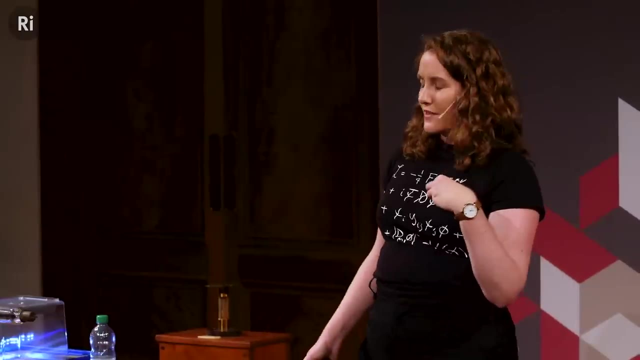 electricity and gases pretty much. And so he had these tubes in his laboratory, And one day he was using it And he noticed a screen glowing across the other side of his laboratory, a fluorescent screen. Now, Roentgen had a trained mind in experimental physics, So instead of just sort of saying 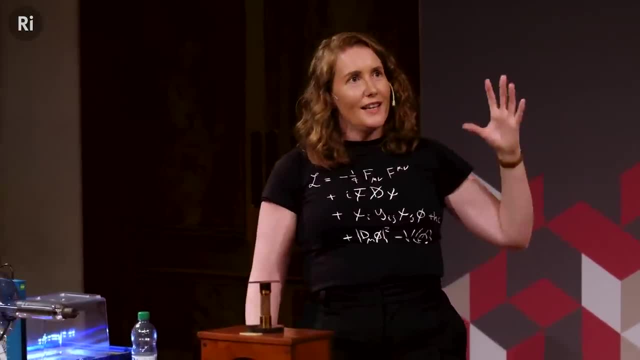 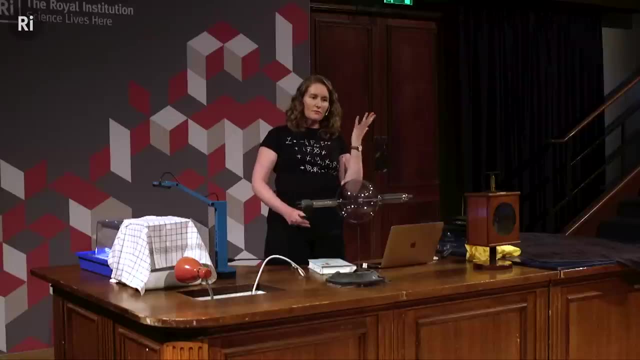 oh, I didn't expect that. I'll just ignore that and go back to what I was doing. he paid attention, right. So he switched the tube off and the light went away Back on. the light came back on, Oh, okay. So he got curious. So he thought: oh, I wonder if I put. 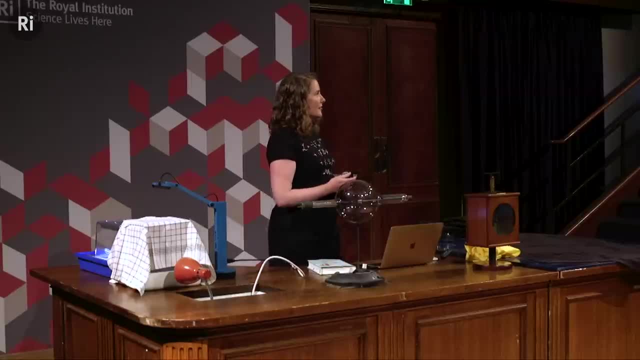 something between the tubes And he said: oh, I wonder if I put something between the tubes. And so he thought: oh, I wonder if I put something between the tubes. And so he looked at the tube and the screen whether it would still glow, And it did. He put some wood there. 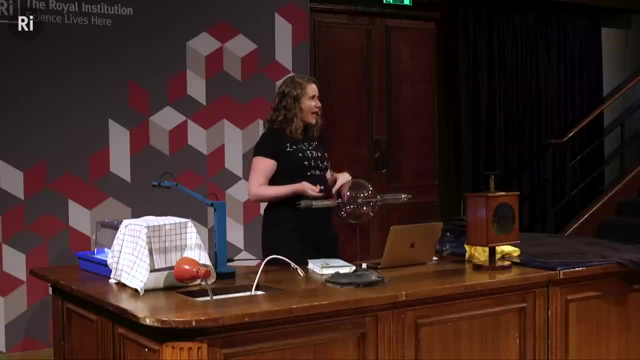 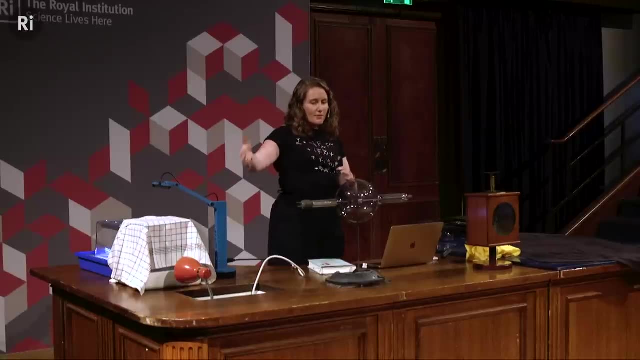 and he put some rubber, and it did. He sent it through the door to the next part of his lab and it still glowed. And then he put some metal in front of the tube And it stopped the glowing, And so he realised he'd found something completely different from the glow. 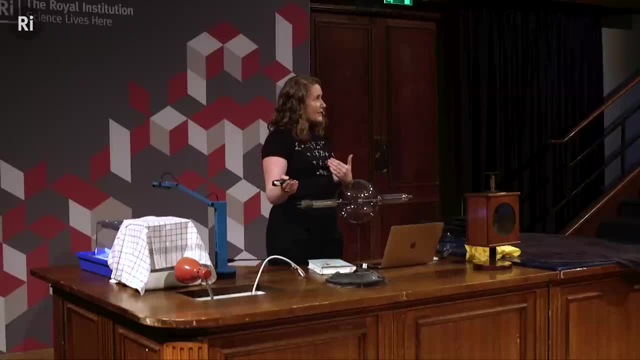 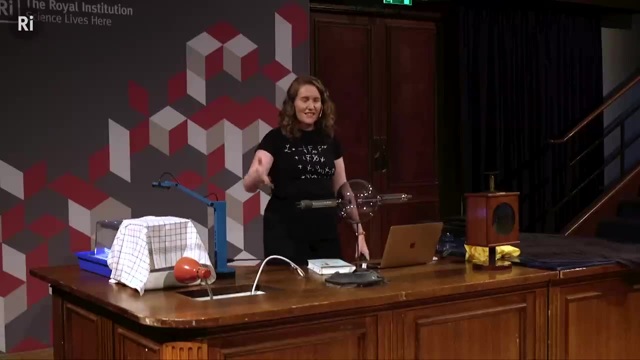 that happened inside this glass tube, And he was observing something completely different from that, And so he put his hand, as all scientists would want to do. we're just sticking our hands in there, you know that's how we work. So he stuck his hand in between the tube and the screen, And what he 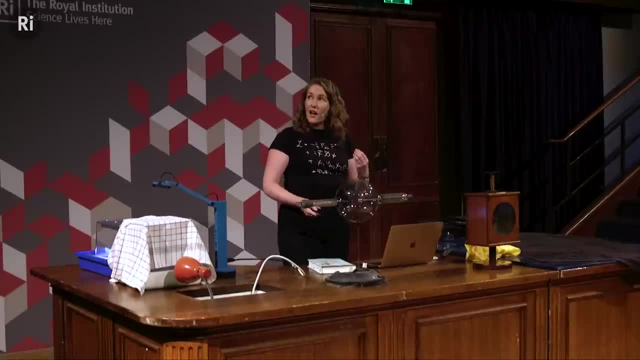 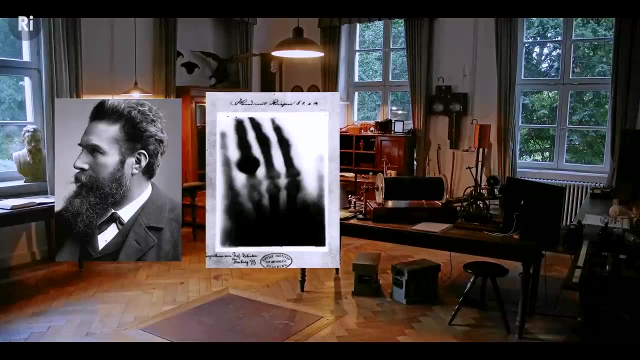 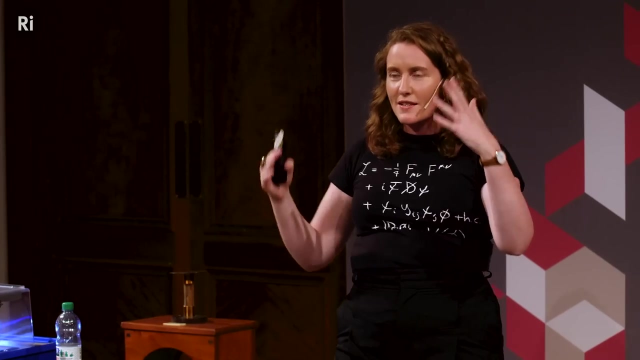 observed was that he could see the dark bones of the hand but not the flesh around them. And then he grabbed his wife, Bertha. He spent about seven weeks in the lab, by the way, investigating this, And Bertha, his long-suffering wife, would bring him food. He didn't tell anybody. 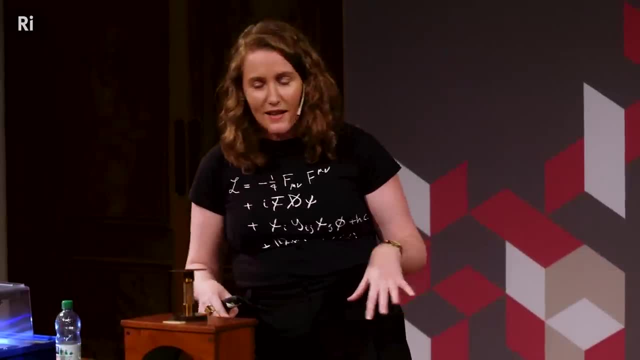 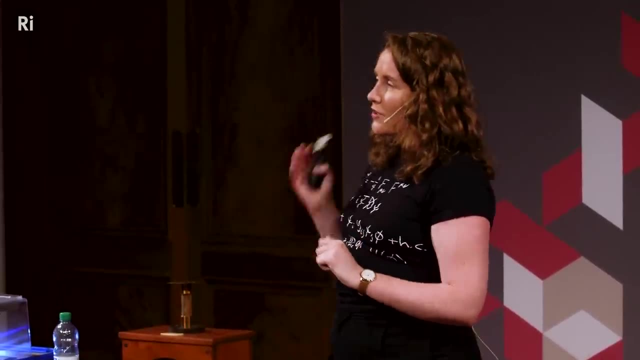 what he was doing. He worked very much alone. He didn't even like having assistants, which is a rarity even in those days. He was a bit of a recluse, but we've already said he was a bit of a strange man, And so he stuck Bertha's hand in front of the thing and he took a photograph And 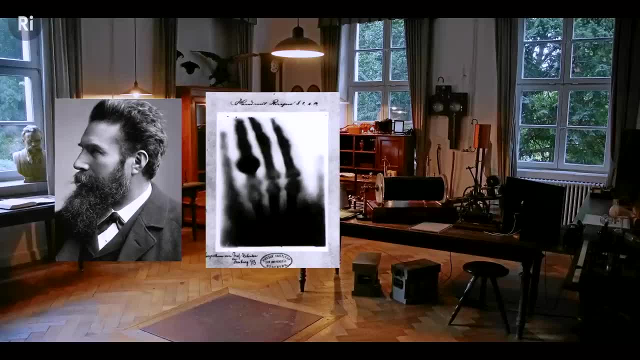 this is the photograph that he took of her hand and her ring, showing that he could see the bones inside the hand, not the flesh, And this, of course, is, as you will all know, watching. this is the discovery of x-rays, which we now know and love. 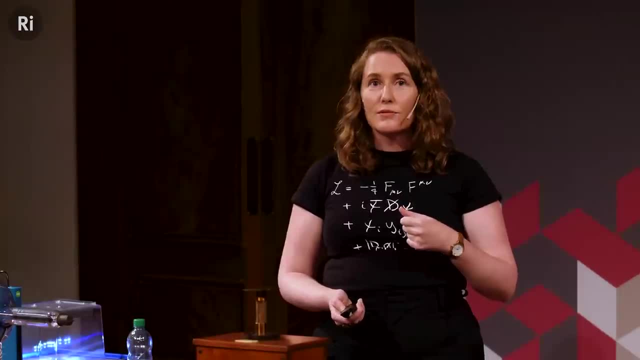 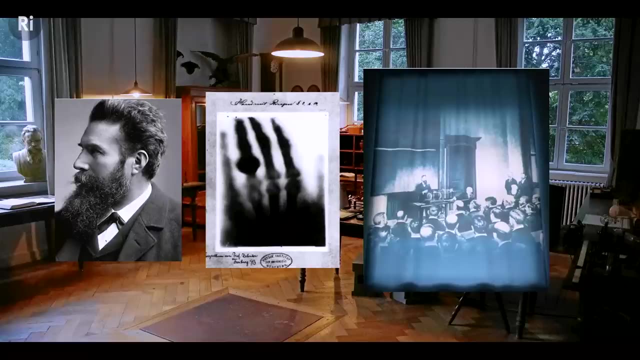 Now, very quickly, Roentgen told the local medical society about that And this is a photograph of him presenting his discovery to the local medical society in Würzburg- And he decided very quickly: instead of patenting his idea, he would sort of hand over this concept. 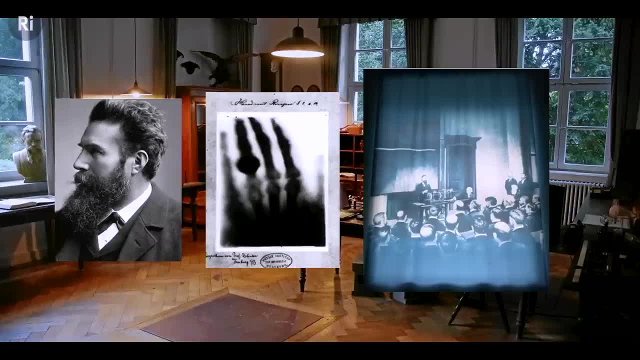 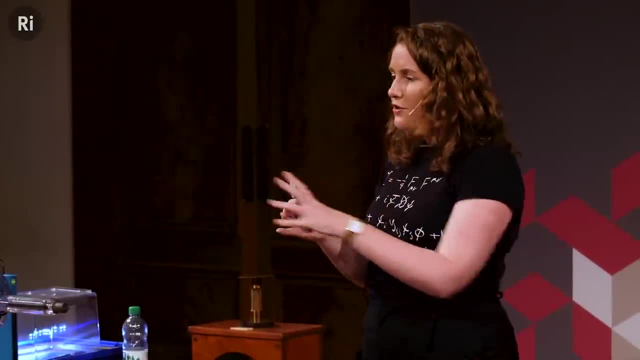 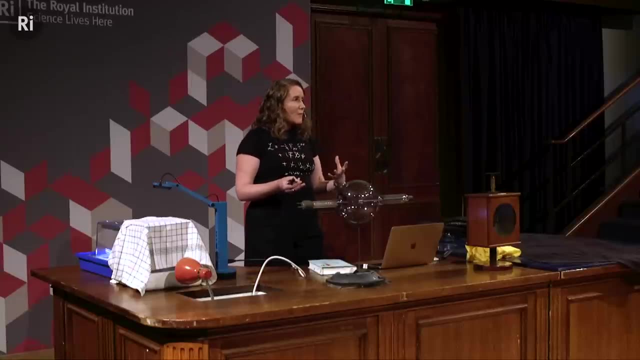 to the medical profession and let them develop the medical application of that. And very quickly we had the following year people using x-ray tubes like this one. This one actually does produce x-rays, by the way, On battlefields to remove shrapnel from soldiers' bodies, And we had it used, you know, almost. 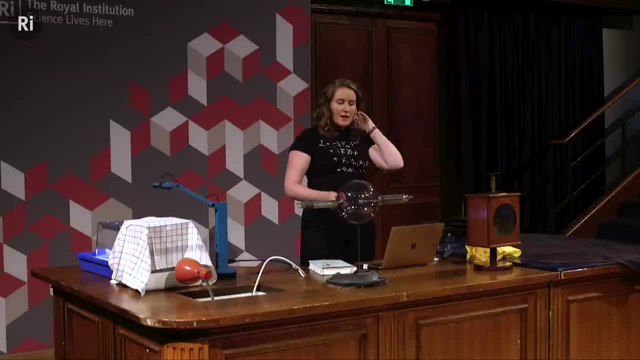 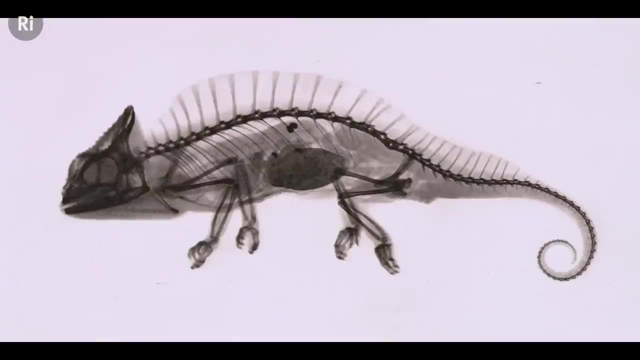 immediately because these things were so common in different labs around the world. It was so common, in fact, that even artists had it. This is a photograph taken two weeks after Roentgen's discovery by some photographers, And so very quickly we get not just an impact in the medical 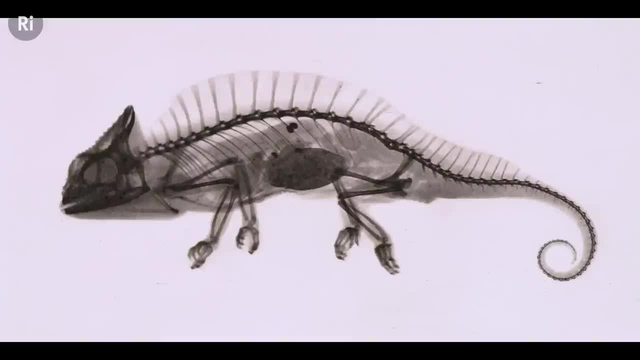 profession. but we also get even a whole new type of photography and of understanding of anatomy, which came from some of these x-ray images. And this is a photograph of him, And he was also beautiful photographs. This one's from Austria And this happened literally in two weeks, right. 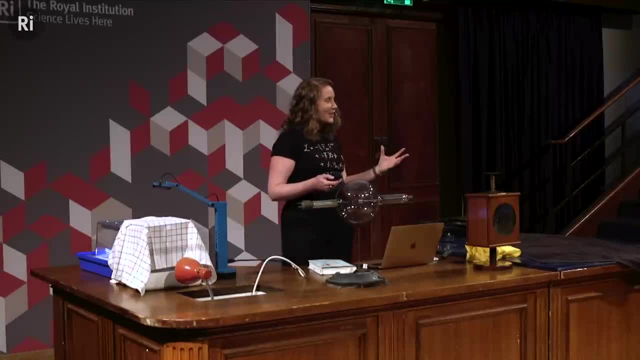 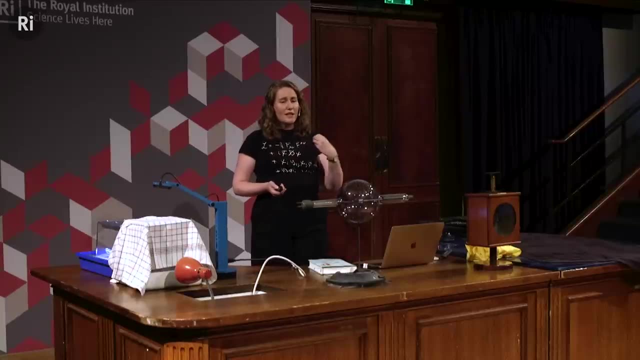 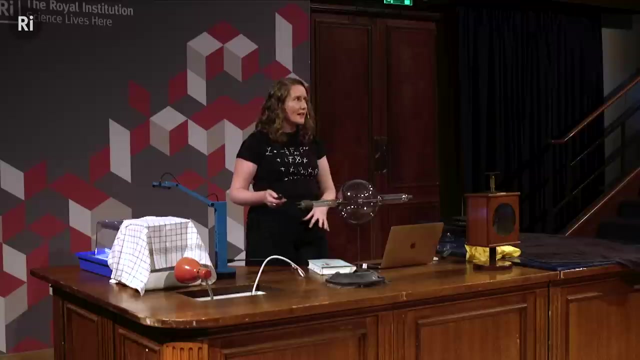 So once someone has the idea and communicates it, it's spread like wildfire. So X-rays still weren't very well understood at that point, but he could determine from his experiments that they didn't quite move around like normal light, but they kind of acted like a type of 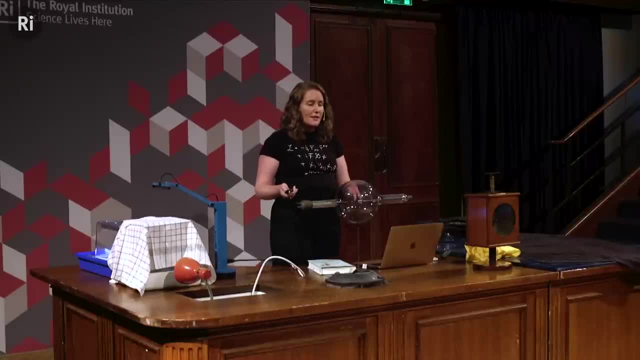 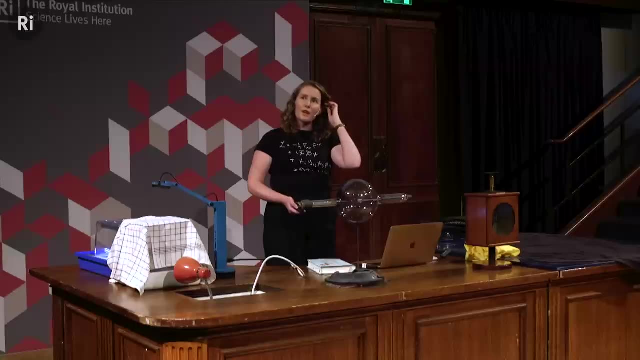 light, And now we know that they're a high energy form of light that can travel through objects. So what happened over time with that is an interesting story, because over many, many years, and now I'm talking decades, we get from the very first version of X-rays and some very 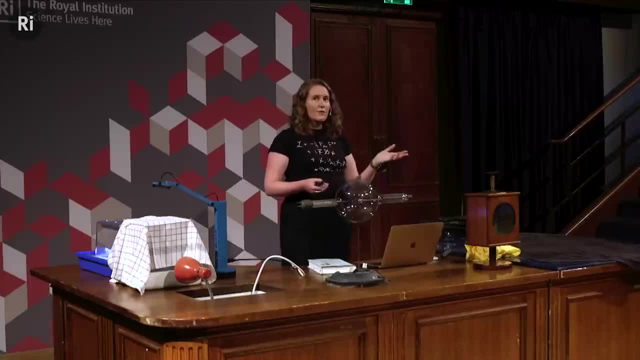 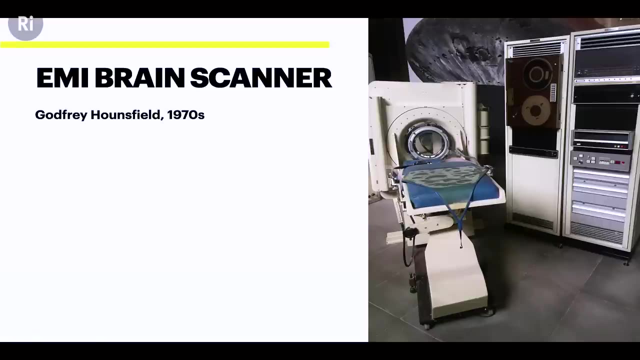 rough, you know, hand X-rays to what we now know and love and use as a first-line medical treatment technology in hospitals, which is the CT scanner, And that took the coalescing of X-rays and advanced, you know, X-ray tube technology. It took the advancement of computers. 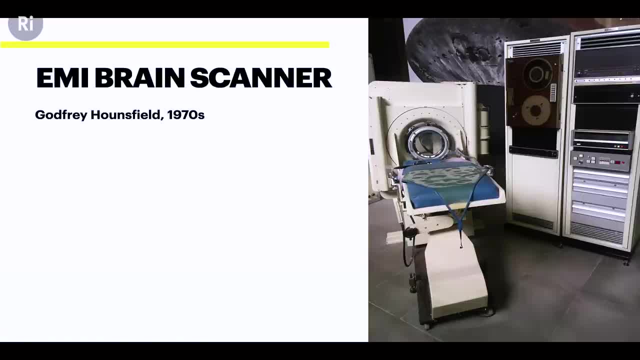 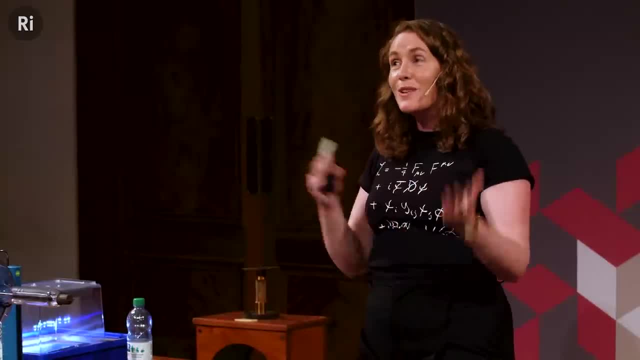 which we'll talk more about, And it took, you know, a bit of clever mathematics And someone working at EMI. that's a record label, if you've heard of it. that's why it was the Beatles record label. But they also created different technologies. And so this guy, Godfrey Hansfield, in the 1970s. 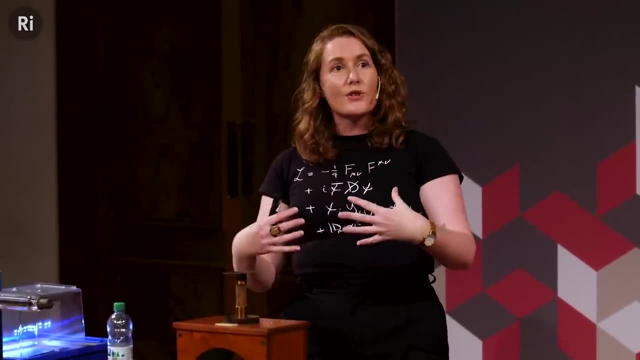 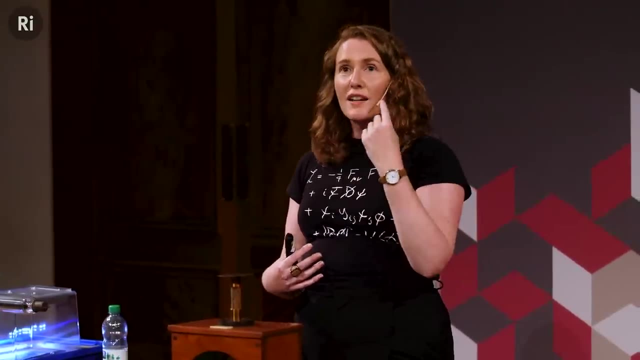 set about trying to combine these technologies together to take images inside the human body where you could actually see in three dimensions. And it was quite a journey. He had to actually test his device And he had to actually test his device, And he had to actually test his device And he had to actually 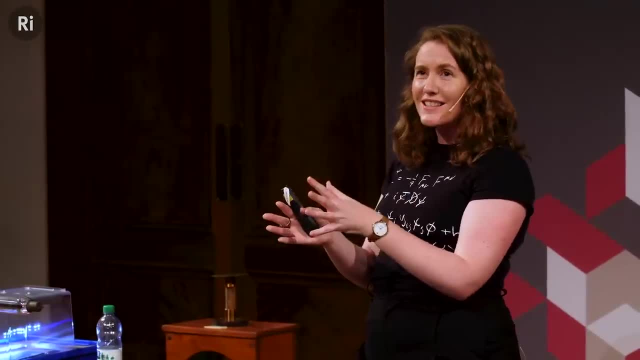 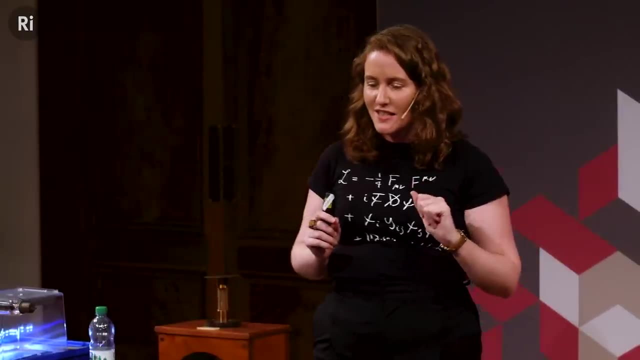 cut out the brains from cows in abattoirs and carry them across London in a paper bag to put them on his test machine, which- sorry if there's any vegans in the audience, But it was remarkably successful And it actually went far beyond what Roentgen thought was. 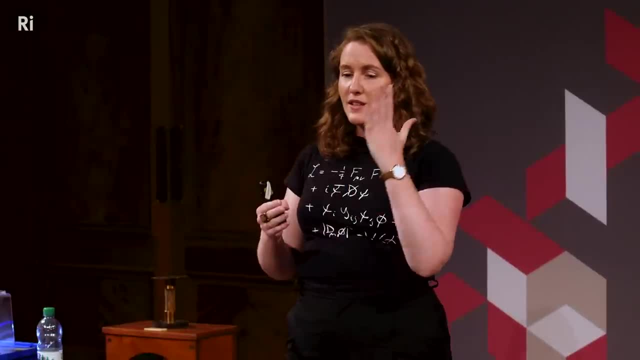 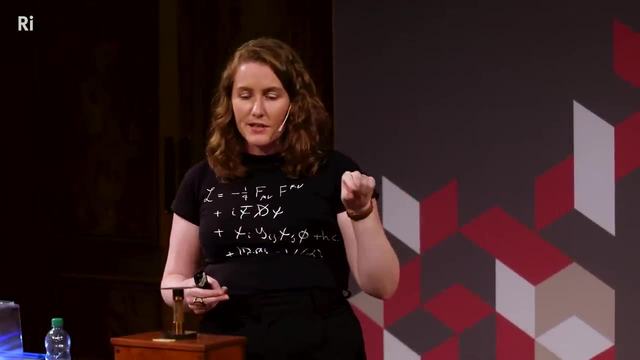 originally possible, Because originally you would think, if there was something in the way as you're making an image, that you'd never be able to get around that. But actually with the three-dimensional reconstruction of modern CT scanners we can see in detail. 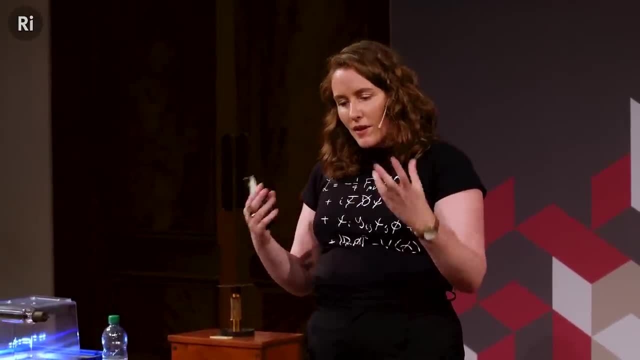 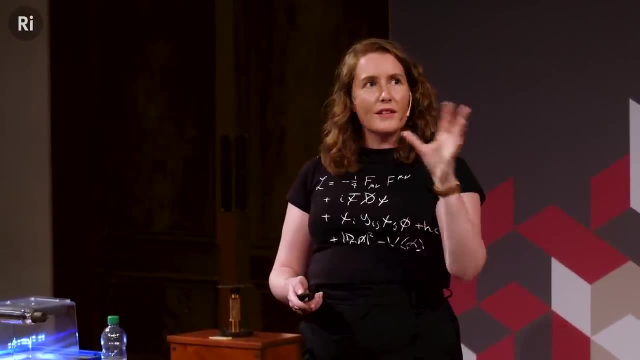 the soft tissues and different tissues and things, And so this is really used millions and millions of times a year now in hospitals all around the world. So a few things to point out about this is that the physicists themselves had no idea what this could be used for right. 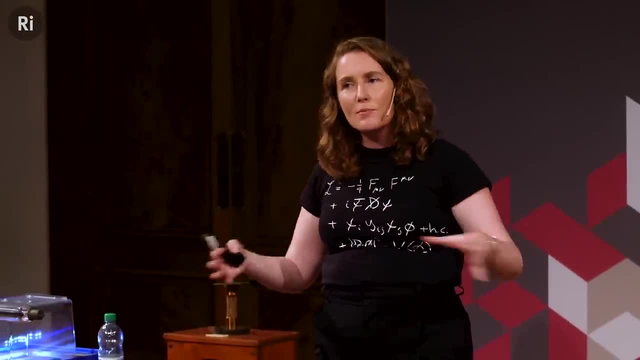 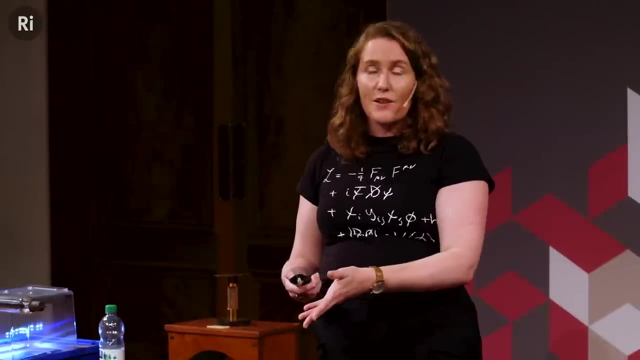 And then also, it took decades for the multiple different inventions and technologies to come together to realise what we would now call an innovation of a CT scanner or a medical technology, And this is important to keep in mind As we go through our story about the timescale involved. 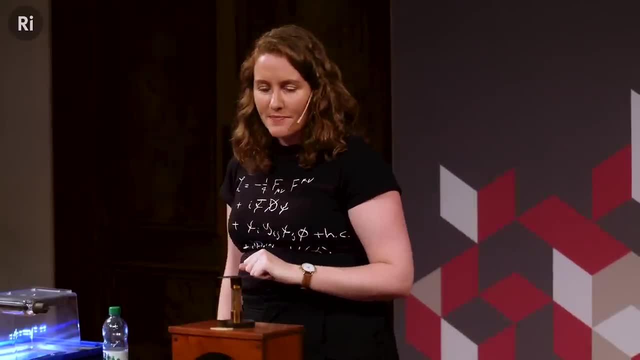 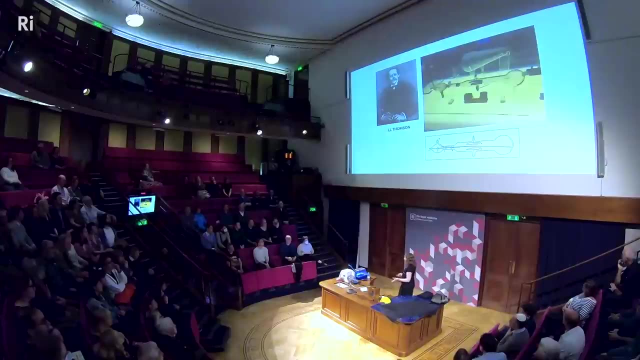 Now, my next story involves almost exactly the same type of apparatus, but it happened here in this theatre. In fact, the announcement of this discovery happened here in this theatre, And this is really where our story of particle physics begins, And it begins with this man, JJ Thompson, who was 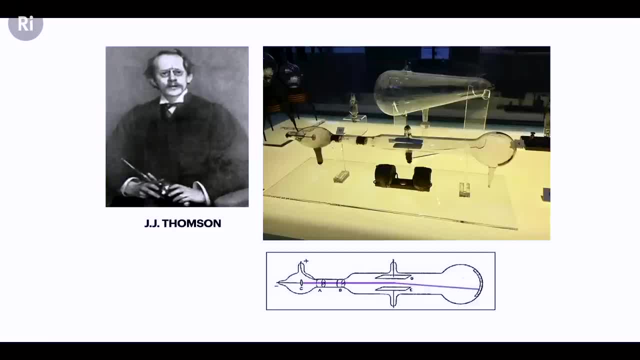 the director of the Cavendish Laboratory in Cambridge at the time And he wanted to explore after Röntgen had discovered X-rays. he wanted to explore what was happening inside the tube because it was making this glow, but still no one knew the nature of the cathode rays themselves. 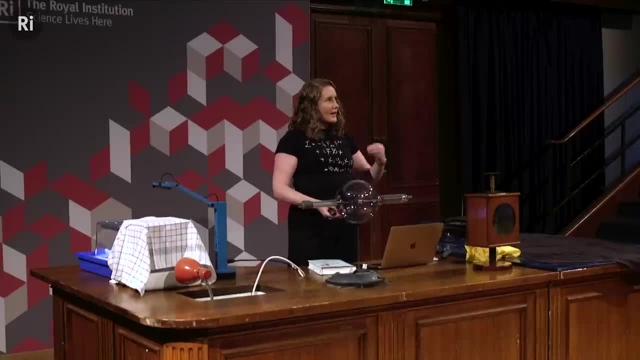 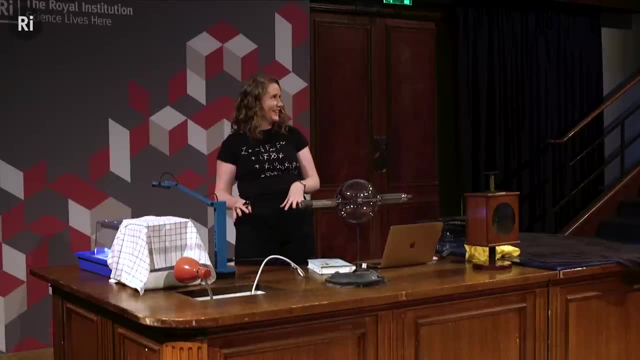 And so he designed an experiment, or I should say, he designed it and somebody else made it, because Thomson was famously completely useless with his hands. Röntgen was very good with his hands, right. Thomson not so much, And so he had to employ the services of a glassblower. 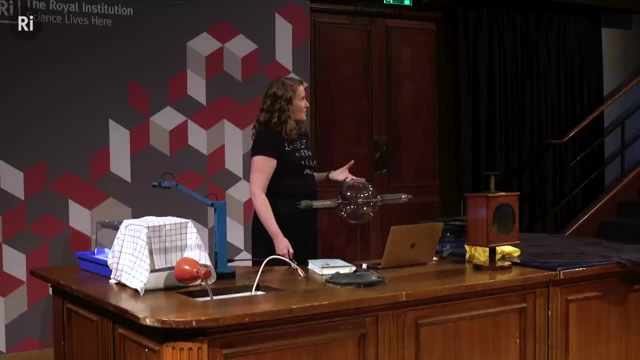 And one of the things that I learnt through writing this book was actually how skilled and detailed it was and how difficult it was to actually invent the apparatus that I'm talking about, to do the experiments, because you might get the impression that anyone with half a brain at that point in time- 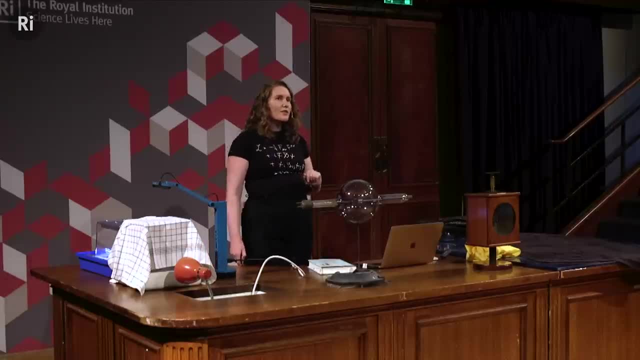 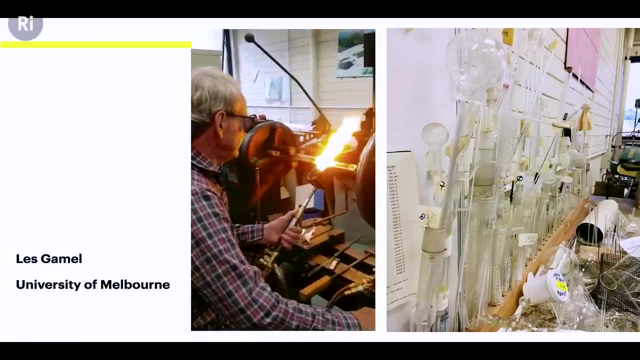 could make a world-leading discovery. So before I tell you what Thomson did, I want to show you this video. There we go. So this is Les Gamble. He's a scientific glassblower at the University of New York, The University of Melbourne in Australia. 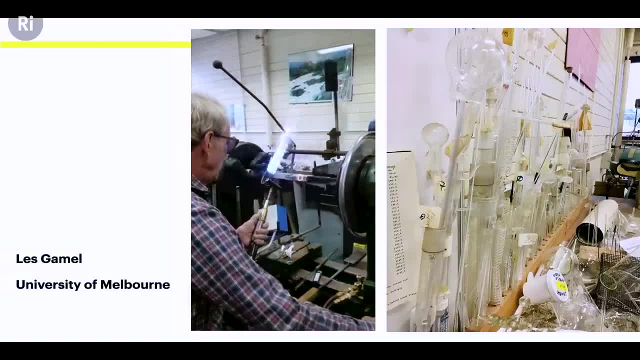 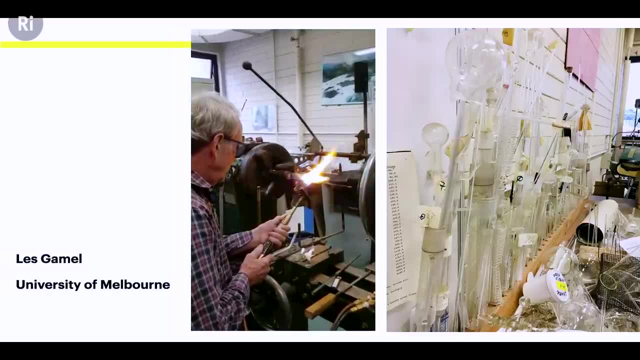 which is one of the institutes I work at. He's just retired, actually through the pandemic, so he no longer blows glass, But just pre-pandemic. I got in there and asked him to show me how it works, And so what he's doing there is he's using some gases. 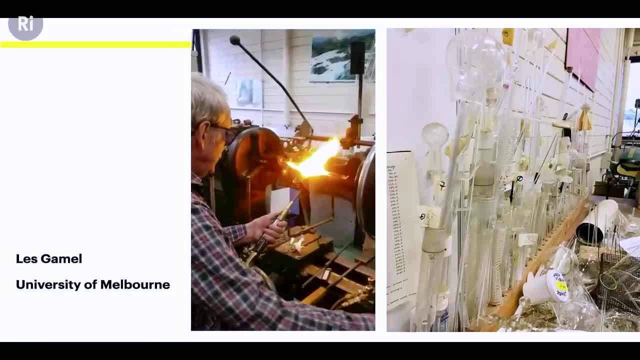 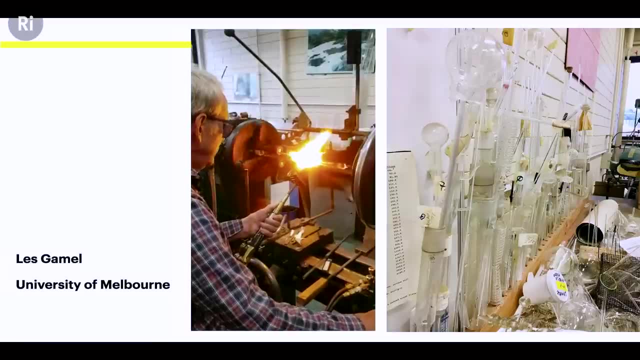 to create the flame, the torch, and he's heating a glass cylinder. You can see it glowing red. Let me pull this away. There we go. And now what you might not see so clearly is in the side of his mouth, away from the camera. 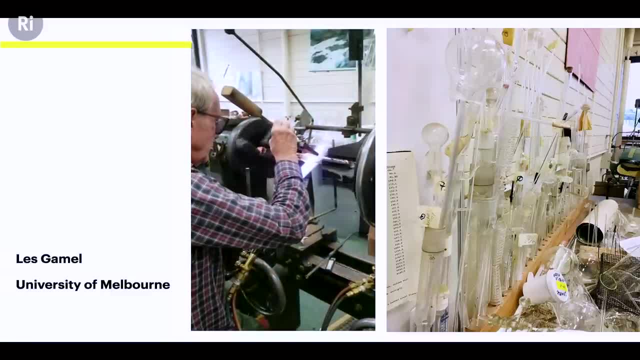 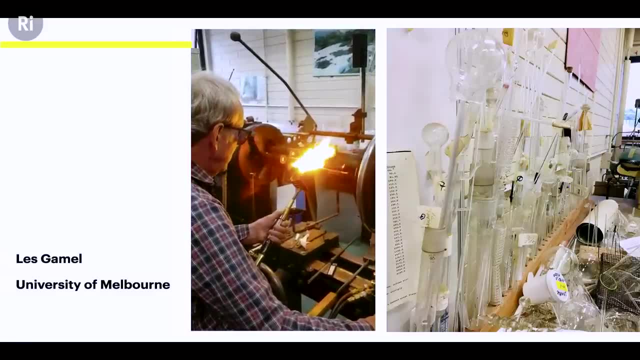 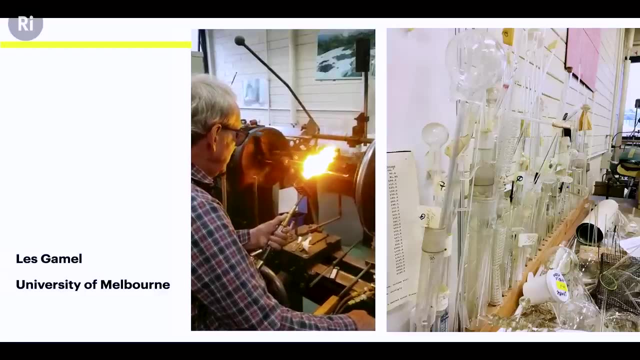 he has a pipe, So he's blowing into that pipe And you'll see him. there he goes. he's blowing in and coaxing it with a metal iron to create a bulb, or a bubble in the middle of the glass tube. I'll give him a minute. 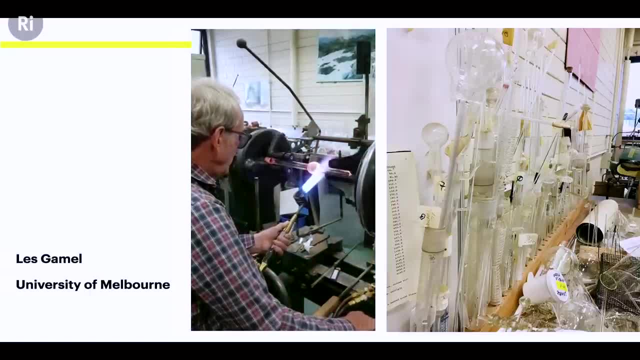 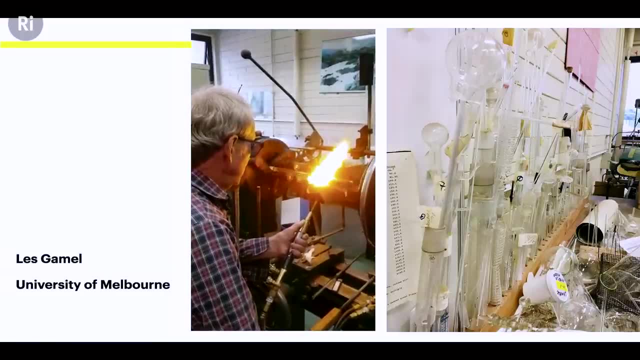 So this sound you're hearing, this whooshing sound, would have been there we go. he's created a glass bubble, So this would have been a sound that you heard all the time in science labs back in the day, which was something that I sort of discovered. 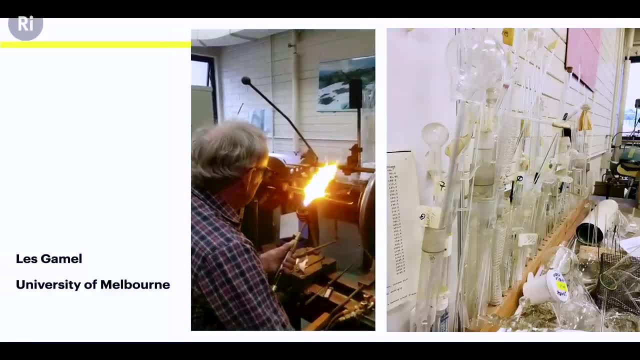 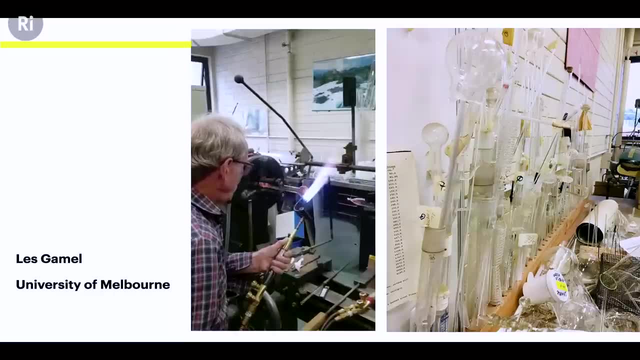 through this process, And in a moment when he's ready, there we go. you can see he's pulled the side away and he's separated the two ends of the tube, And so what he's left with there, there we go, is a glass bulb. 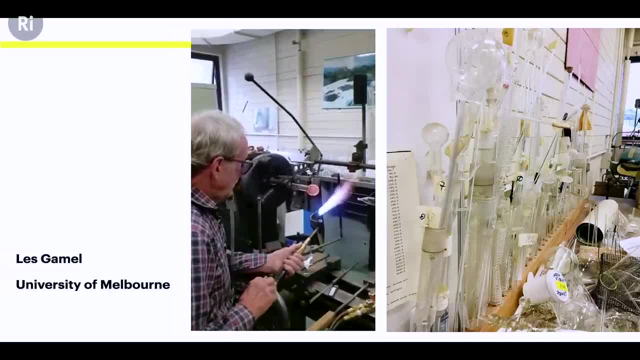 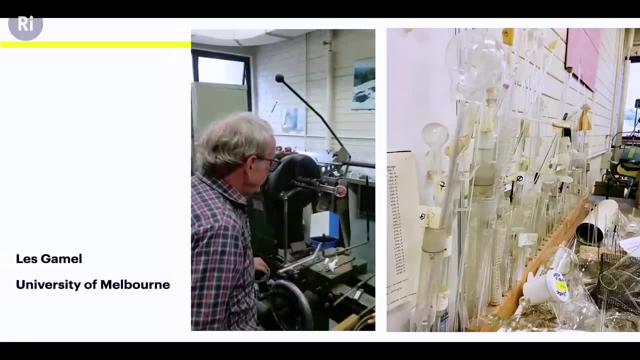 Now this one he did just as a practice to show me how he actually did it. And it's quite astonishing and it cools down so quickly. You can see, look the colour's gone already. There we go. so he did that one to show me. 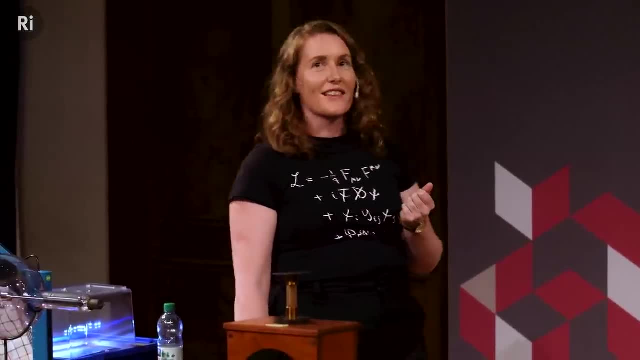 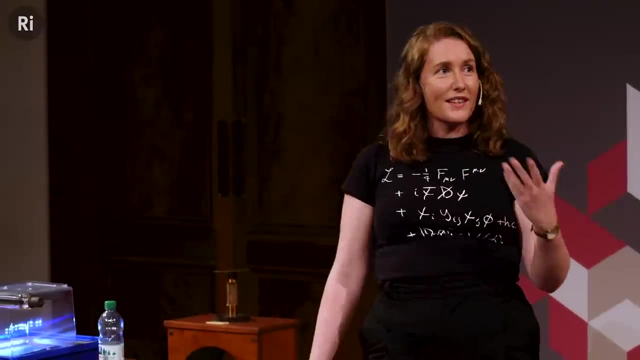 Some of the other things that he's created are on the right-hand side of the picture. there This is his lab, which I love because it's just like it's a real working lab. It's full of glass. So just to make the point that we think. 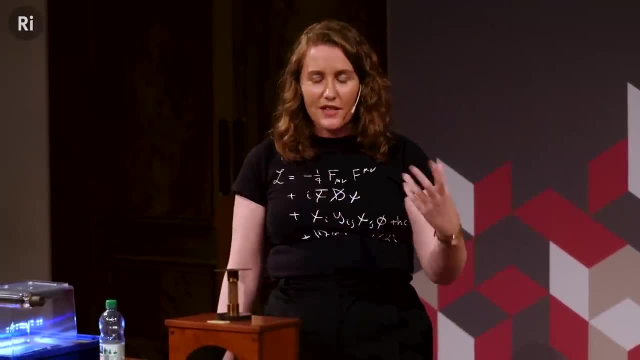 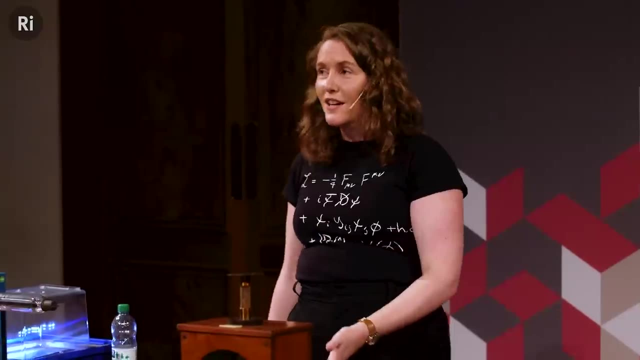 that nowadays we do this like very detailed, very complex engineering work, but actually back in the day it was much more artisanal, And if I was a physicist then I would have had to learn how to do this myself, Breaking glass again and again in order. 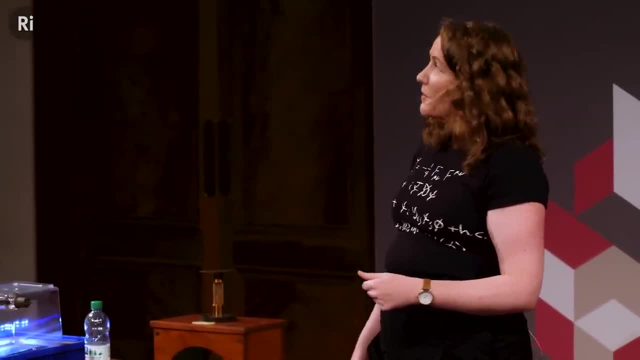 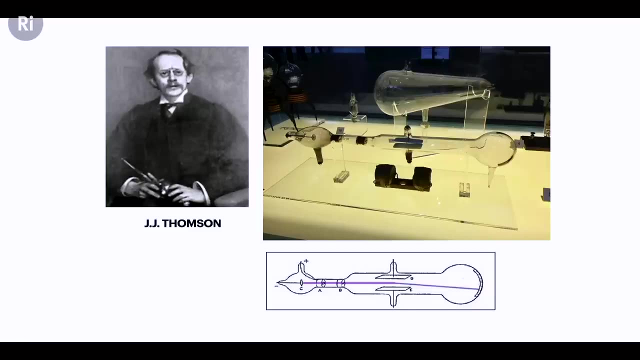 to create the apparatus that was needed. So let me come back to JJ Thompson for a minute. So there was two things that Thompson wanted to ask about these cathode rays, And he had a theory that these cathode rays were a type of particle. 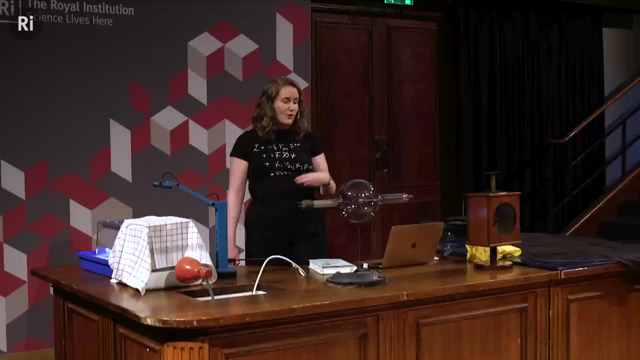 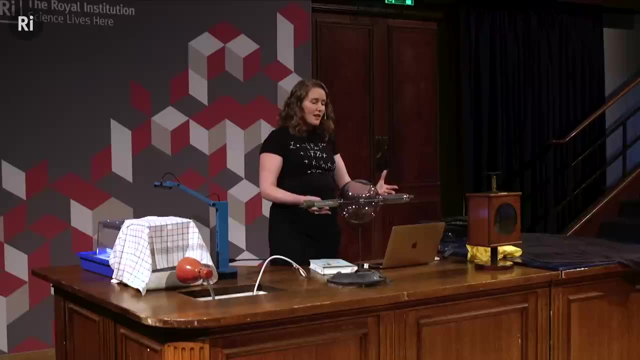 Now, this was not held by his contemporaries in Germany. In Germany, they thought that this tube was glowing because there was a form of light in there, But he thought that it might be a type of particle, And if it was, then he should be able to measure two things. 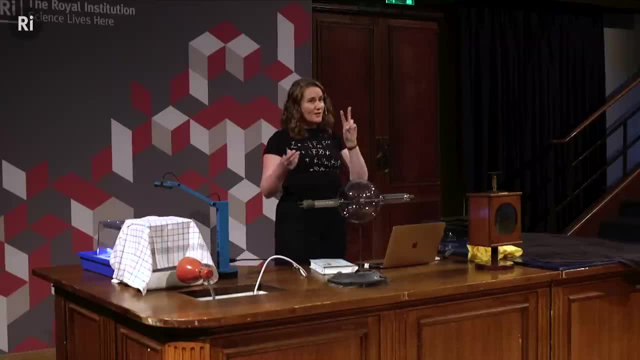 One was the charge and the other one was the mass, And in fact what he really wanted was the ratio of those two things, the charge to mass ratio. So he used a tube like this, but it's the one shown in the picture here. 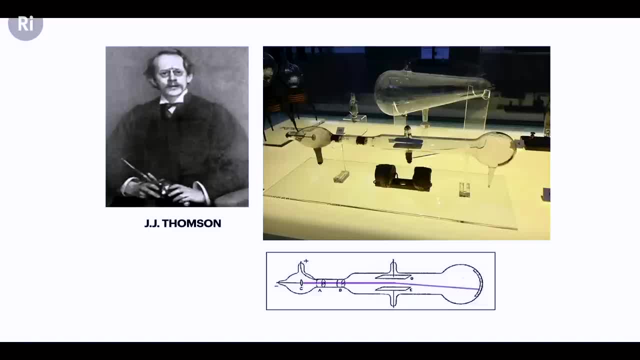 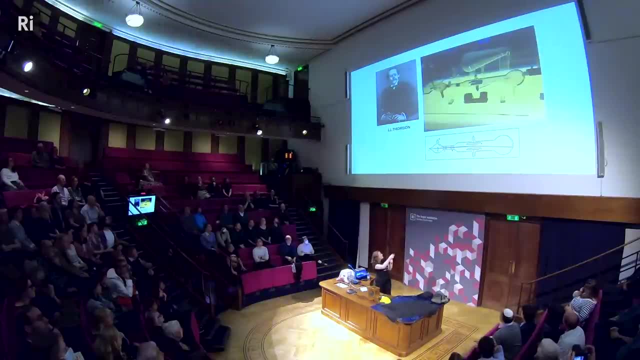 And this is actually in the. I've got a laser pointer. This one is actually in the Science Museum in London if you'd like to go and see the original. That's my photograph of it, And inside here he was able to apply magnetic fields. 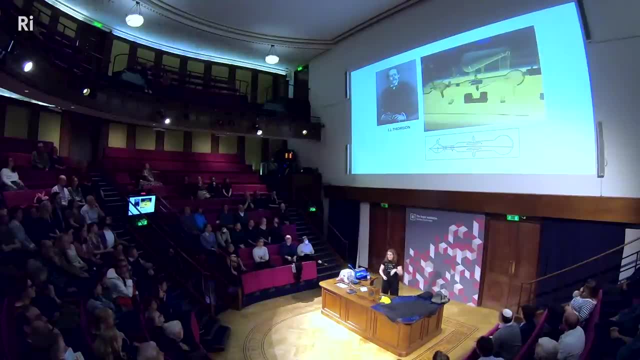 and electric fields in order to bend the beam around And to measure, firstly, the charge. he would put it onto a device like this one- This is called an electroscope- And let me just actually let me show you how this works. 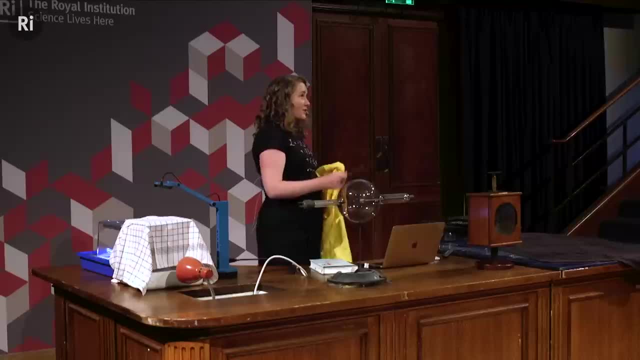 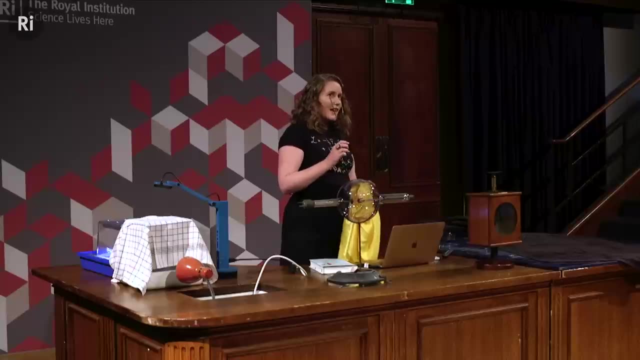 because this will become important in a moment. So this is actually an original electroscope from the Royal Institution collection. I think it was owned by James Dewar And apparently they've never before used a collection item to actually show a demonstration in this theatre. 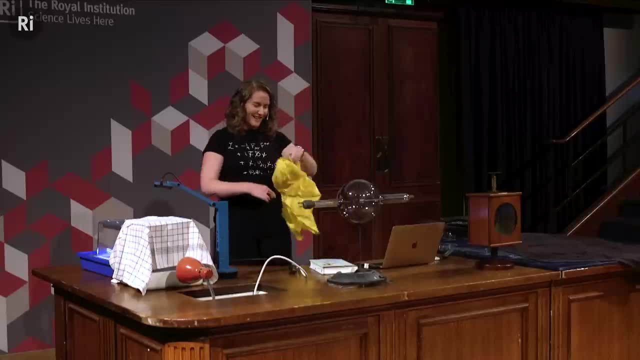 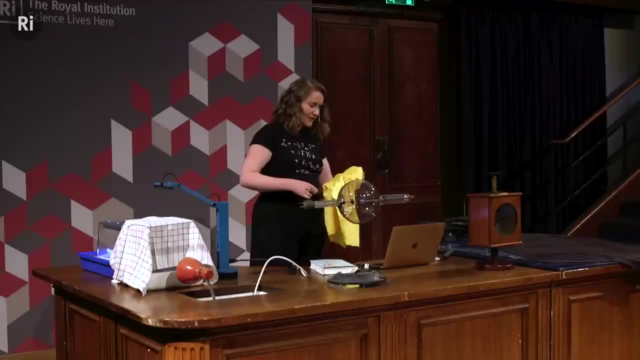 So I have the great honour of being the first person to actually try and use a heritage object to do a demo here. So let me, if I can, get this sorted out. So I've got just a Perspex rod here and this cloth. 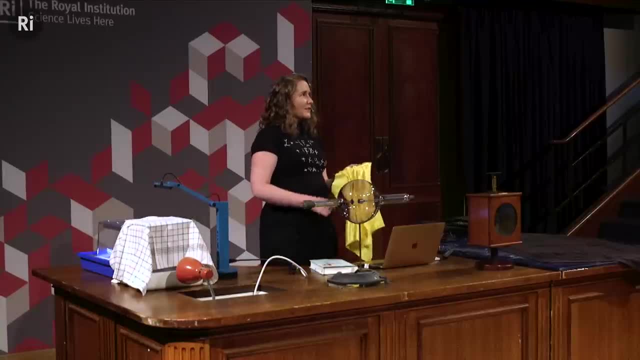 which hopefully will charge the Perspex rod up. So this is called an electroscope, this device, And it just it has sort of this metal plate. on the top There's a metal rod coming down, And hanging off the metal rod is two thin leaves of foil. 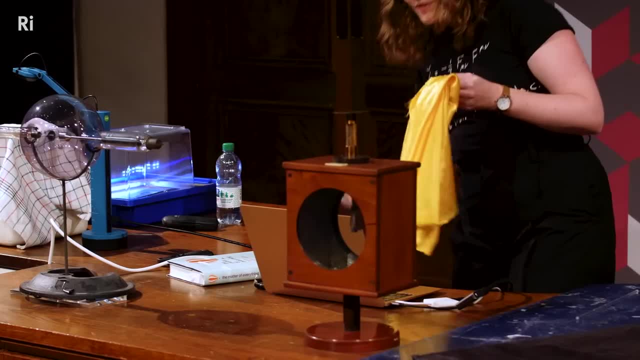 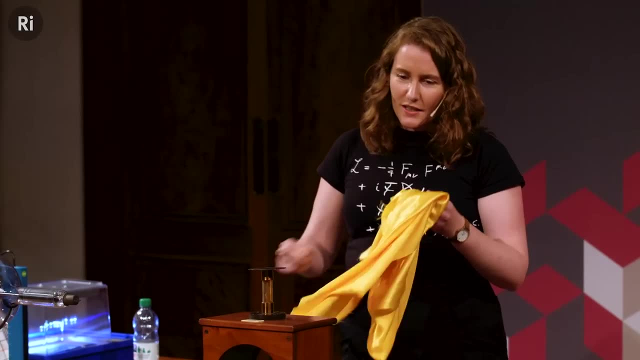 And they would usually be big gold, or this one looks silver in colour, So it might be, I don't know, some other thin, highly ductile metal, And when you charge up the electroscope, there we go. I'll just leave that placed on there. 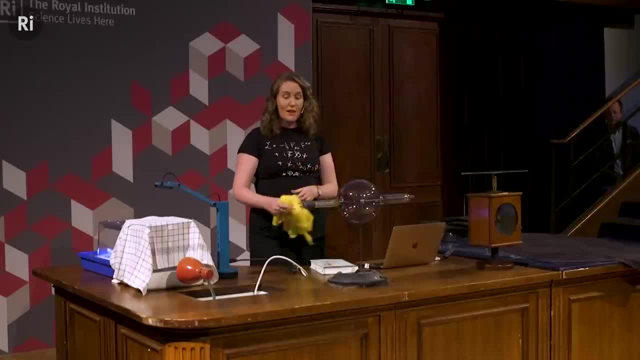 Hopefully you observed that The people in the front hopefully can see what happened with this. the leaves did this, Yeah, yeah, they splayed apart And so by measuring so you could charge up one of these And when you put a. 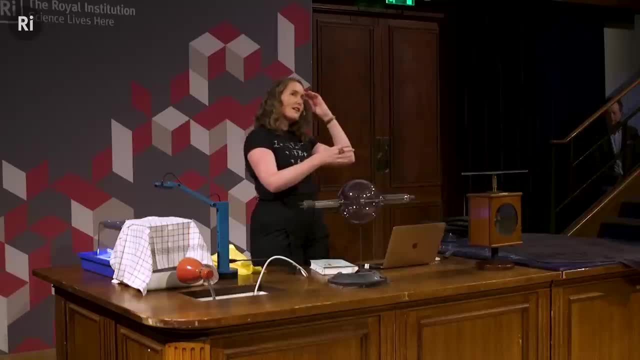 something that was charged onto the plate. in a version of this, over time the leaves would fall back down toward each other And if you sort of measured how long that took, you could measure the charge that was being deposited onto the electroscope. 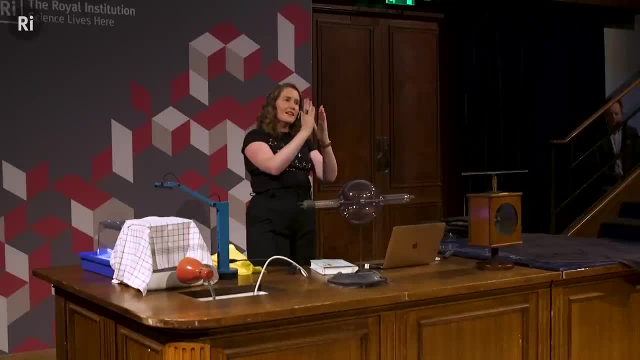 And eventually they put sort of meters on them so that you could call it an electrometer right to actually measure it over time. So I'm very glad that that works from the collections. Thank you, Charlotte, who's our collection manager? 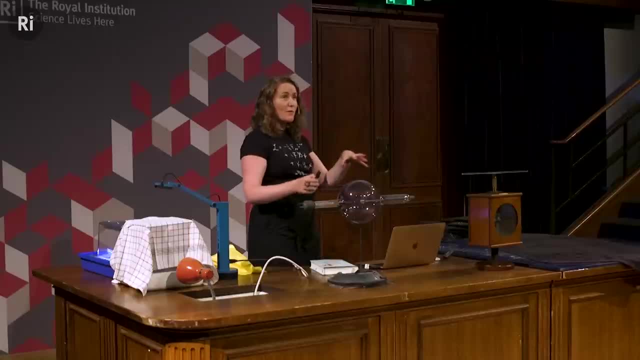 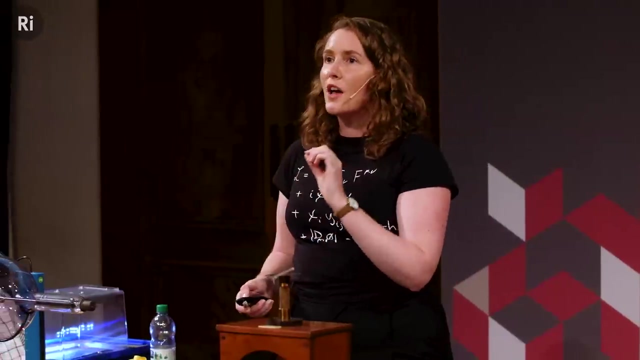 for bringing it up. So this is the kind of equipment that JJ Thompson was working with. Now, what he found was that these cathode rays had a normal electric charge, a negative electric charge, but they were 2,000 times lighter than the hydrogen atom. 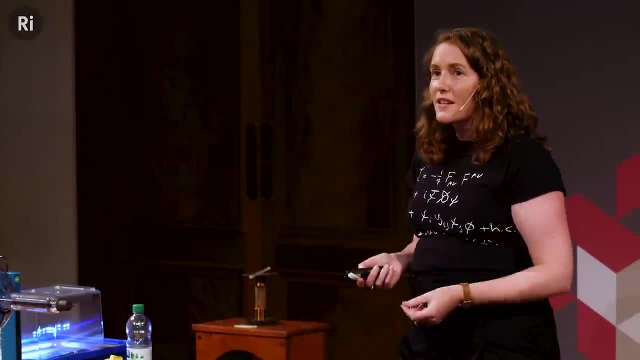 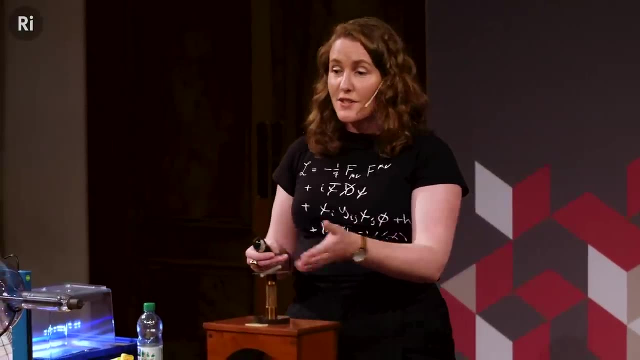 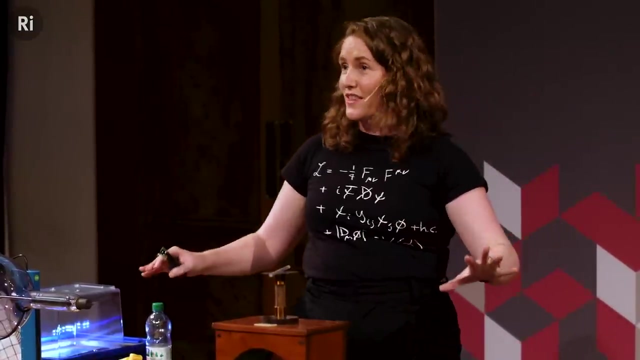 which was the lightest thing they knew at that time. What he discovered was the electron, as we now call it, And Thompson announced and did this series of experiments showing the charge and the mass and the different bending with the electric and magnetic Magnetic fields in this very theater. 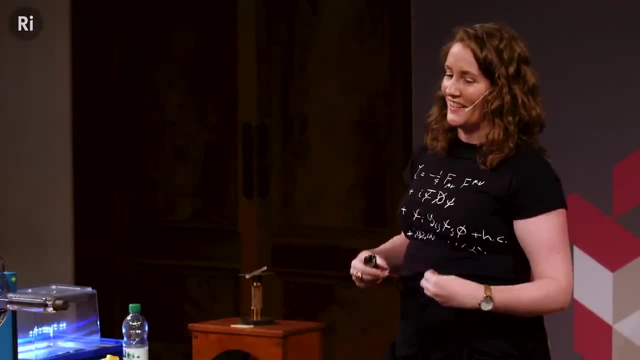 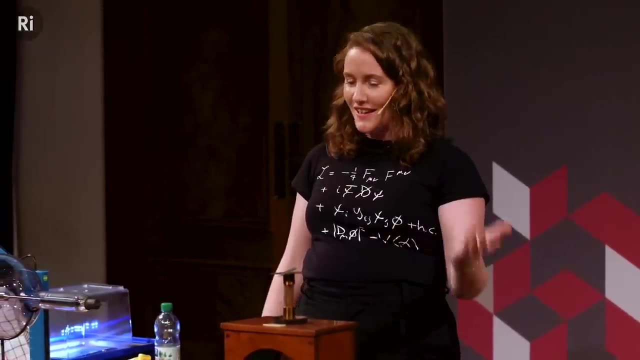 perhaps at this very desk that I'm standing at. So it is quite an honor to stand here and explain his experiments- poorly, I'm sure. Unfortunately I don't have his exact device to show you the exact experiments, But it's quite an astonishing thing that, with 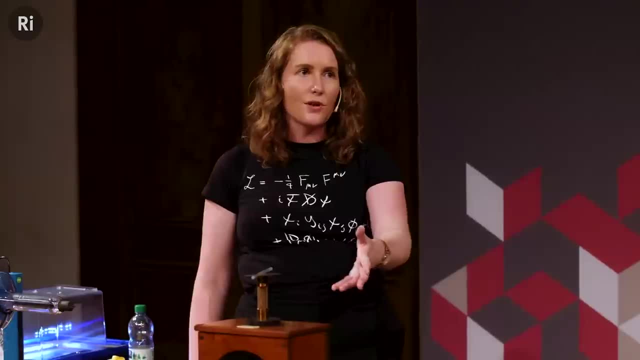 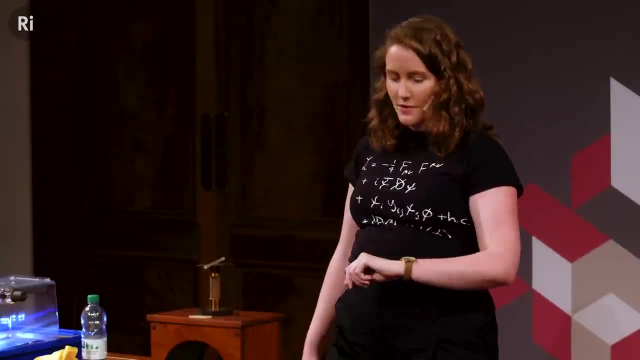 such a simple apparatus made from glass and a simple electroscope made from sort of a wooden box and some bits of metal that you could discover the first subatomic particle, the first particle smaller than the atom Right Now. Thompson didn't think this would go anywhere. 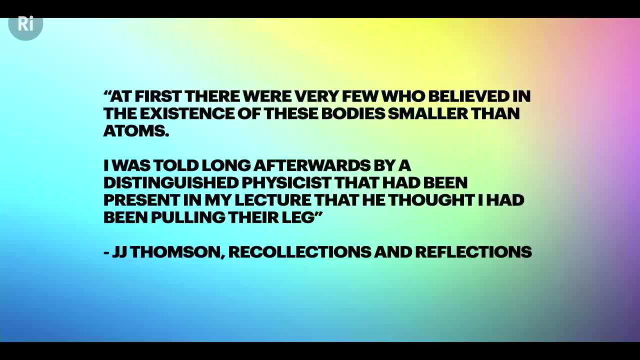 And in fact it wasn't very well received- the idea that there were particles smaller than atoms, He said. at first there were very few who believed in the existence of these bodies smaller than atoms, And I was told long afterwards by a distinguished physicist that had been present in my lecture. 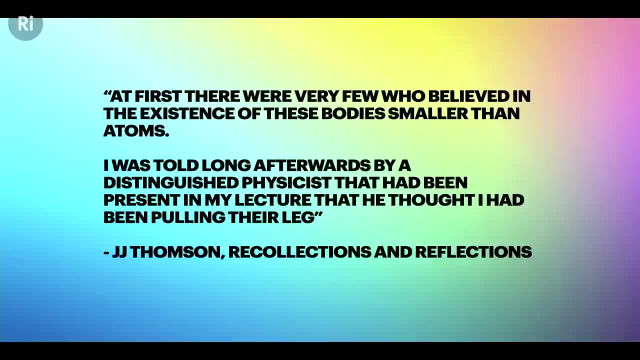 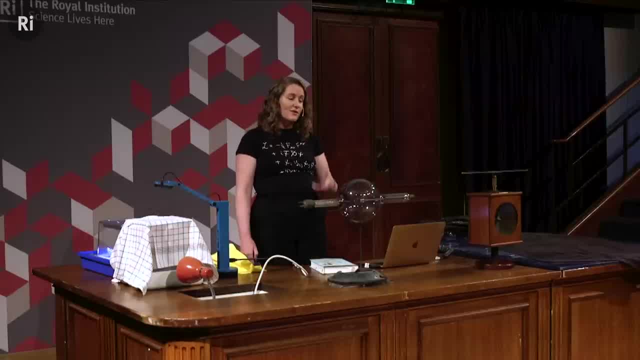 that he thought I'd been pulling their leg. Now, in fact, 20 years later, he came back to the Royal Institution and gave another lecture about the industrial applications of these electrons, Because it turns out that they were incredibly important. So, first of all, he understood that in these tubes 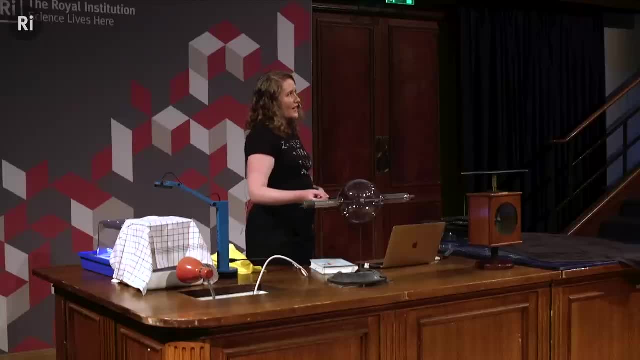 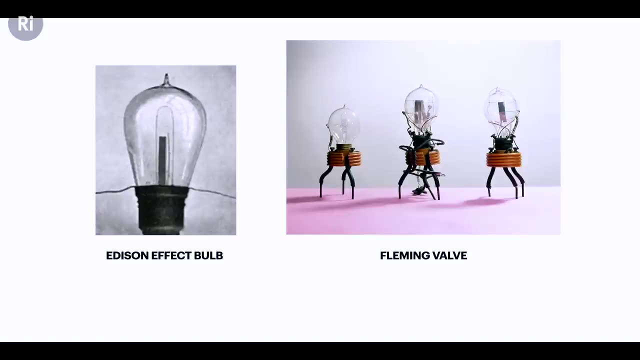 the electrons were being created by the filament or the cathode at one end. And when he studied light bulbs that say Thomas Edison was creating for lighting households, he found the same thing: that light bulbs also generated electrons through a process called thermionic emission. 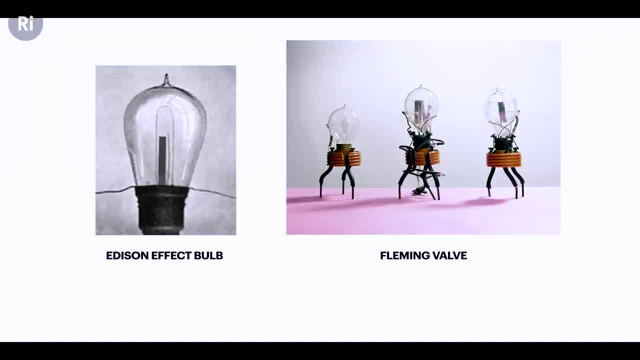 And this all came together with a person called Alexander Fleming a few years later, When he took an invention of Edison's that Edison had set aside, where Edison noticed that if you put multiple electrodes in a light bulb you can control the flow of current that comes out of it. 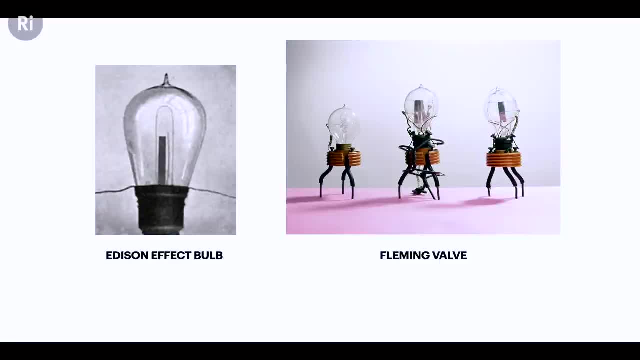 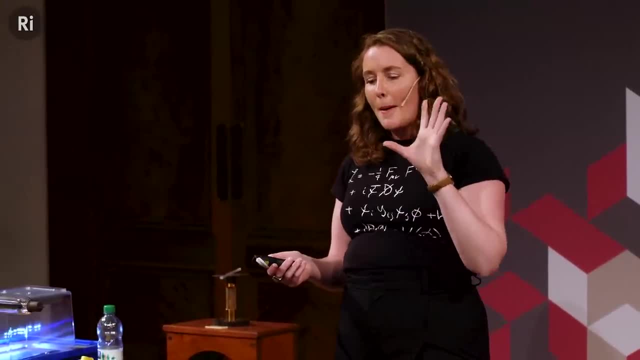 Now Edison couldn't see a use. He set it aside. He didn't understand it, He didn't try to understand it. In fact he was quite scathing about the kinds of scientists like Thomson who wanted to understand such things. But Fleming managed to bring together Thomson's work. 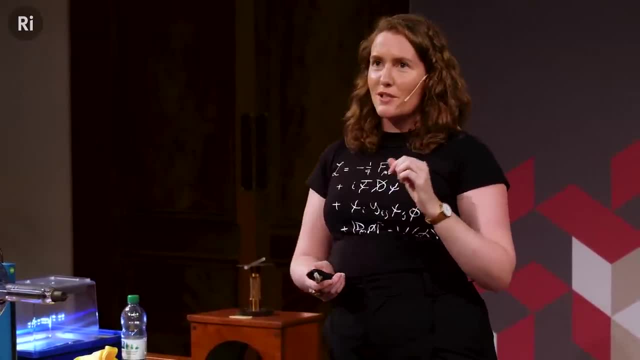 and Edison's work and created these devices which look kind of like miniature robots. So he was able to create these devices which look kind of like miniature robots and he was able to create these devices which look kind of like miniature robots. 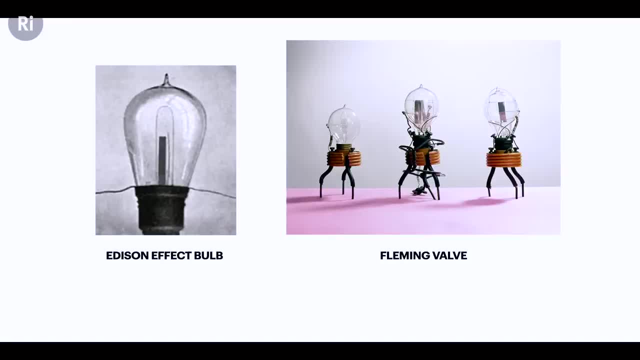 and he was able to create these devices which look kind of like miniature robots, which are called Fleming valves. Now, the important thing about a Fleming valve is that it is the very first electronic device And Fleming realised that this could be sensitive to a radio signal coming in. 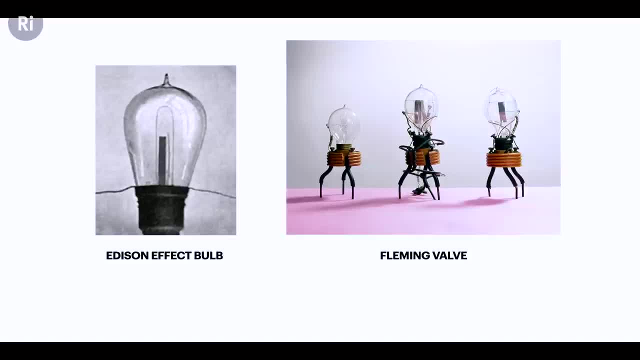 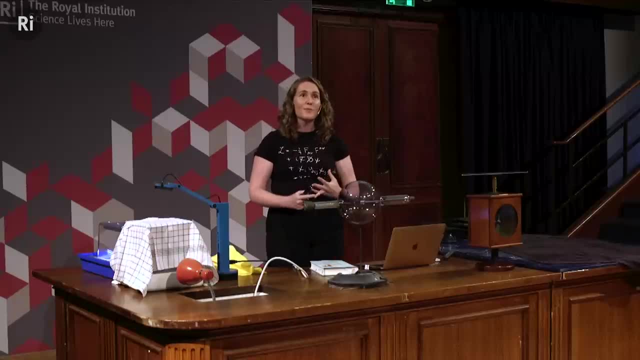 And if you put a radio signal in it can switch on and off an electrical current. This might not sound like much, but it is underpinning the entire radio telecommunications in early computer industries. So electronics as opposed to electrical devices, which we had previously. electrical devices work. 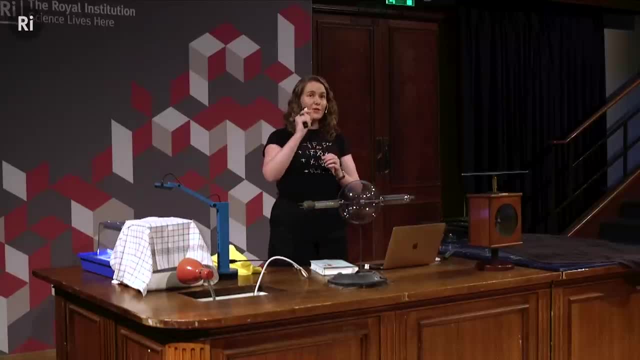 with currents and wires, but electronics now works with electrons moving through vacuum or through the air. And so this invention, which came off the back of Thomson's understanding, completely revolutionised our world. completely right, We would have no computers, we would have no radar radio. 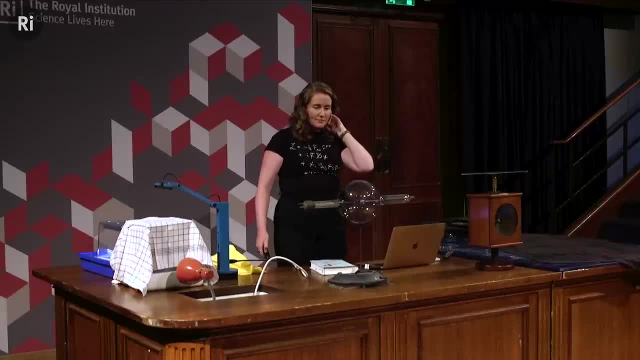 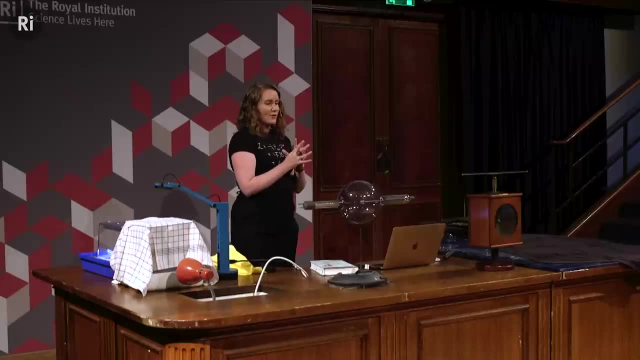 long distance telecommunications, any of that without this invention? Okay. So let's move on from that. So one of the other things I learnt as I went through this story, and I'll talk about this a little bit as we go through. 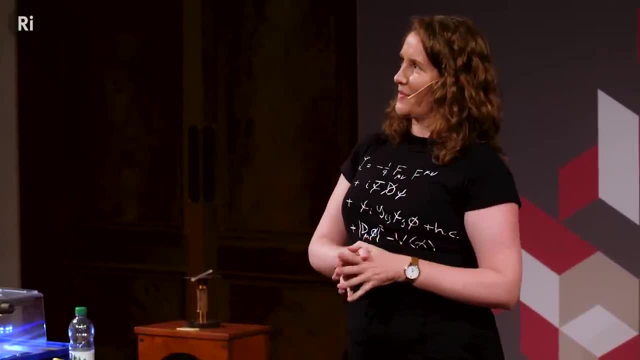 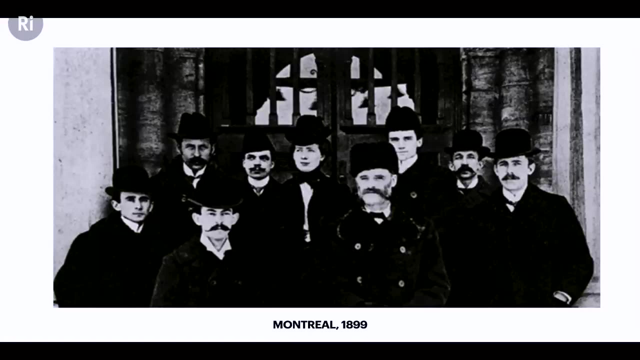 was that there were more people involved in these experiments than I thought at first, And this is a photograph of Ernest Rutherford's research group, his first research group in Montreal Now. Ernest Rutherford was a student of JJ Thomson. He was a New Zealander. 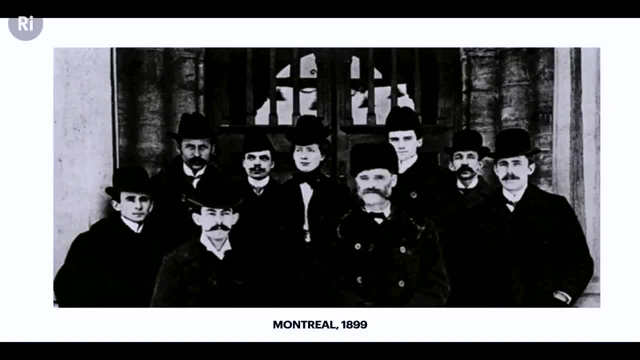 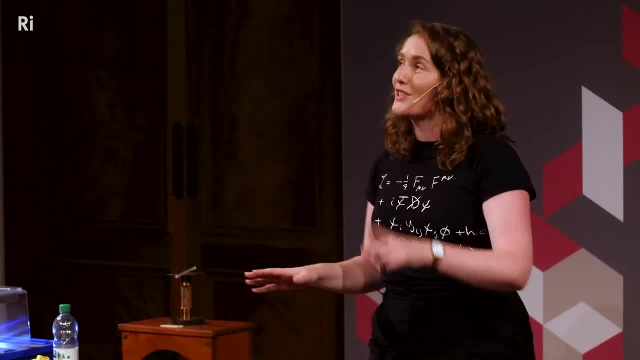 He was massively tall, massively boisterous, full of energy and used to speak so loudly that he would disrupt the electrical apparatus in his laboratories. Some of the students eventually built a light-up sign about this big above their table of experiments. that said: 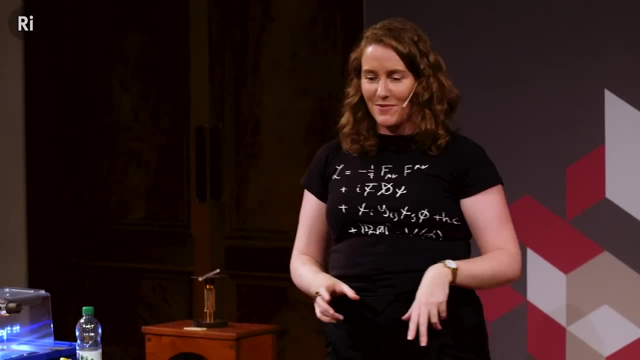 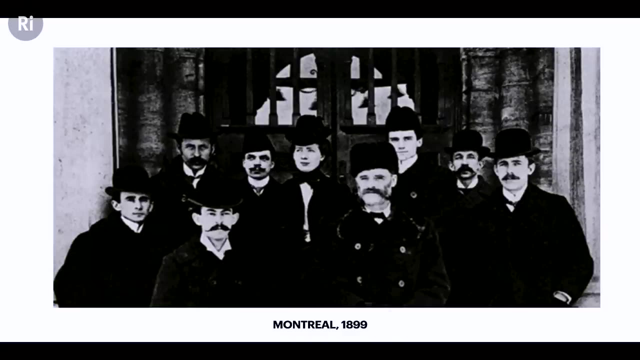 talk quietly, please, like this elaborate sign. And he would still walk in and like, hang his wet coat on something and electrocute himself. So Rutherford was a bit of a character, but he loved building simple kinds of experiments, as do I actually. 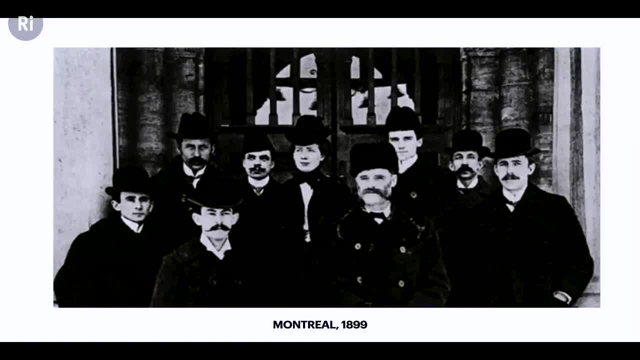 Now you'll notice someone in this picture who you might not recognise right, And this is the first person in this research journey that I went on who really jumped out at me, And I don't think it takes much for me to point out who she is. 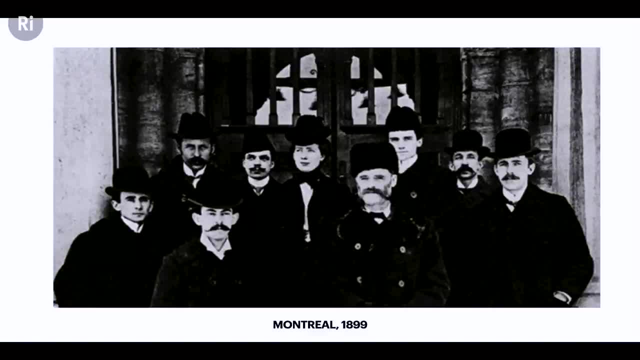 This is Harriet Brooks. She was Rutherford's first research student at Montreal And she, together with Rutherford and Frederick Soddy, a chemist, did some foundational experiments in understanding radioactivity. Now, during her time at Montreal, she was proposed to 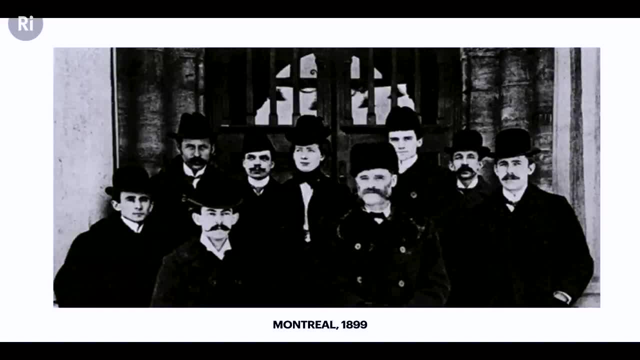 And she was told at that point that if she was going to become married, she would have to quit her job because she was to support herself. she was teaching physics at one of the women's colleges there, And so of course she protested and other people protested. 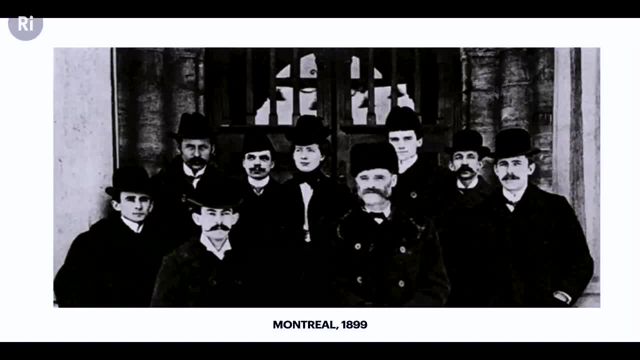 on her behalf- not, of course. actually that wasn't taken for granted. But she protested and it didn't work, So she broke off the engagement. This is how committed this woman was to doing physics. Now she was one of seven children. 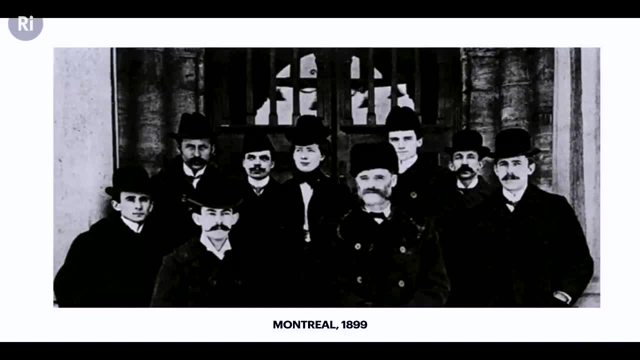 And she could not be supported by her family, which was unusual actually in the history of women in physics that she was not supported, That she wasn't actually from a particularly rich family. She had to support herself and had been doing. 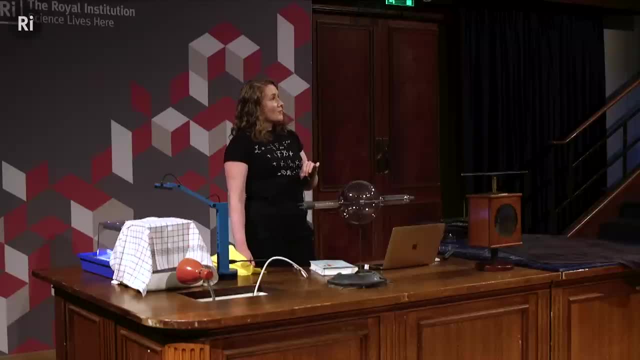 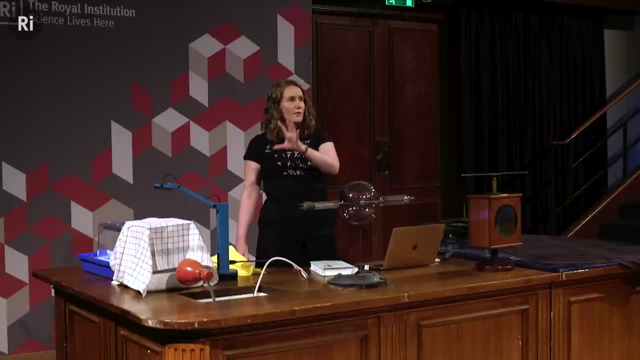 so through scholarships, because she was a very, very good student. So what happened later in her career is after making some amazing discoveries, and she went to the UK and she worked with Thompson, who kind of ignored her because he was busy with other things. 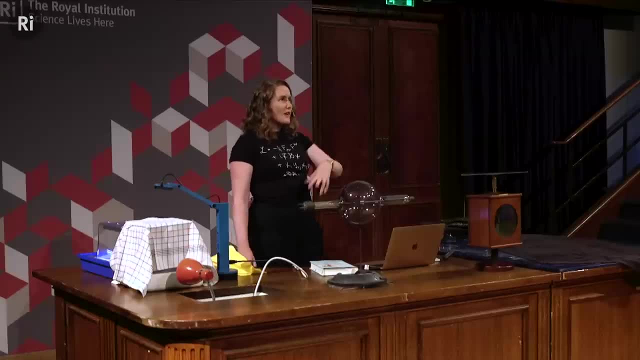 But she sort of moved back and forth Canada back to the UK, worked with Marie Curie for a while And then, at the grand old age of 31,, was approached again for marriage by a different man who she'd known when she was in Canada. 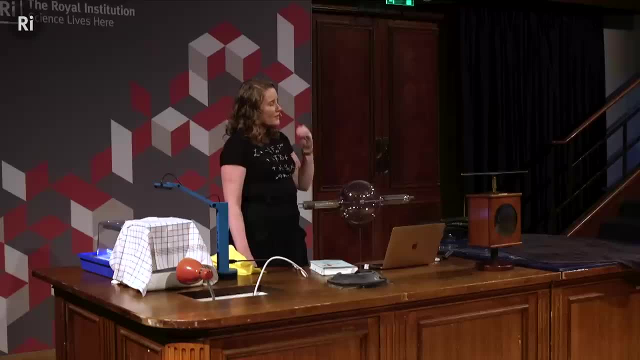 And at that point she actually the societal pressure was so strong that she actually got engaged, Had a couple of children And had to quit her work And never worked in physics again, which is probably why we've never heard of her. 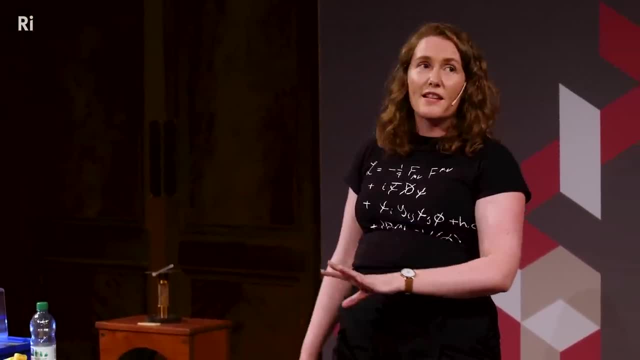 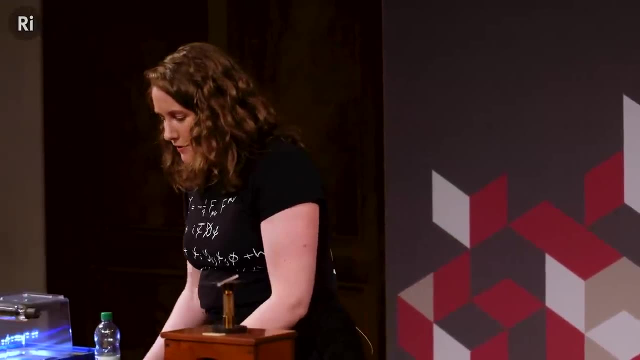 But in Canada she's now quite well known because in around the 1980s people realised the contributions that she had made, And I want to read a little bit about this. I think she's one of the biggest characterists. She's, in fact, the first woman in the British Empire to be close to her. 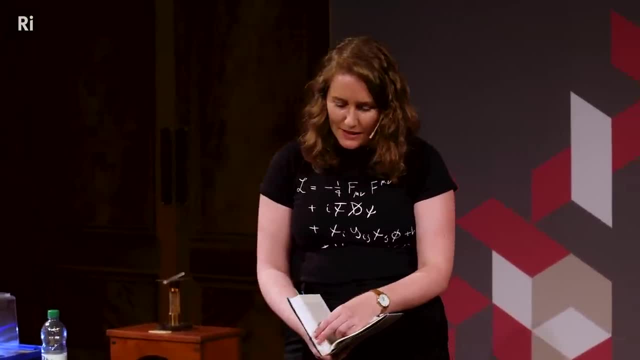 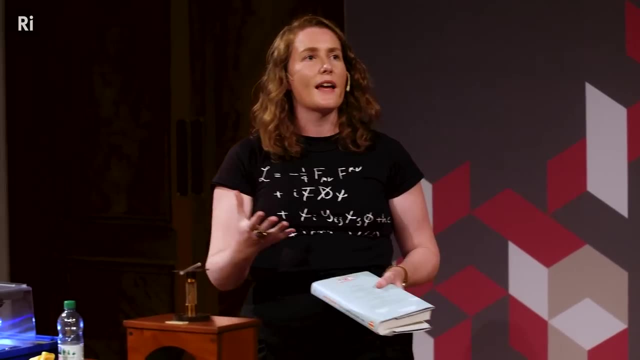 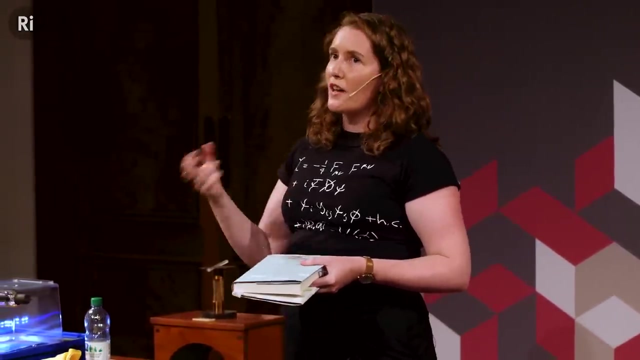 little bit from the book around radioactivity and its importance, because this work that Rutherford did in Montreal helped us understand that radioactive elements have a half-life. That means over time everything is changing. Elements are transmuting from one type to another over time. 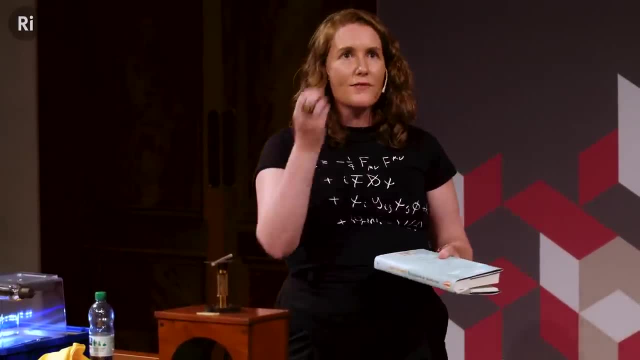 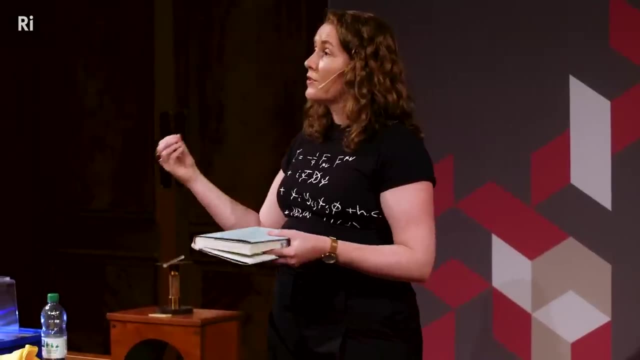 so nothing in nature is static, Even the elements we call, even the elements that we say are stable. well, that just means that their measured lifetime is longer than the age of the universe as we know it, But they are still. eventually, everything is going to change, and this is quite a large mental. 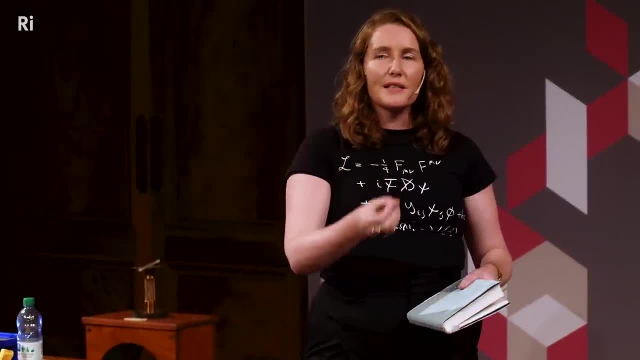 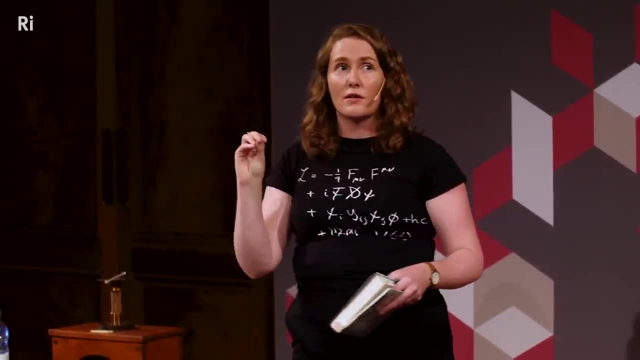 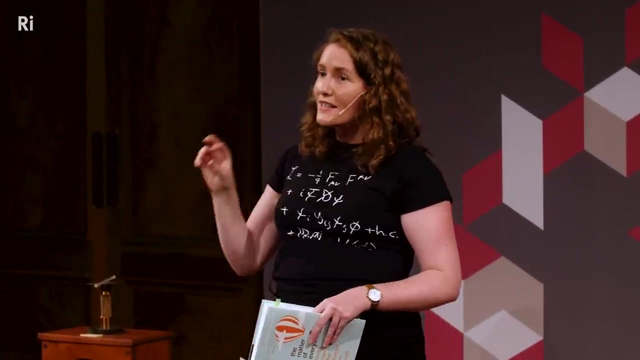 shift, But it also created the ability for us to understand the world in a way we'd never understood before, because if things change over time, that gives you a clock right, And so what Rutherford realised quite early on was that this could be used to understand the age of the earth. 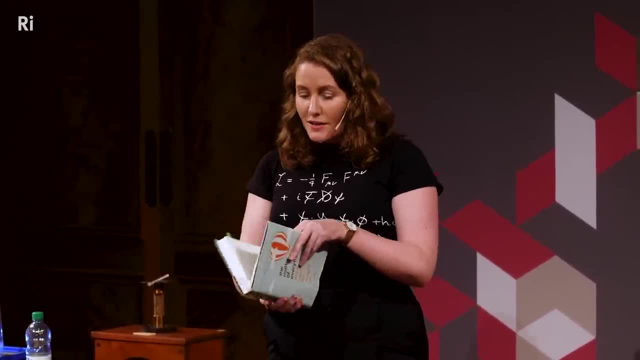 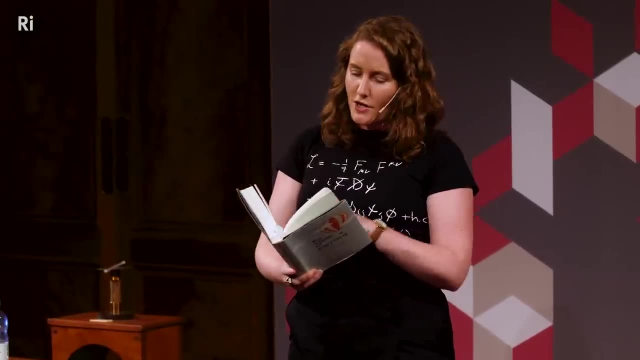 and the' age of other things on the earth. So, as well as revolutionising our understanding of the age of the earth, which we now know is close to five billion years old, let me read some of the other things that we know about because of this understanding of the transmutation of elements. 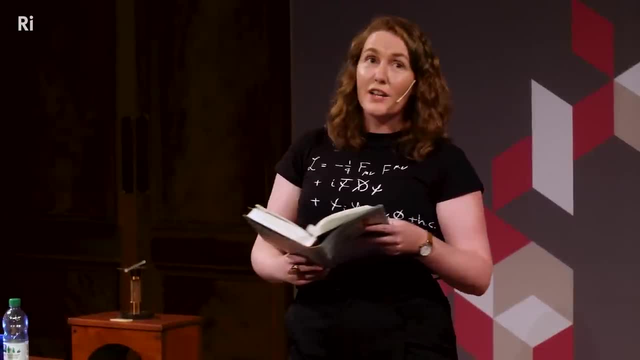 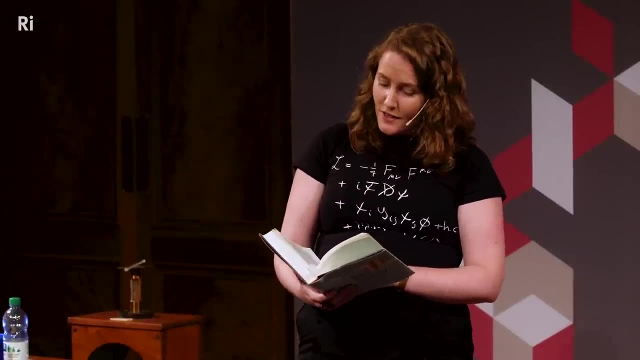 and radioactive half-lives and what we call radiometric dating techniques. So we know that the Shroud of Turin is a medieval forgery and we can put a date to the Dead Sea Scrolls. We know Homo sapiens migrated out of Africa not once, but over multiple periods, and we know how they spread. 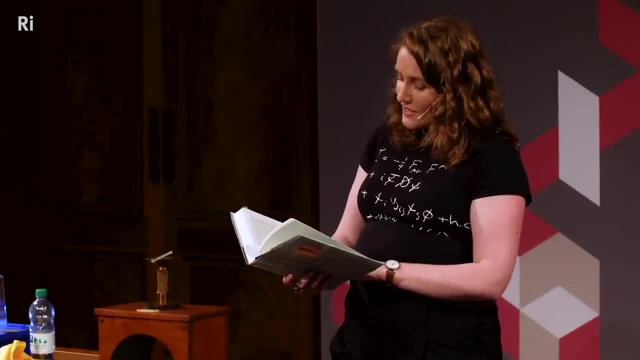 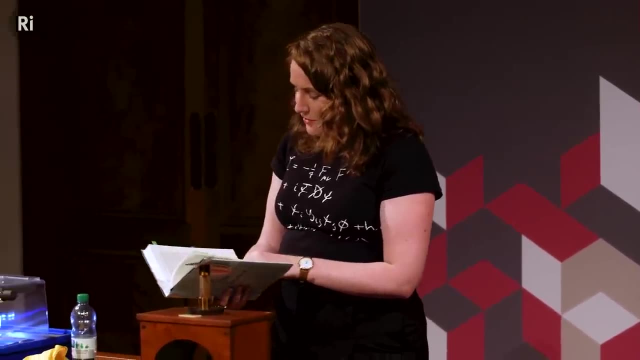 across the globe because we can date human remains like the 14,300 year old ones found in a cave in Oregon. In archaeology, we can put a time scale to objects, not just locally, but can compare them over different countries and even continents, letting us build a story of the prehistory of 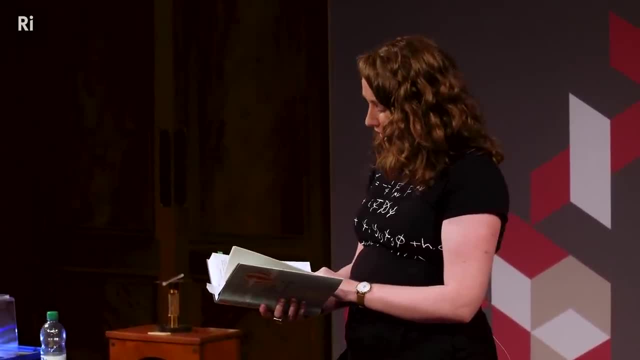 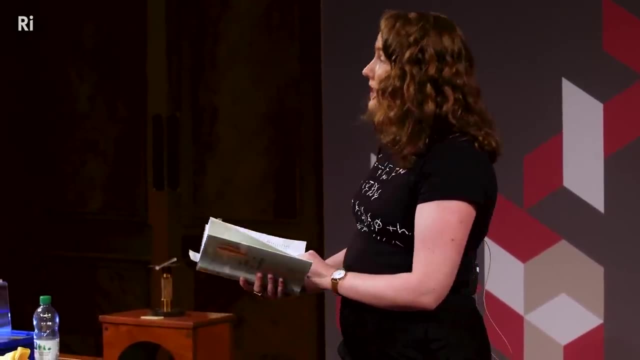 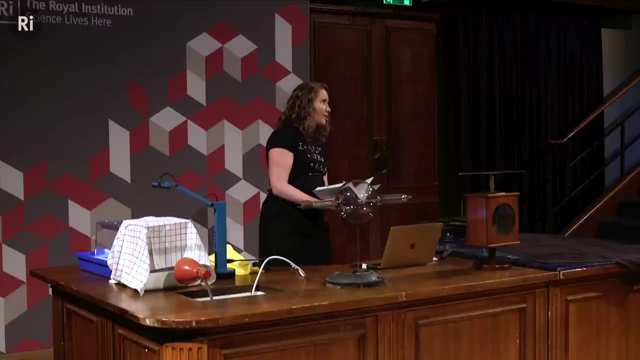 the world. We can date ice as far back as one and a half million years old to understand the ancient climate from ice cores, And it's also thanks to radiometric dating that we know when dinosaurs roamed the earth and the date of the asteroid, which appears to have wiped them all out 65 million years ago, which is a theory. 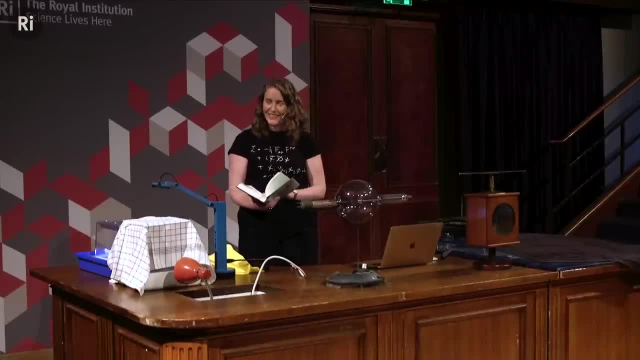 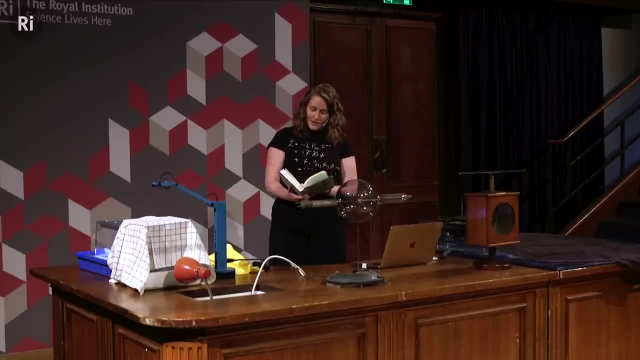 that went out of favour and is now back in favour. by the way, Going further back, we can identify the first evidence of fossils that might be animals, which is a kind of early sea sponge found in the 665 million year old rocks in the Trezona formation of South Australia, And I could 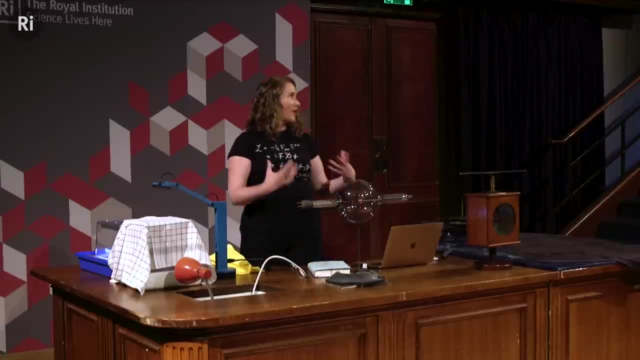 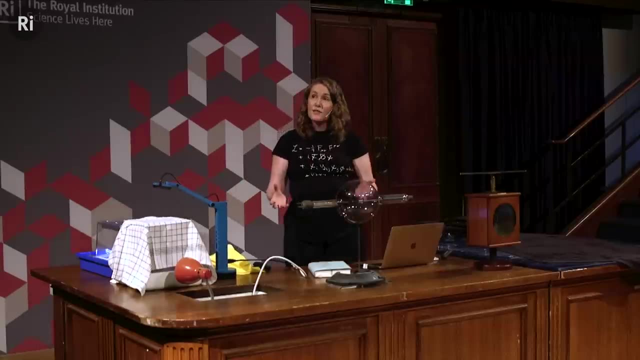 go on, but the amount of things that we culturally take for granted, the amount of things that we are granted of knowing in our society, either about prehistory history or our culture or art or archaeology, is astounding, And a lot of it we know purely because we understand that elements can. 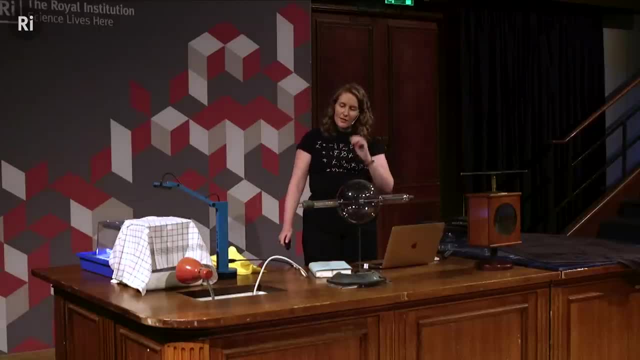 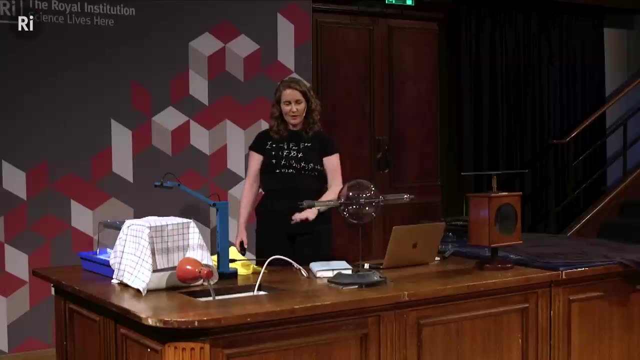 transmute one to the other because they're radioactive, which was an enormous change in the world Right. So the next experiment I have for you is one that's very close to my heart and also inspired the lovely balloon on the front of the book. 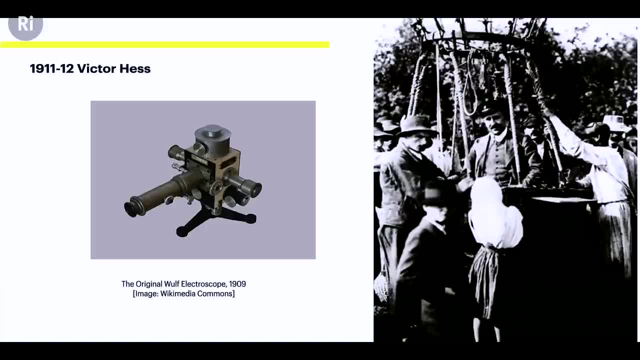 I showed you the electroscope before and you will have noticed over time- those of you who have been observing very closely, because I know you're scientists who like to observe these things- that the leaves that were splayed out very far have fallen back down and are touching each other. Now this might be because the air in this one isn't very well insulated, etc. etc. 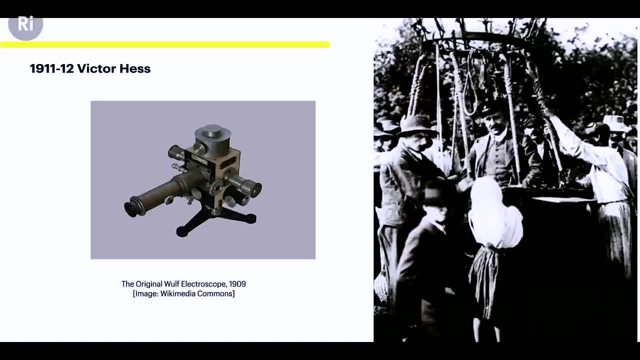 But this was an effect that was observed again around the turn of the 1900s- that even when there wasn't a radioactive source present, an electroscope or an electrometer would discharge over time, And what that meant was that there must be a source of radiation. 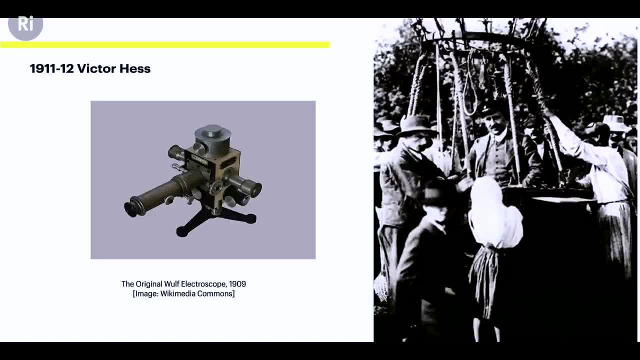 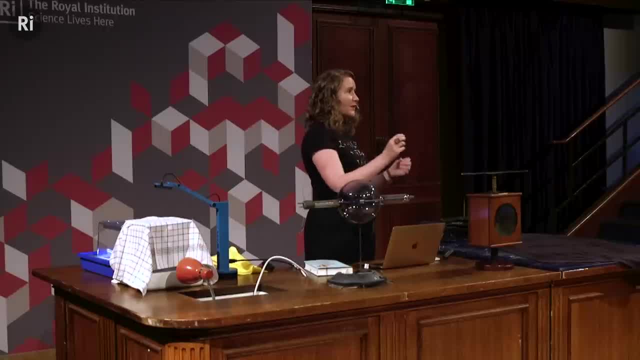 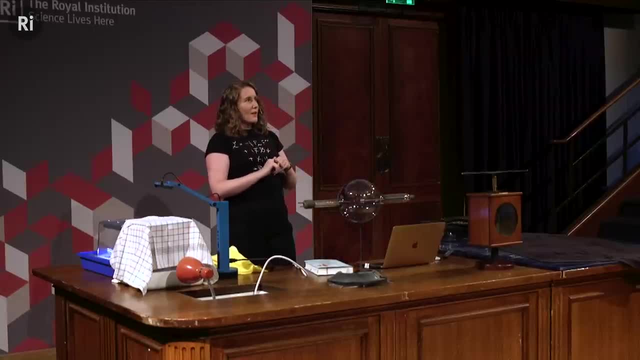 around them that they didn't know about or that they weren't bringing into the room. Because when a radioactive source decays, it decays into charged particles, and those charged particles will then discharge the electrometer or electroscope. Now people went in search of 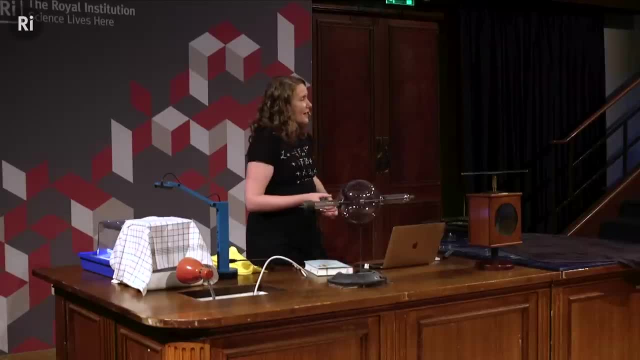 this extra source of radiation because the obvious place it must come from is from the Earth. So all the radioactive sources that we had, including those that were found by Marie Curie and Pierre Curie, were milled and refined from the materials at the Earth. 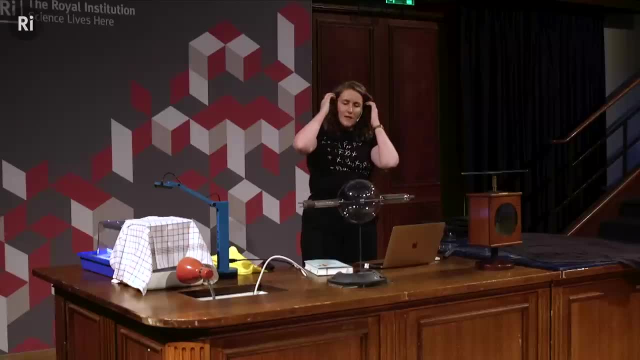 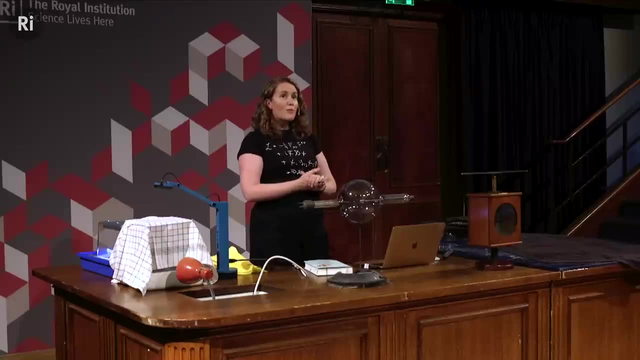 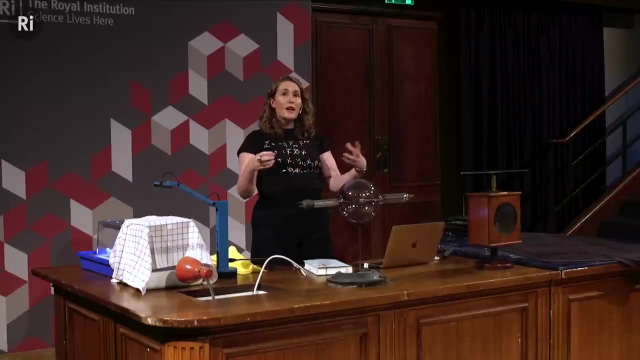 There are very small percentages, but radioactive materials exists on the Earth naturally, And so people took electroscopes and they went up the Eiffel Tower and they went down into the ocean and they went into rail bridges under the ground trying to detect this. 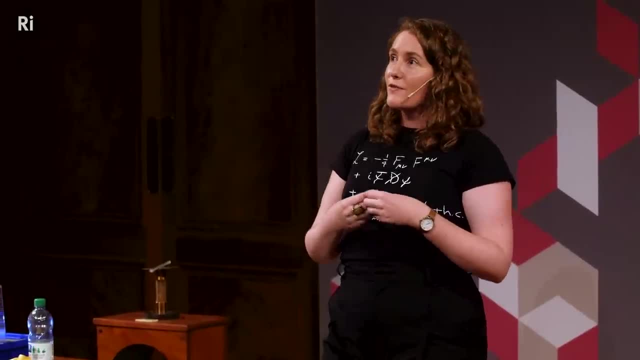 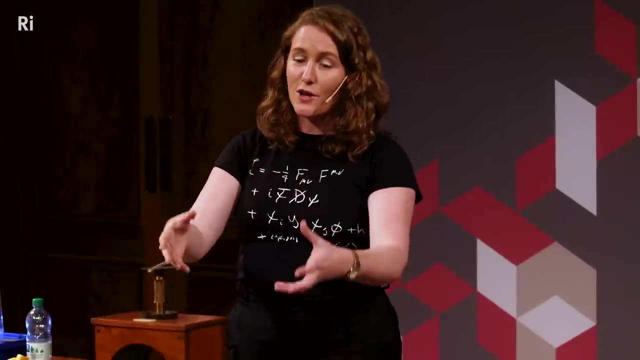 extra source of radiation and they couldn't find it. It was no good, basically, But part of the problem was their equipment. Now, if I told you I was going to take this electroscope and I was going to take it up in a hot air balloon, 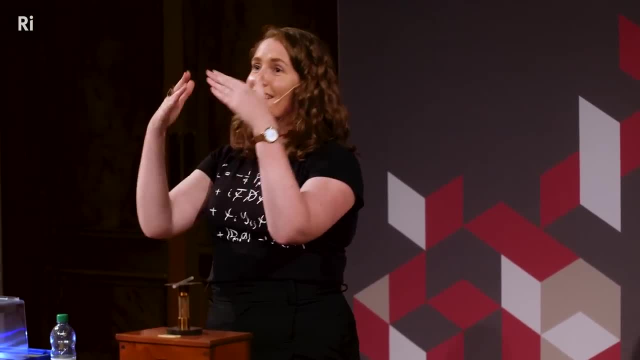 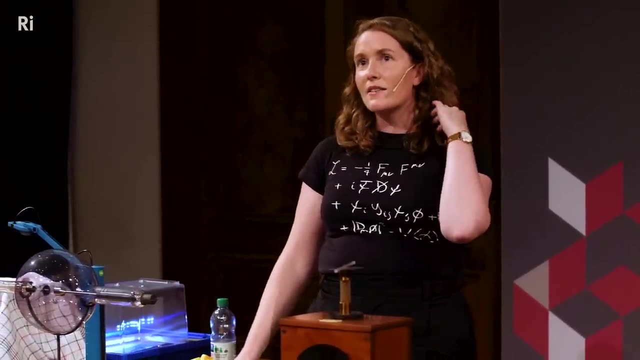 and measure things with it, you'd laugh at me, because clearly these leaves are going to wobble around and it's clearly not an appropriate instrument. So in about 1910, a Jesuit priest named Theodore Wolfe invented a better version and it looked like this: 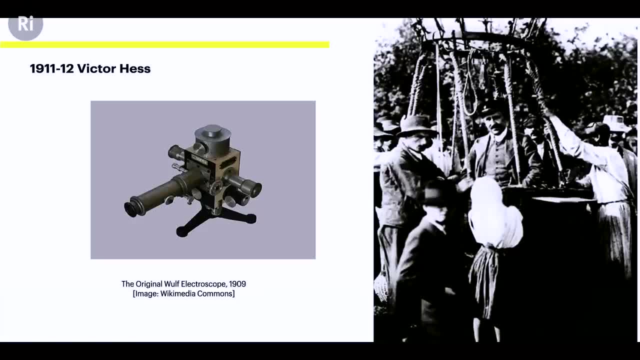 It had a microscope on the side and inside. instead of a couple of leaves, it had some wires instead. Now, I know this seems like a small thing, but it made the device much more robust, And so he wasn't the first person to go up in a hot air balloon. 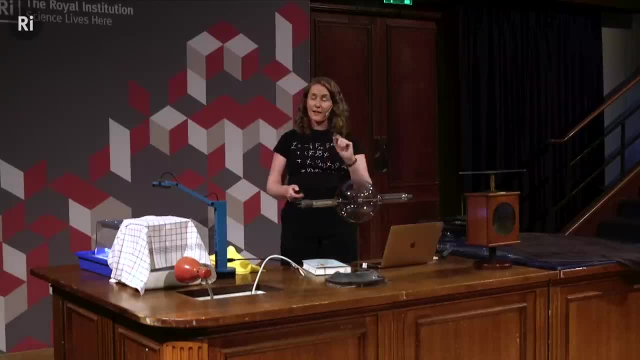 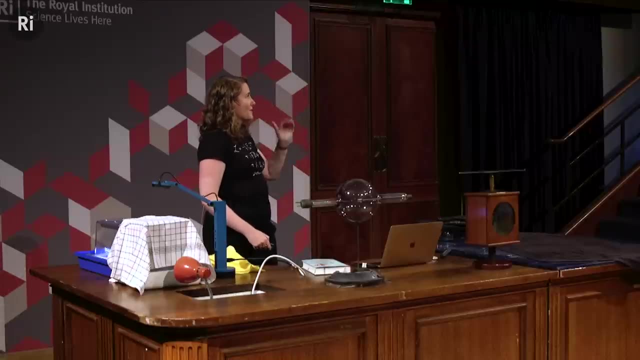 but Victor Hess was the first person to do this. well, And he took a couple of these Wolfe electroscopes and he did six balloon flights very high up in the atmosphere. He went up further and further and further, up to about 5,000 feet in the end, actually. And what he found was this: that as he left the Earth, the amount of radiation he was detecting decreased. That's what he expected. But as he went further and further up into the atmosphere, the amount of radiation he was detecting increased again. 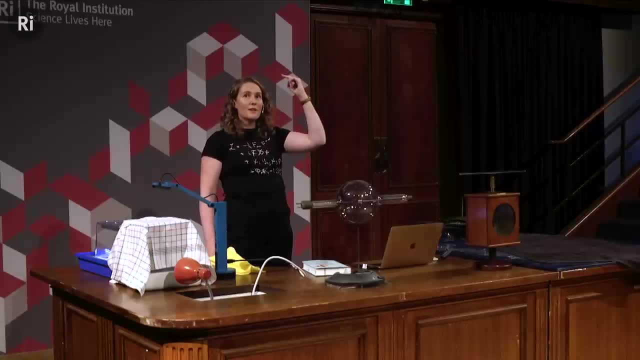 and it just kept increasing the further he went up And what Wolfe had discovered was cosmic rays, that is, a source of high-energy charged particles coming from space that had never been observed before, And he had no idea what it was or how it was being generated. 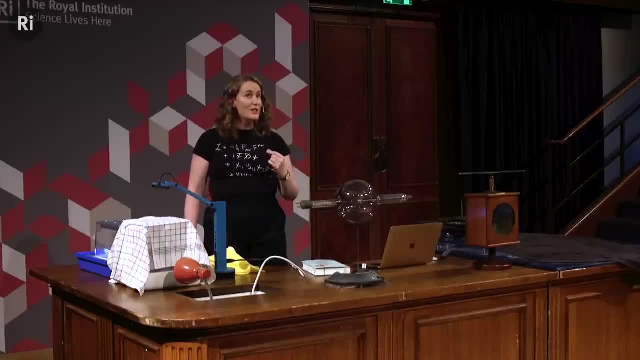 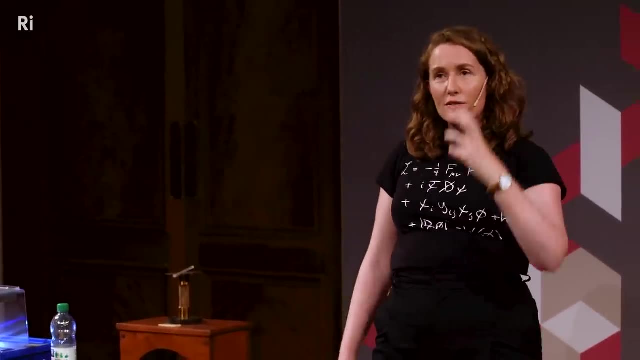 And one of the lovely things is, even now, to tell you the truth. we don't know how it's generated, We're still learning about it, But these charged particles would come raining down from space and were detectable in his experiments. 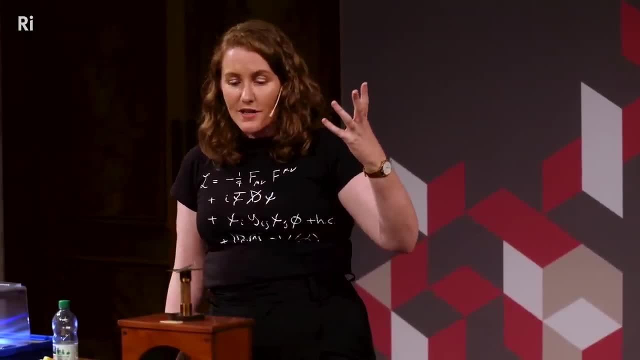 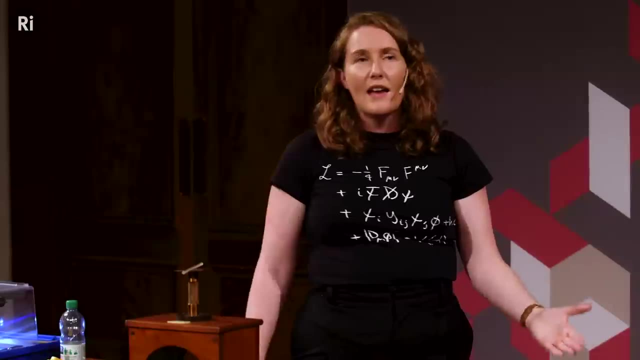 And we now understand that most of these are high-energy protons which come into our atmosphere and collide and they generate other types of particles which I'll talk more about. And at this point his story collides with somebody else working in Cambridge. 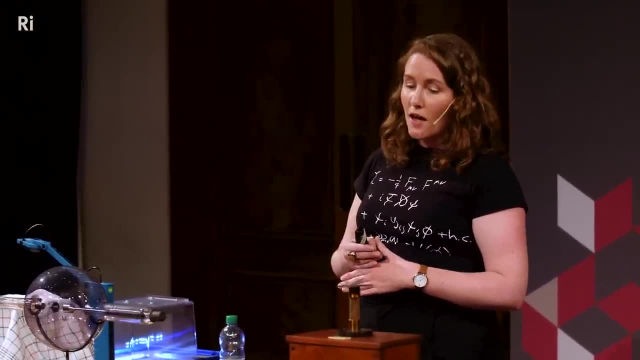 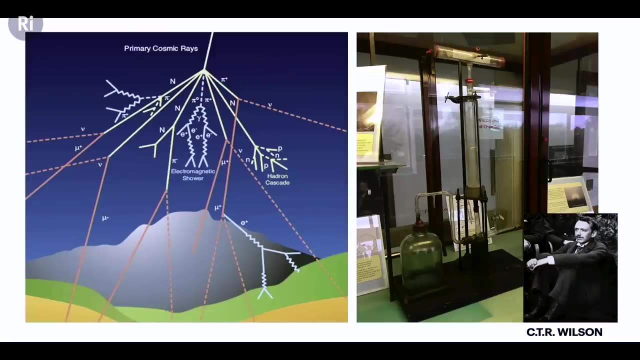 someone who was very interested in meteorology who's called CTR Wilson And you can see him sitting down there on the right. His first love was actually meteorology And he had built a chamber out of glass and the original version in Cambridge I've photographed here. 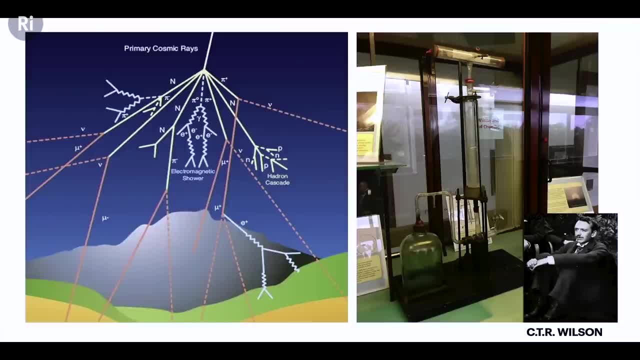 where the chamber could expand, and as it did so, it created clouds. And he'd actually built it to try and study clouds in the laboratory, because that's what he was interested in. But what he found was that when he put an X-ray source up against the cloud chamber, 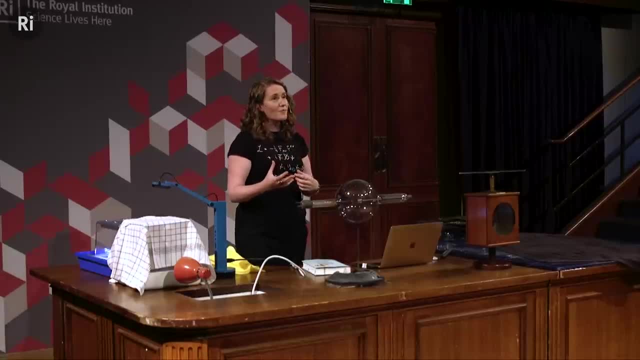 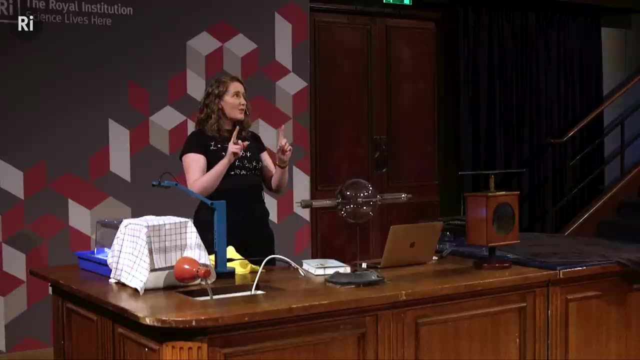 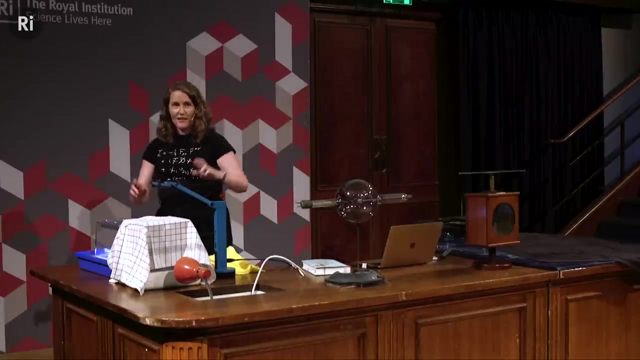 he could see the radiation from the X-ray source, And so he redesigned the whole experiment to be able to see radiation for the first time. And we've got a couple of cloud chambers over here and fingers crossed they're working. That's why I've got two of them. 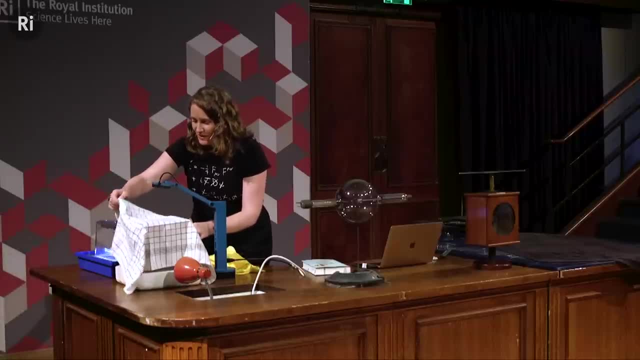 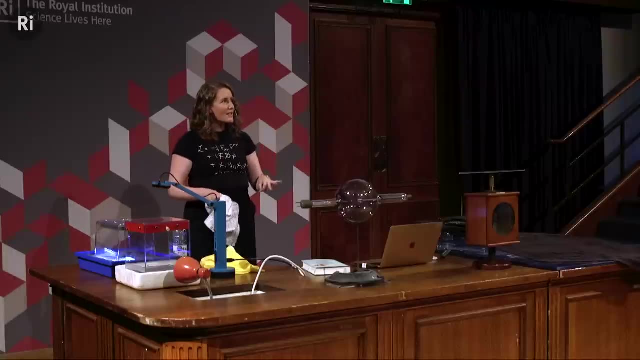 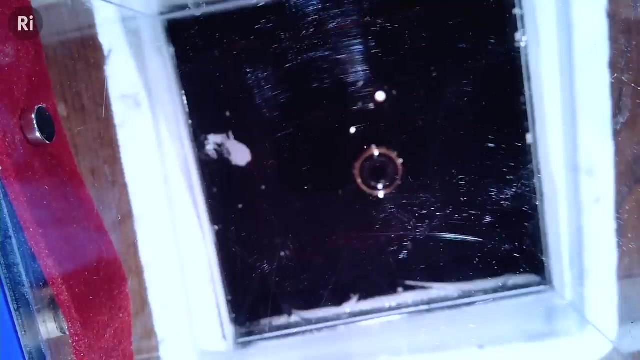 Two for redundancy. So I've got a couple of things to show you over here, because it is quite an astounding thing to be able to see with your eyes, for the very first time, the effects of radiation. Now let's have a quick look at this one. 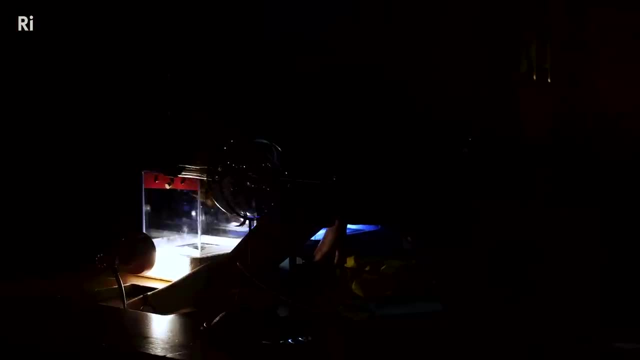 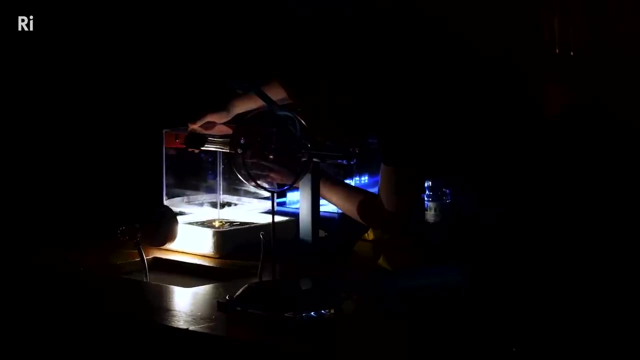 If we could bring the house lights down. Tom, Let me pop a light on All right, this one's behaving badly, so I'll start over on this side. This one. have we got the Yep, we've got the camera up. 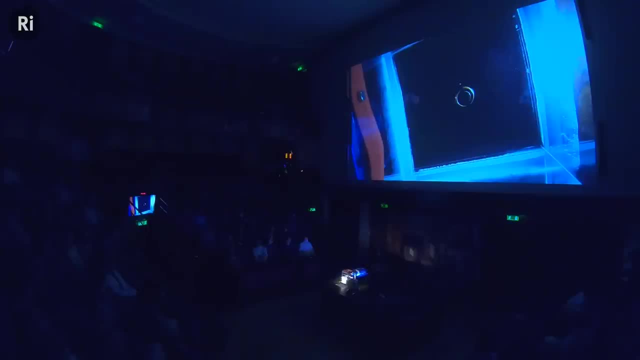 So, okay, I wanted to show you this one, but it's not currently working so well, because this is another original object that we have here. I was talking about radiation before and Marie and Pierre Curie. Well, in 1904, Marie and Pierre Curie travelled over here. 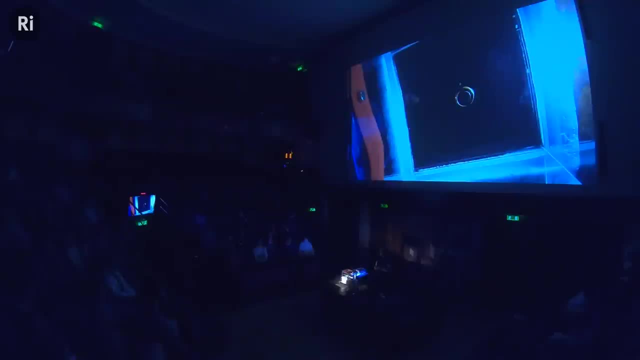 to this very lecture theatre, to the Royal Institution, to talk about radiation, And they brought with them a source of radium that they had refined themselves in a container, And Charlotte, the archivist, has given me the lid of that container, which still has a low level of radiation. 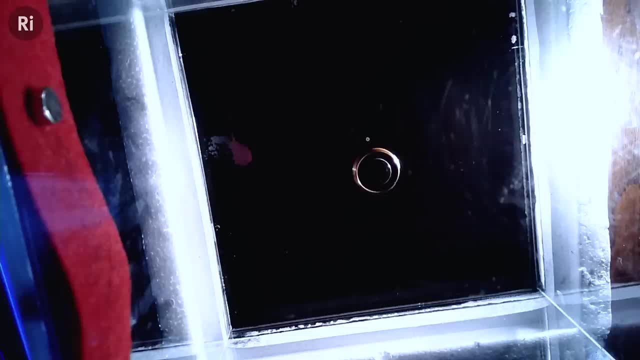 And that's the object you're seeing actually sitting inside the cloud chamber there Now. sadly, because it's taken a little while, I don't think we're going to see much on that one at the moment, but we'll see, Tom, if you want to come and play with it if you're around. 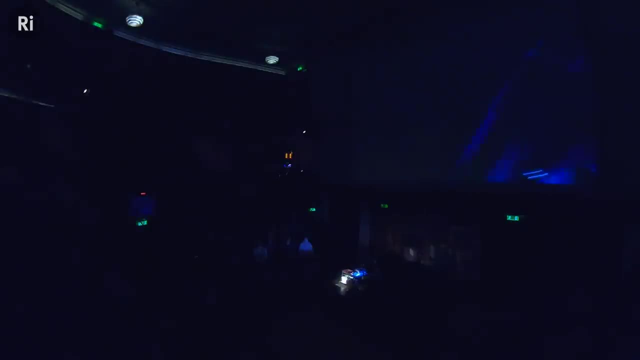 feel free to come and try and reset that one. This is a real live experiment, so it doesn't always work first time, And I'm going to try to show you this one instead, So OK, so first of all, what I'll point out that you're seeing here: 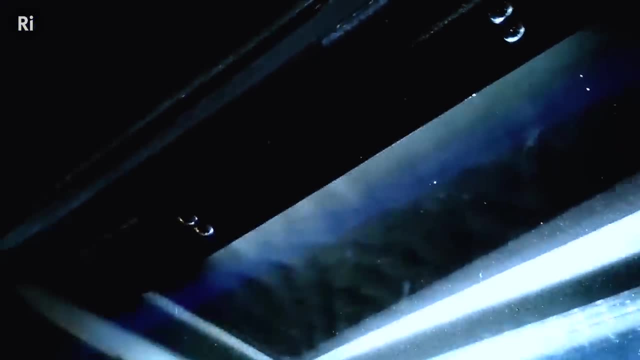 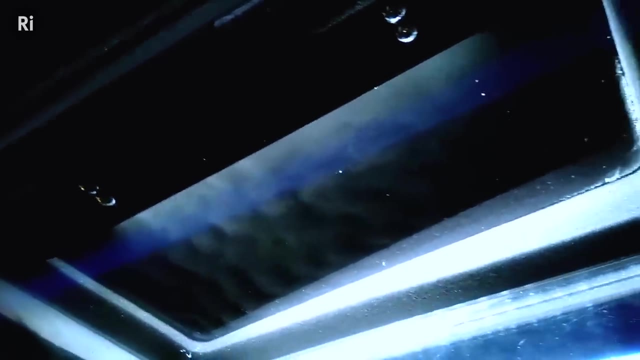 is. you can see some sort of cloud-like stuff trailing down right. I'm pretty sure you can see that. So what is happening inside this chamber is there's a vapour of alcohol which is falling toward the bottom, where I've got dry ice. 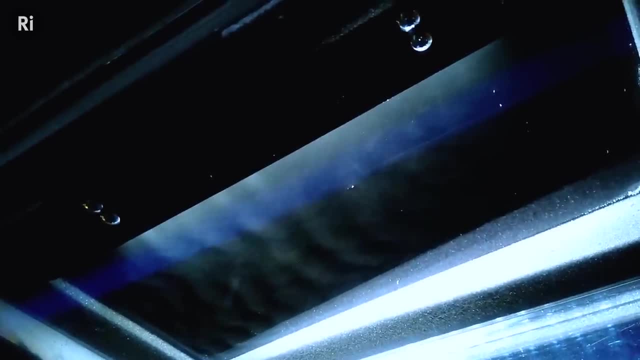 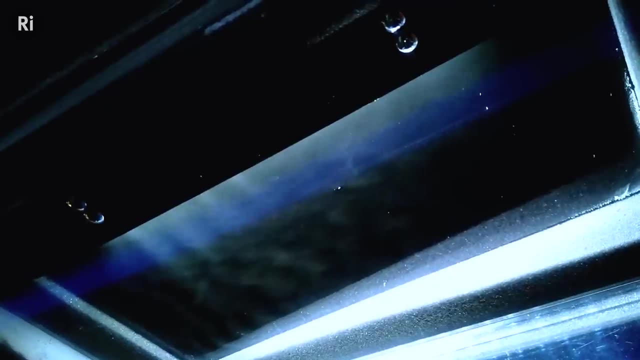 And dry ice is at about minus 70 degrees, and so it's creating a temperature gradient, And so the vapour falls down to the bottom and forms a layer that's called a supersaturated state, And what that means is the alcohol the vapour really wants to condense and form clouds. 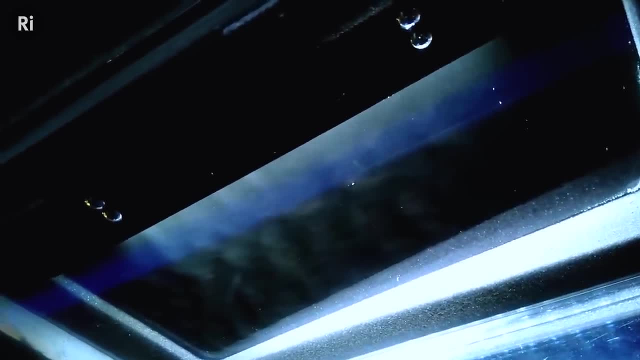 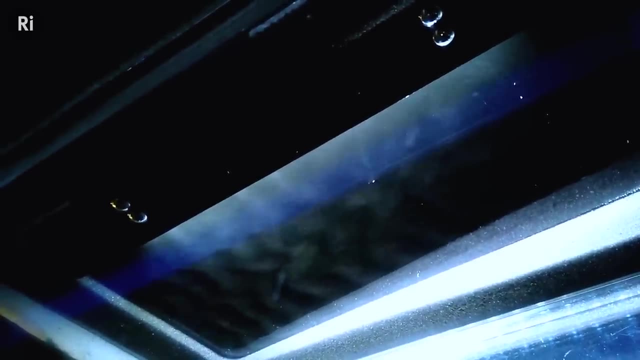 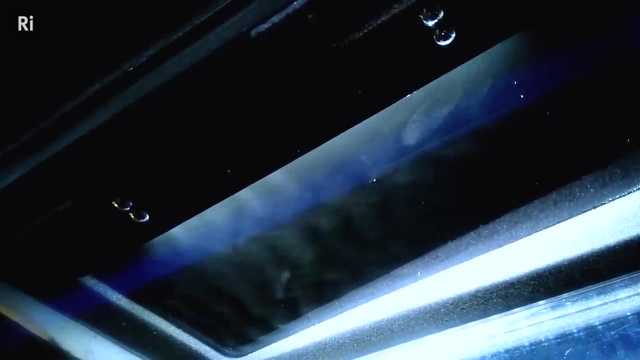 but it needs a little little bit of energy to do so. Thanks, Tom. And so if you watch this very carefully, if I can actually hold it stable, there we go. you can see just occasionally a little cloud trail. There we go. There's a few, There's a big fat one. 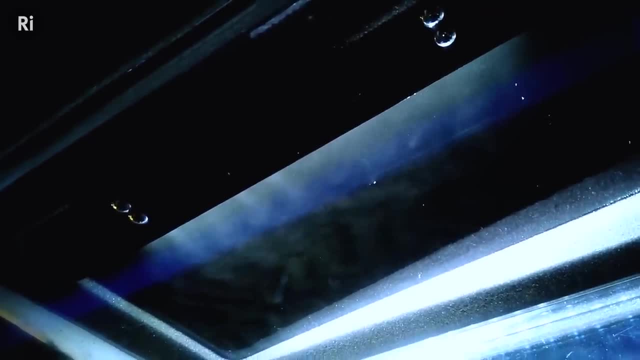 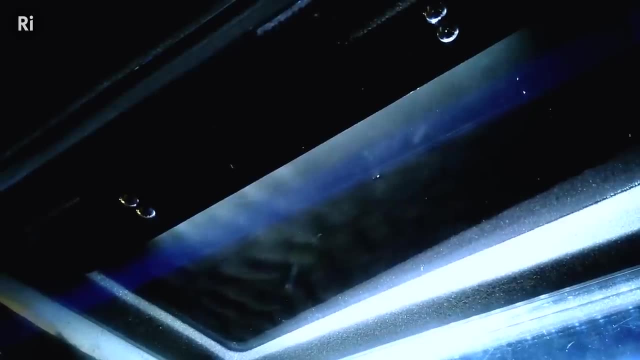 And now you'll see also some thin wispy ones that come through. Now I'll point out here that I do not have a radioactive source in this second chamber, So what we are seeing here, if we see tracks, There we go. There's one Another one. 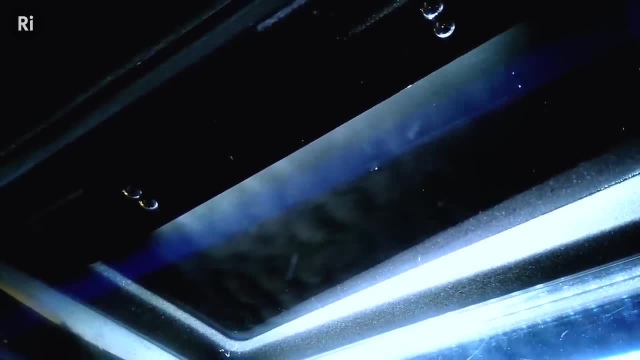 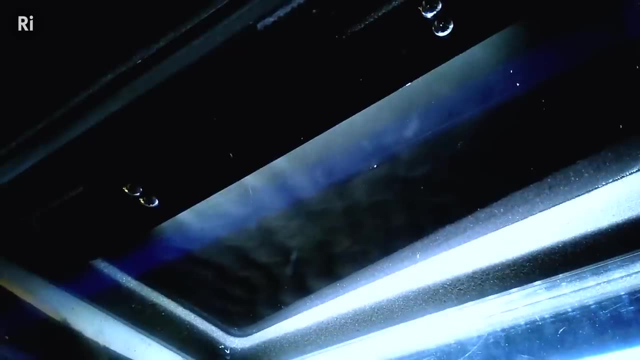 What we're seeing here, if we see tracks, is actually the cosmic rays that Victor Hess created, or perhaps some radioactive decay of, say, radon gas in the air in the theatre or of some elements in the Earth which are coming through. 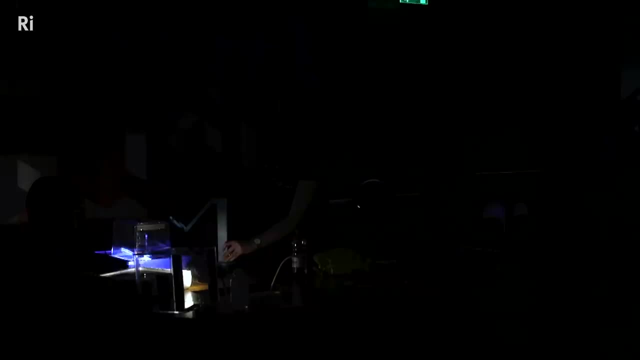 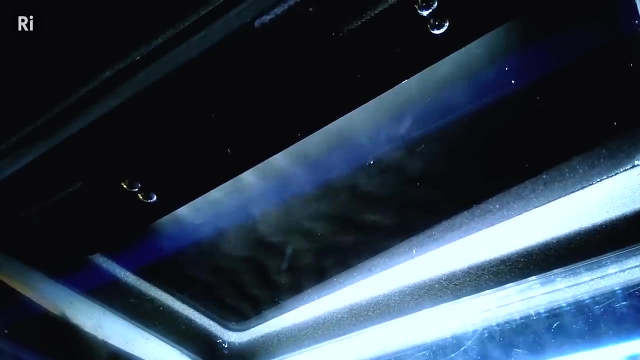 But some fraction of these are going to be from cosmic rays. I'm going to sit there and let it. I actually could watch it all day. It's quite mesmerising. One of the astonishing things really is that you can build a chamber like this at home. 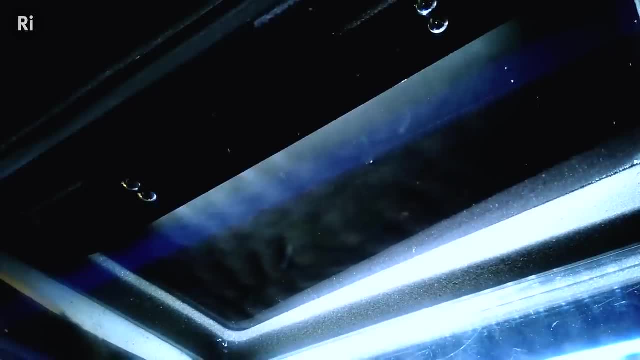 if you can order some dry ice from a cocktail maker or a supplier. It's actually quite easy. It's propanol, by the way, the type of alcohol that's used, And you're welcome. We'll leave them running. So you're welcome, if you're in the theatre, to come down and have a closer look afterwards. 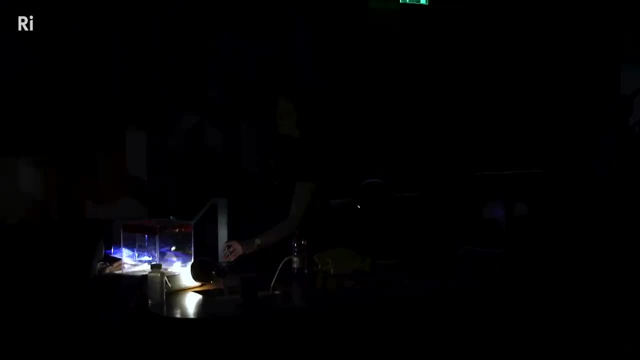 Especially at this second one that Did you. Yeah, you need to wipe some alcohol off, just to It was a bit sort of saturated. Yeah, All right, so we'll get that one reset up. So hopefully, what you'll be able to see, 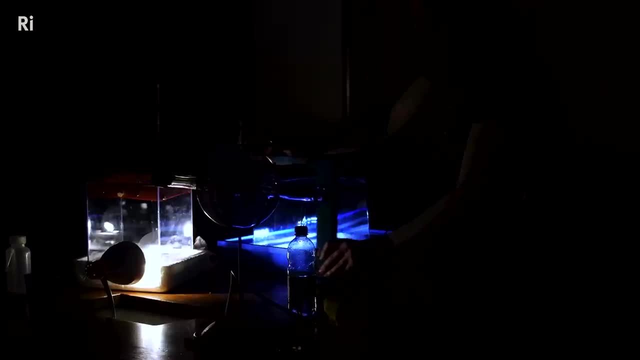 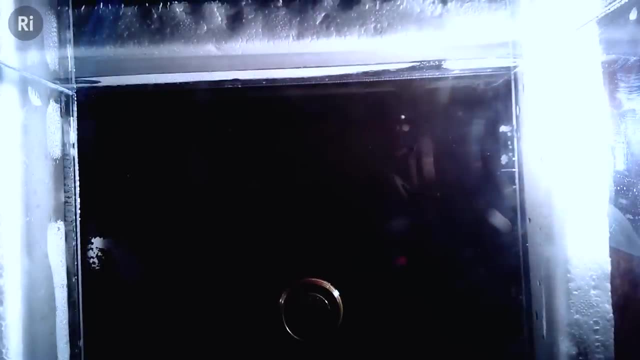 So this one, we're looking at cosmic rays, but hopefully, if you come down at the end of the lecture, we'll be able to look back over at this other one, which hopefully by then will be showing some nice tracks from the radioactive source that I've put in there. 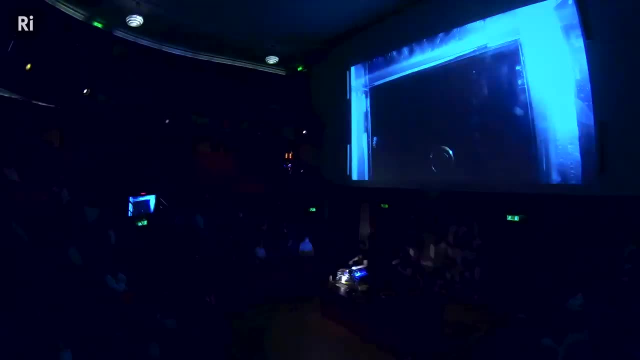 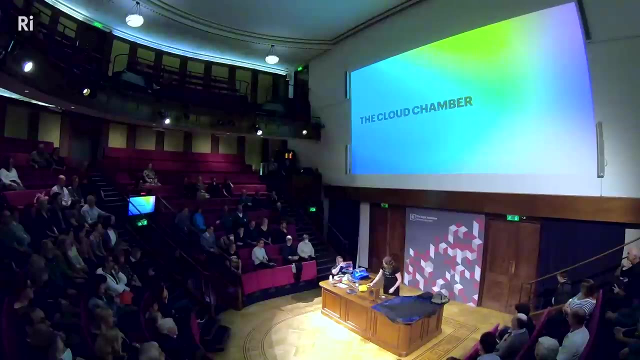 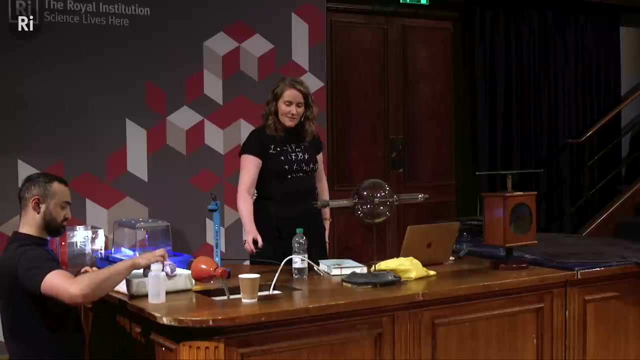 OK, if we can bring the house lights back up again. Thank you. This is why we always have redundancy in case one of the real experiments doesn't work. The thing is, they're quite temperamental. If they get too saturated, they lose their state. 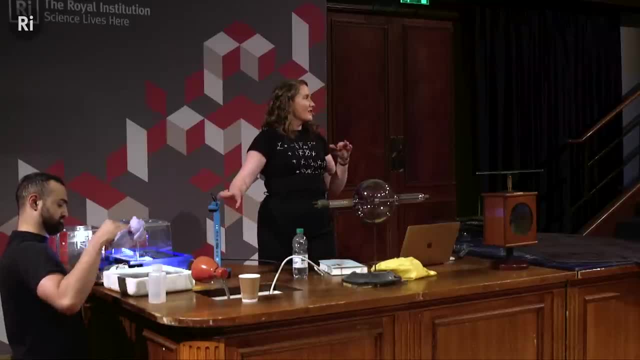 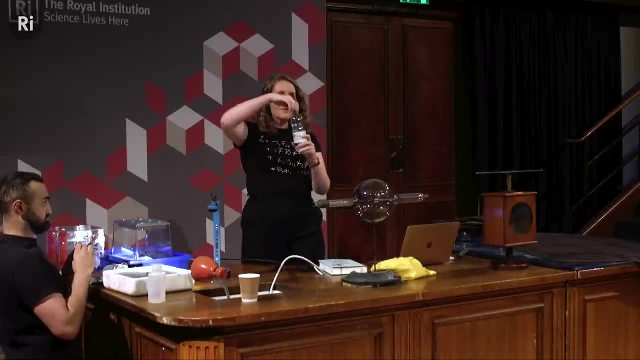 Now this is actually a later version, invented about the 1930s, which uses this so-called diffusion method, whereas Wilson's original one used a pressure difference, which is what happens, sort of, if you open a bottle, If you open a bottle of soft drink, and you see that cloud in the top. 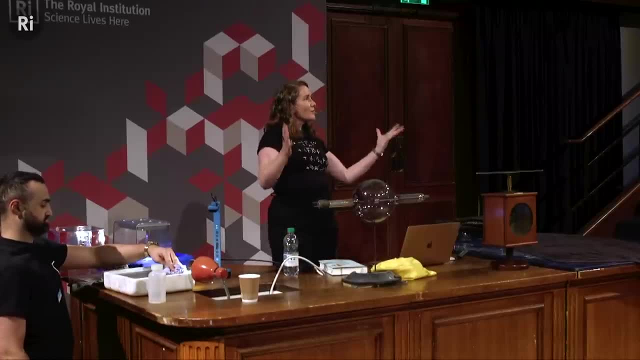 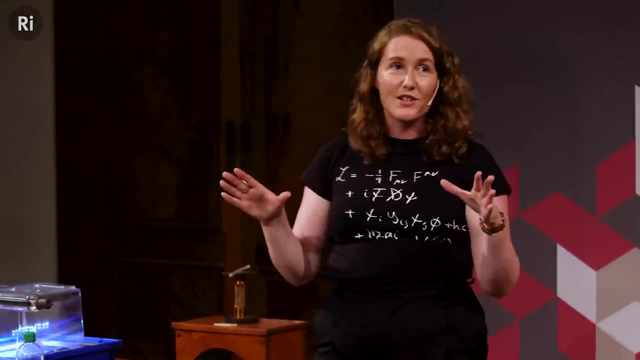 it's sort of the same effect. OK, so what happened with the cloud chamber? Well, there was an incredibly adventurous journey. that happened after the invention of this device, because now that you could see and photograph the passage of charged particles for the first time, 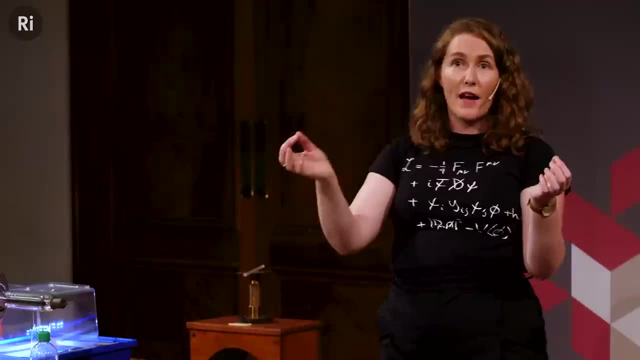 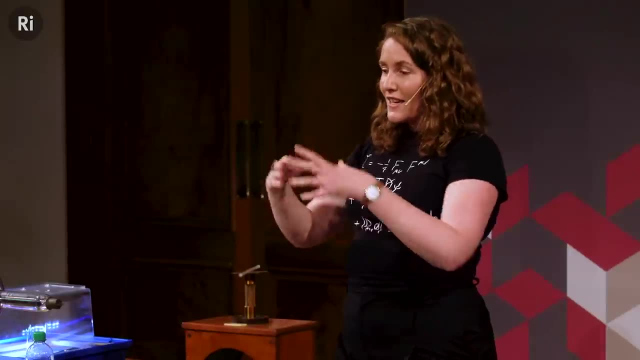 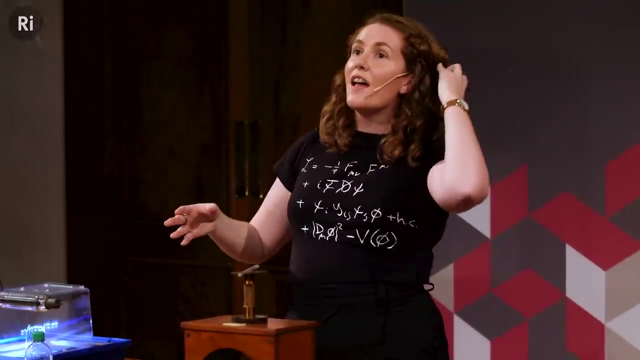 you could just look at the tracks that we were seeing. So those short, fat ones were alpha particles, Long, thin ones are probably electrons. And then, when they started taking these chambers, putting them in big magnetic fields and leaving them and photographing them for a long, long time, 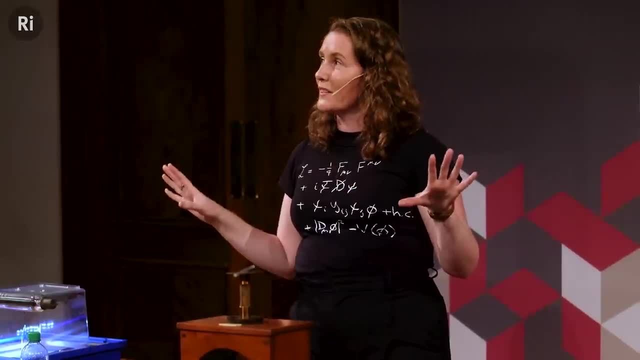 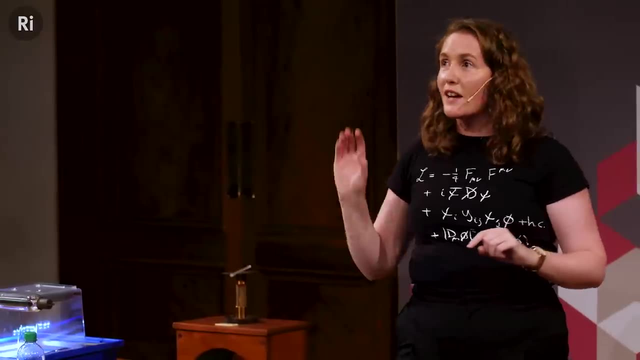 what happened was they found other particles that they weren't expecting, that played no role in ordinary matter, And the first one of those is called the positron, which is like the electron, but it's the antimatter version That was found in 1932.. 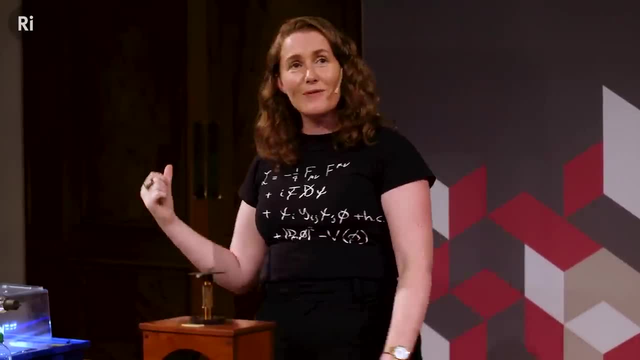 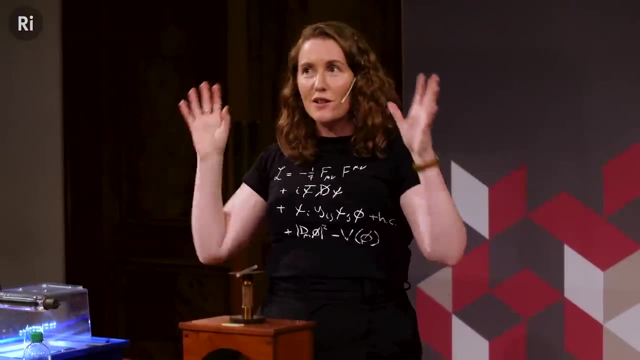 And then, just four years later, they took one of these on the back of a big flatbed truck up a mountain in California and in these inhospitable conditions- you know it's really cold and windy and stormy up there- they left the thing running for about six weeks on end. 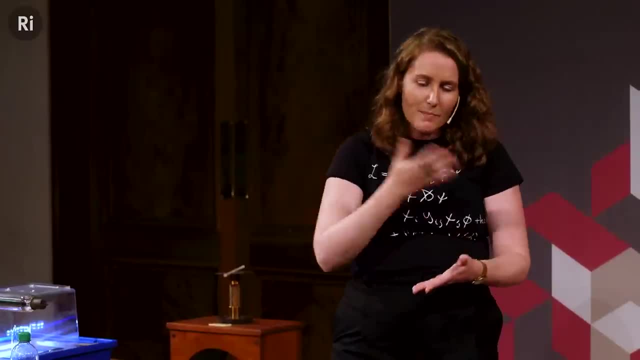 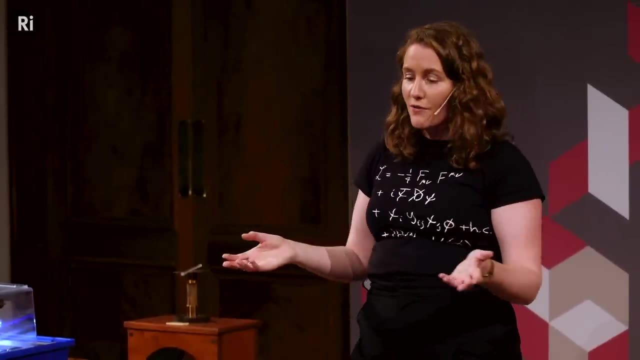 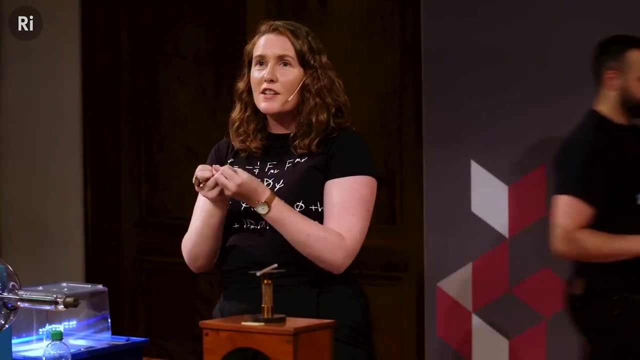 taking photograph after photograph after photograph, poured through all of these pictures and then found another new type of particle called the muon, which was like the heavier version of the electron, And this sort of revolutionised our understanding of physics, because, if you think about the fundamental particles that make up nature, 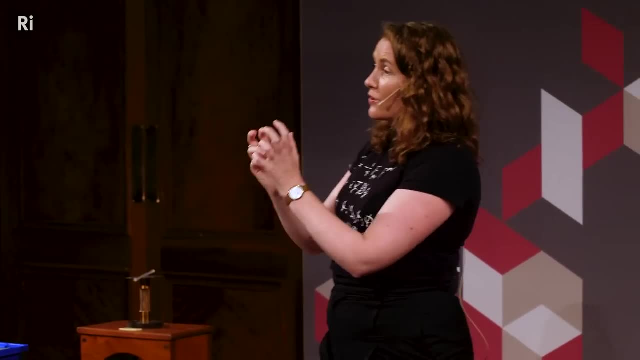 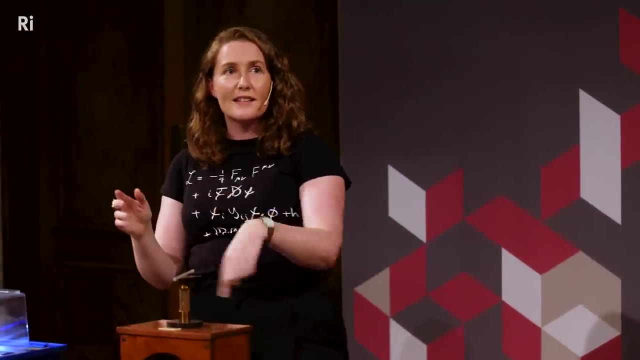 we normally talk about atoms. Inside the atom there's the nucleus, which by this point they knew about. the electrons around the outside and inside the nucleus is protons and neutrons, And later we found what those protons and neutrons are made of. 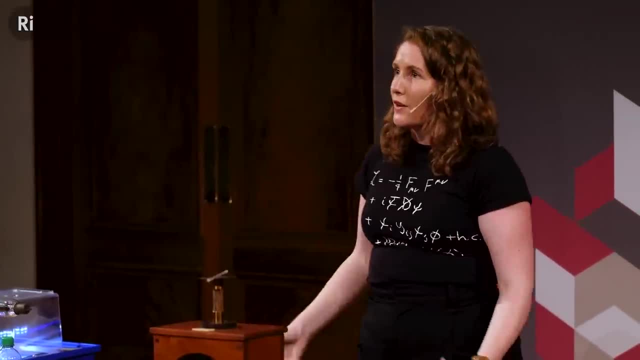 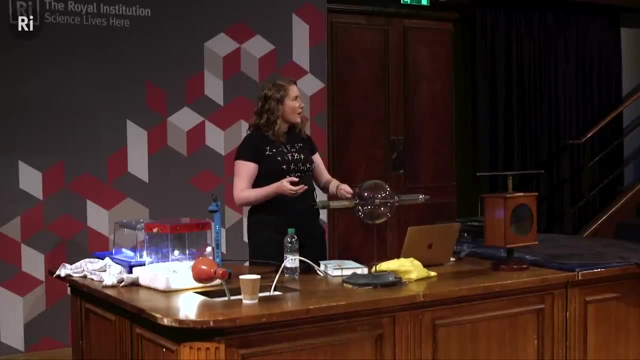 And here we have particles that don't make up the matter around us, right? They're completely different, And there was one theorist called Isidore Rabi who reacted to the muon discovery by literally just saying: who ordered that? Like it was so unexpected. 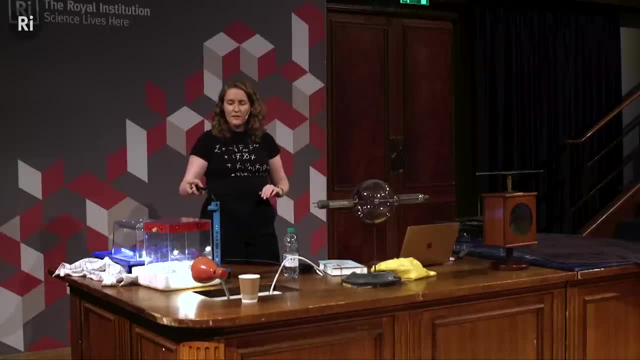 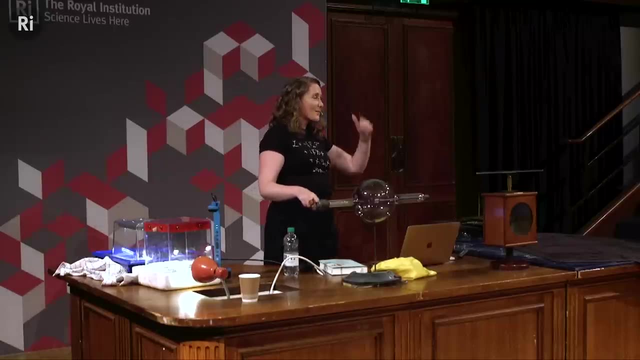 Now, at the same time as this, it was really annoying to take a really you know, like unpredictable chamber up a mountain, or let alone up in a balloon, or up to even higher altitudes and take measurements with it. 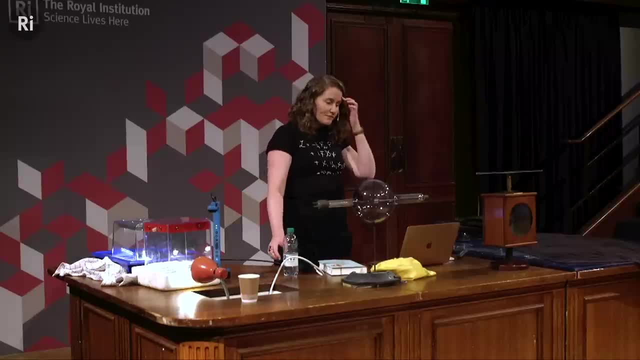 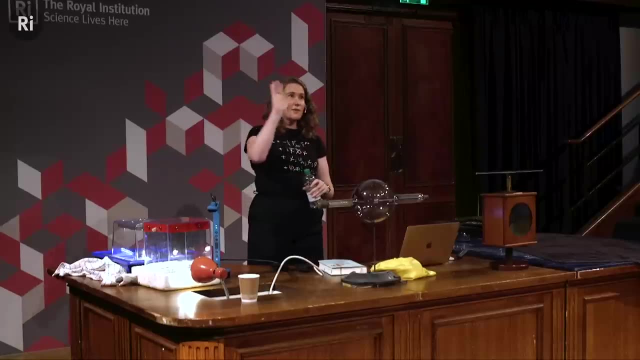 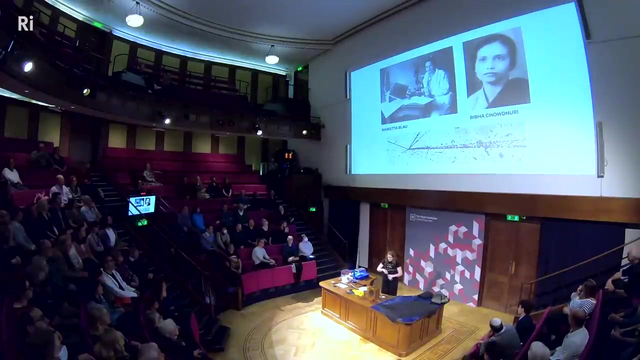 So instead there was a different invention, using photographic plates or photographic emulsions, made by a woman named Marietta Blau, who, I'm guessing, most of you have never heard of. I think, yeah, So she was working in Vienna, unpaid. 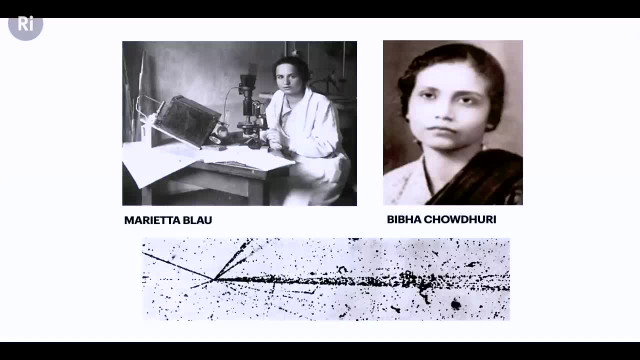 and she invented this technique using thick photographic emulsions. She worked with Kodak and Ilford and other big companies to develop them. She developed this technique of being able to leave instead of a chamber which you had to photograph all the time. 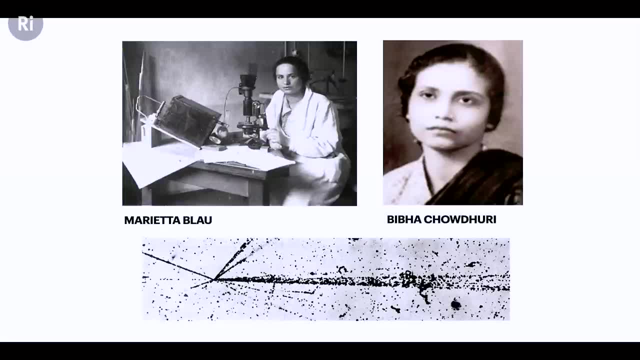 she'd leave these thick photographic plates up at altitude in the mountains for months at a time, and then she could take them away and she could process them, And by doing so she actually found some quite remarkable things, including the image here which they referred to poetically as a star of disintegration. 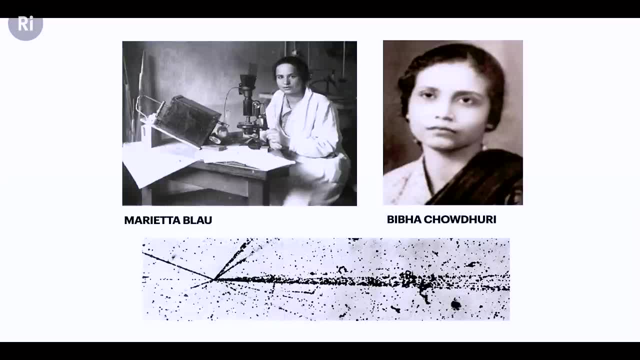 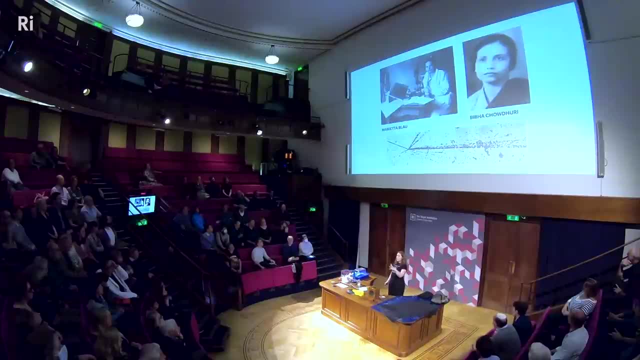 which is where a high-energy charged particle is coming in and the nucleus of an atom is decaying and throwing out tracks in all different directions. So Marietta Blau was a pioneer of this technique and there was another woman in India at the time. 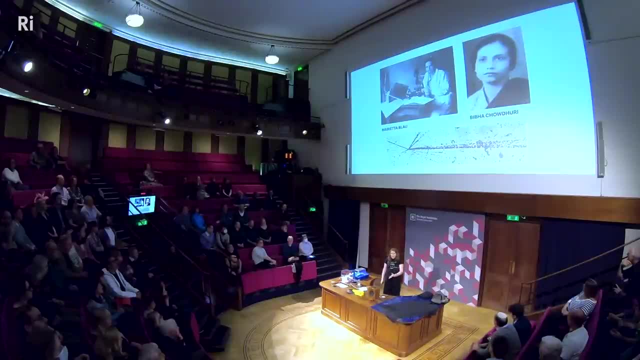 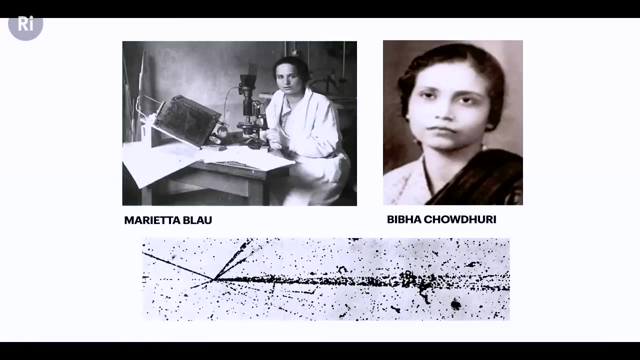 who picked up this technique and used it as well, but because we ran into World War II at this point her supply of emulsions was not very good. But Biba Chowdhury, who I'm guessing you've never heard of. 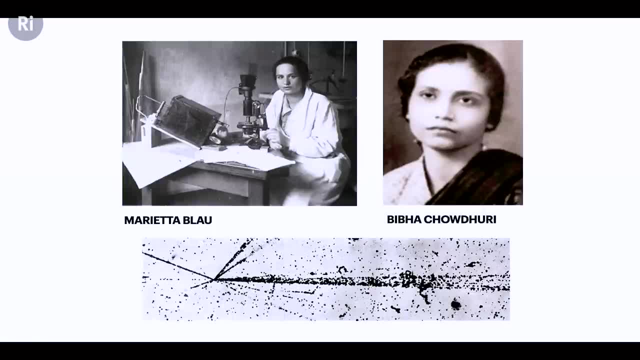 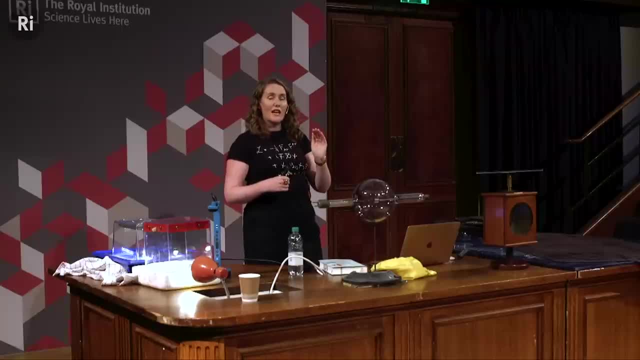 because I hadn't. she's one of the people I learnt about in writing this book actually found another type of particle, similar to a muon, but slightly heavier again, And it's a type of particle that we call a pion. 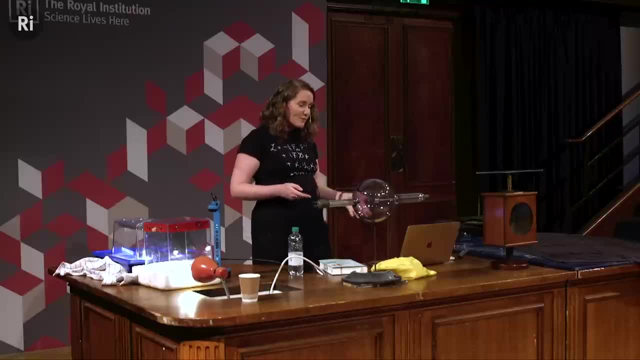 There's a couple of particle physicists in this room, so this will make sense to them, but to anyone else, it just means we were discovering more and more and more, more and more particles. right, But one of the important things about Blau and Chowdhury. 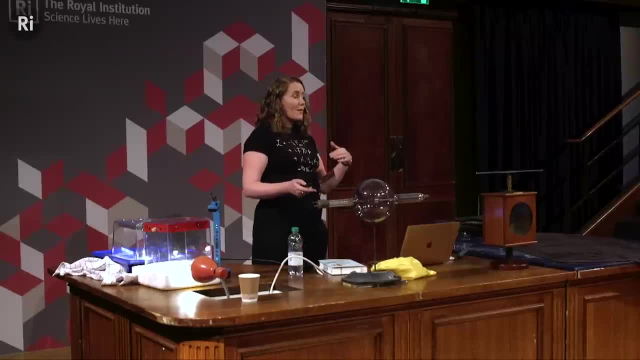 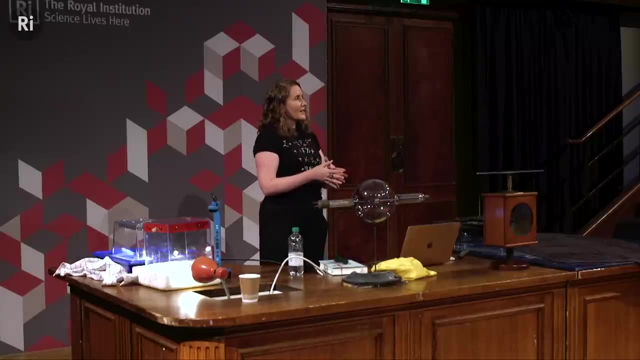 and some of the other women that I've mentioned, including Harriet Brooks- not Marie Curie, because we know and recognise her work very well, because she won the Nobel Prize. the important thing about these women is that their stories weren't written down, weren't recorded. 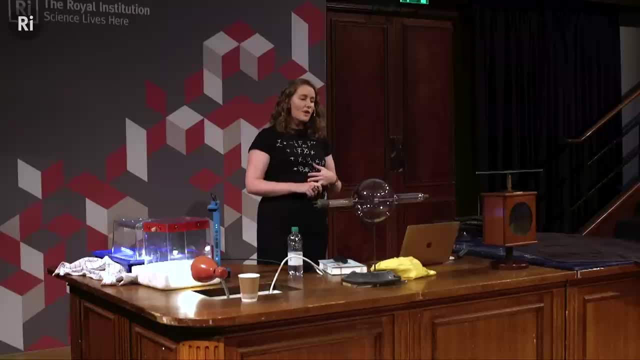 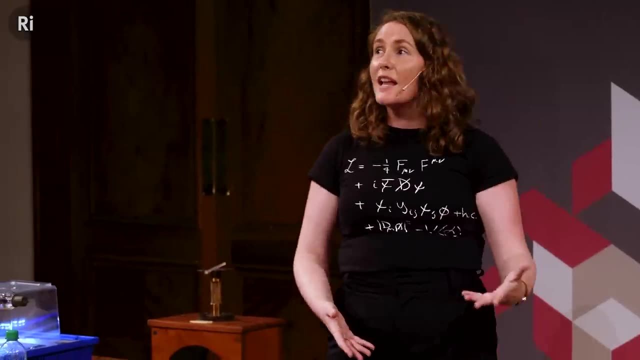 and they really weren't acknowledged for the work that they did. And one of the difficulties I had in writing this book, in writing their stories back in for their amazing discoveries, is that we don't know anything about their personalities or their lives actually. 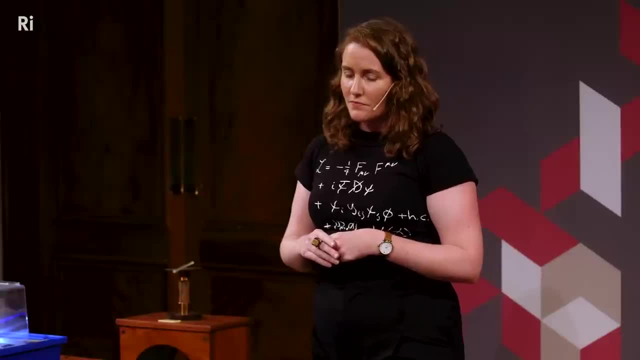 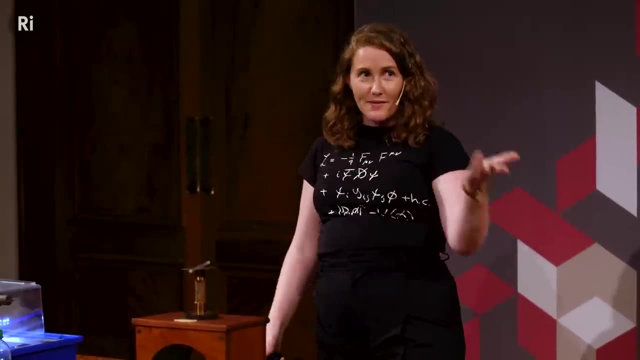 because it just wasn't recorded and it wasn't written down. But let me tell you what happened after the discovery of things like muons, because this is, as I've said, I've talked about, changing the world, right? So one of the amazing things that happened with muons- 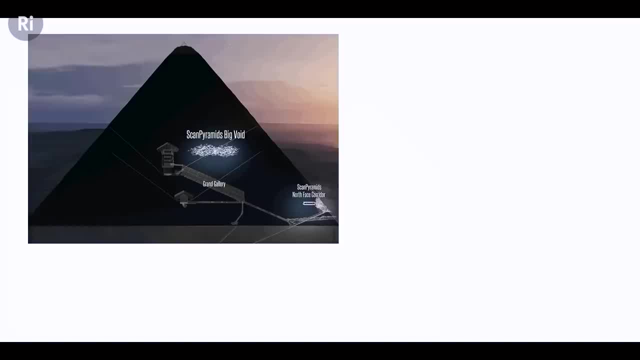 is. we've developed over time, taking cosmic ray muons and using them in technologies to do things which we couldn't do before, And one of the things that they did was to use them as like a giant X-ray scanner through enormous objects, because they can travel a long way. 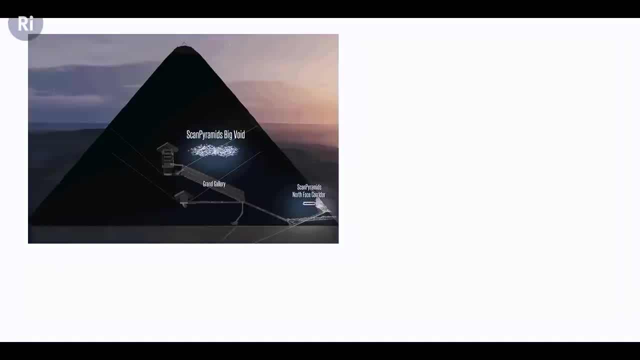 through metres and metres of rock And in a project called Scan Pyramids in Egypt, they actually discovered a new room in Khufu's Great Pyramid in Giza using this technique, So the muons can travel sort of straight through and be detected. 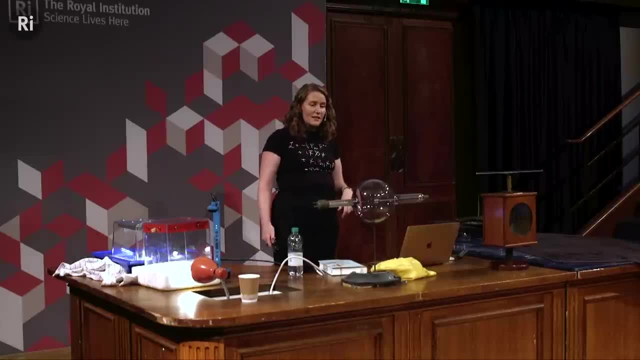 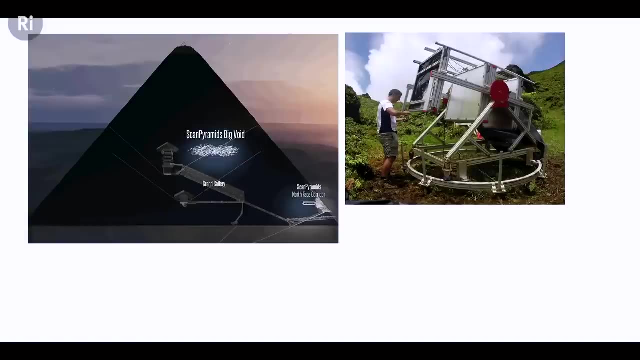 mostly using Marietta Blau's emulsion technique, And this is what a detector like that looks like, and they don't just use it for pyramids, they're now using it for volcanoes as well, to actually see the magma and the changes in magma in volcanoes. 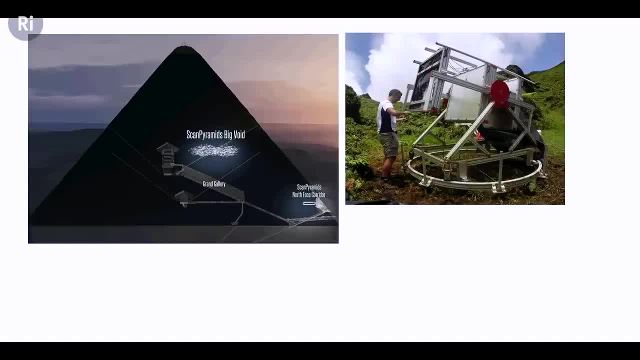 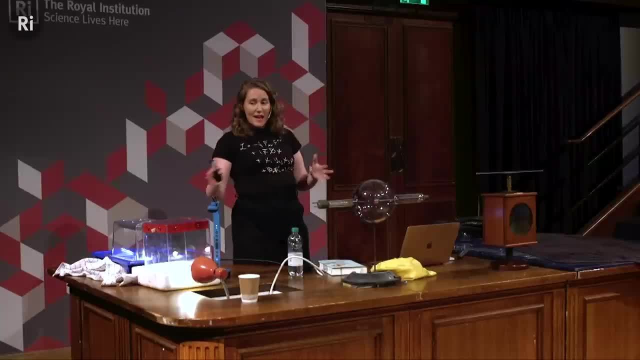 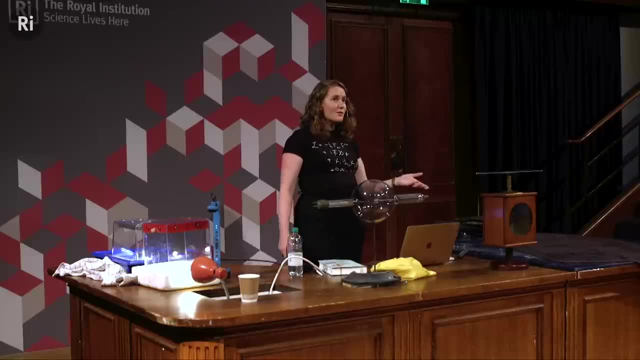 So instead of We're used to having X-rays of sort of small objects and bodies and dogs and things like that, but now understanding cosmic rays and having the technology means that we can actually use naturally occurring radiation sources which are around us all the time. 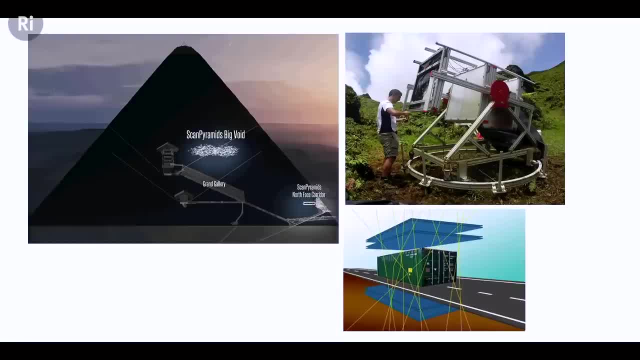 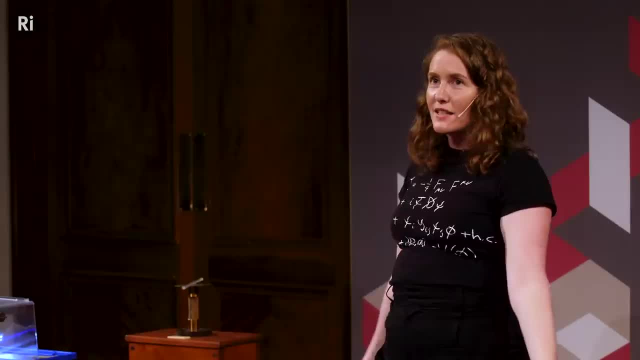 to measure things which we simply can't do, Things we simply wouldn't have known how to do before. So, just to summarise this space of 20 years, we had this huge overhaul in our understanding of physics And, along the way, in the book as well. 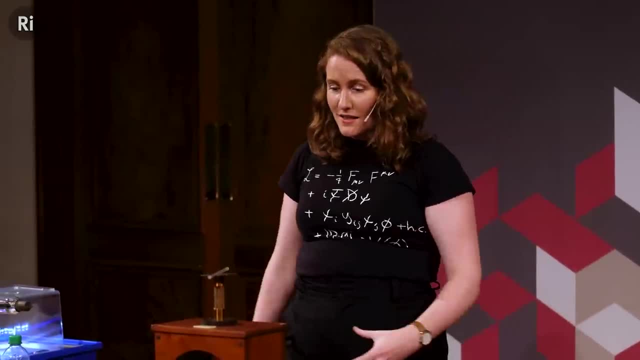 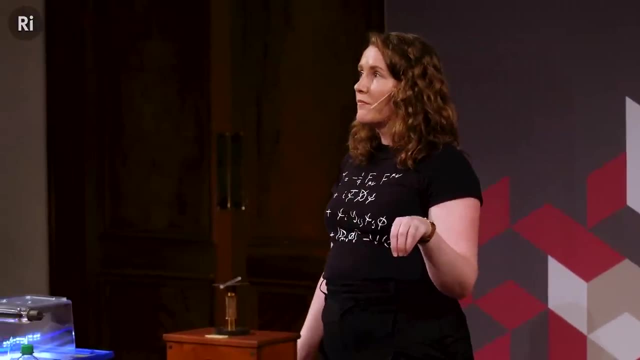 we get the development of quantum mechanics at the same time right, And it all ties together. So we understand that the atom was no longer the smallest object, that some atoms weren't stable over time and that that change was an inherent part of nature. 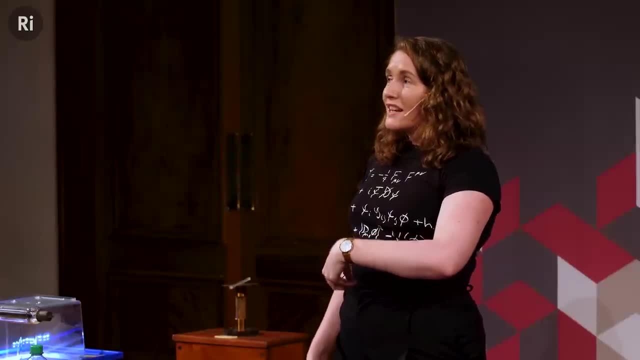 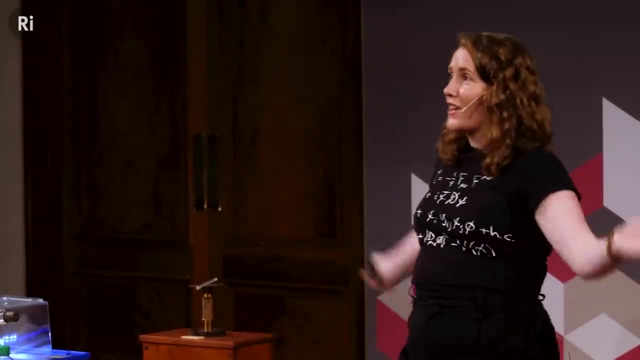 that the atom was mostly empty space, that light acts like a particle, that light a wave- in fact, all of matter acts like a particle in a wave, that we're living in a violent shower of high energy particles coming from space, and that the universe is far richer and more complex. 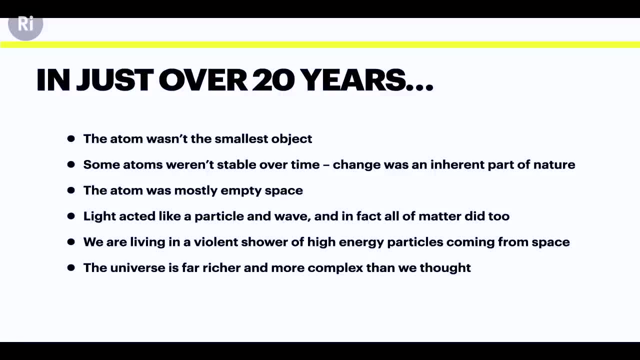 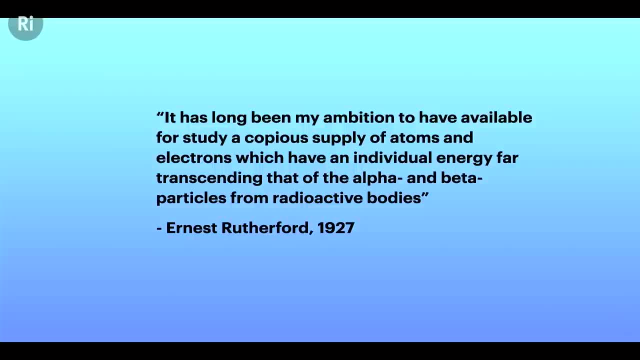 than we originally thought. So this was a huge change that happened at the start of the 20th century, But it actually continued. That trajectory continued massively because at the end of the 1920s Ernest Rutherford, who by then was the president of the Royal Society, 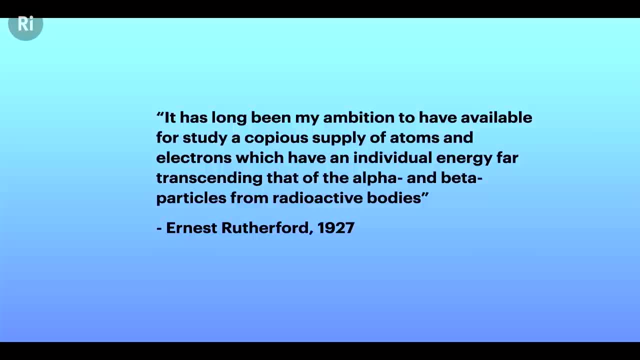 decided he needed to dig deeper into the atom because he still didn't understand what was at the heart of the atom. They knew that there was an atomic nucleus at that point in time, using another experiment called the gold foil experiment that some of you will have heard of. 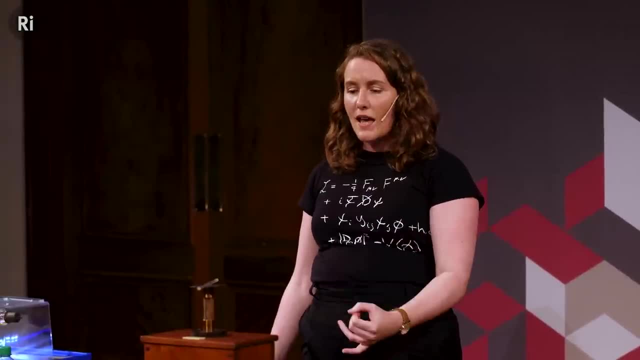 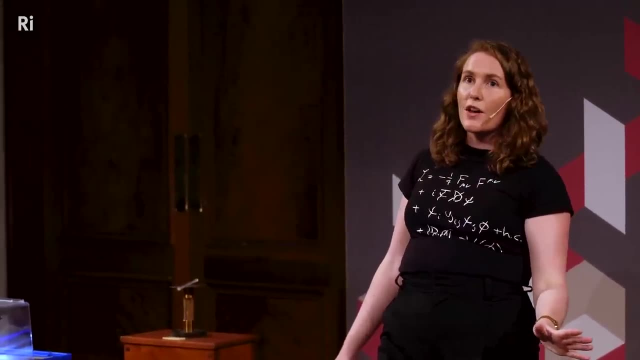 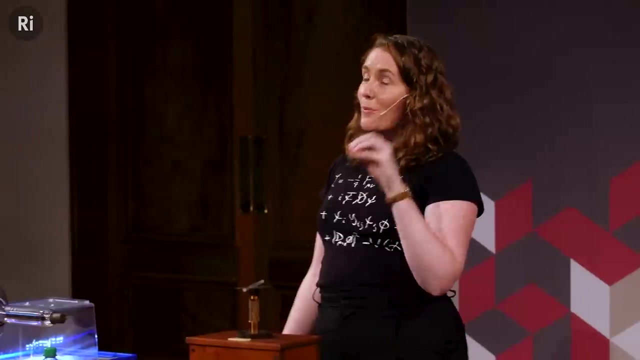 So he presented to the Royal Society this ambition that he wanted to have available for study a copious supply of atoms and electrons with an individual energy far transcending that of the alpha and beta particles from radioactive bodies. Now there's one way to get particles up to high energies. 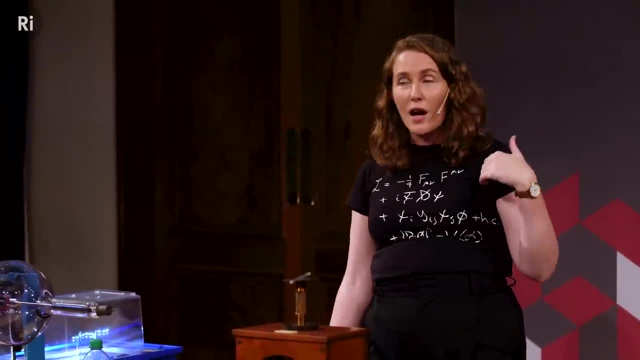 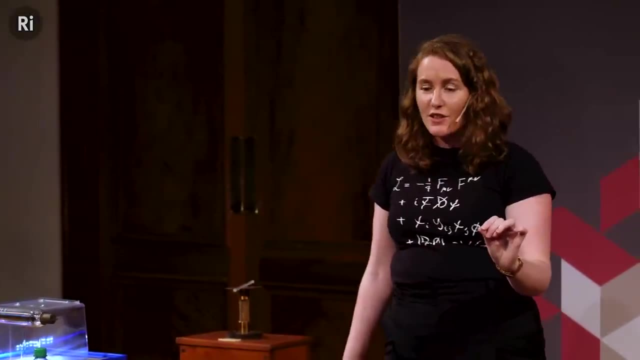 and it's what my field is. I work in particle accelerators and that is exactly what he was asking for, And to get a particle up to a high energy, you need a high voltage, And they calculated that the voltage they would need. 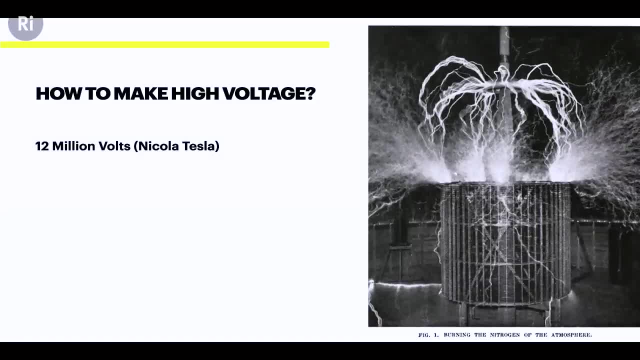 to split open the nucleus of an atom was about 10 million volts. Now, if you've walked under a pylon that transports our electricity at 300,000 volts, you'll realise how frightening 10 million volts was, And at the start of the 1920s. 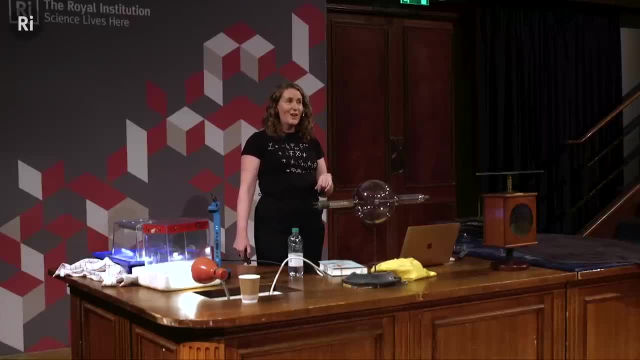 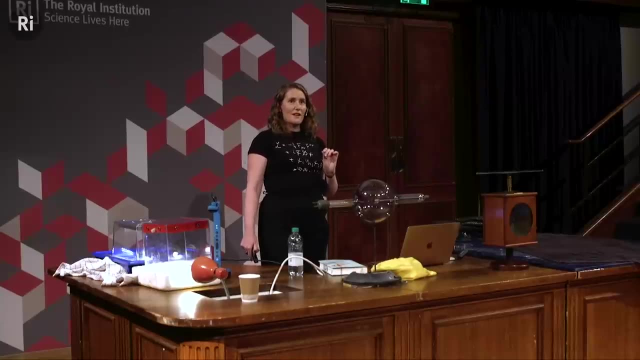 most homes didn't even have electricity, right? So, at this point in time, requesting 10 million volts for a physics experiment was pretty wild, right, And the only person, one of the only people working with those kinds of voltages was Nikola Tesla. 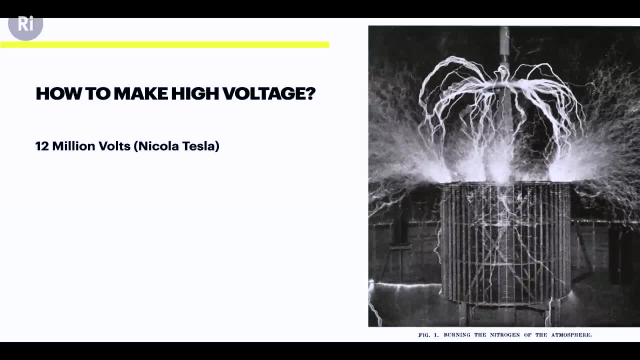 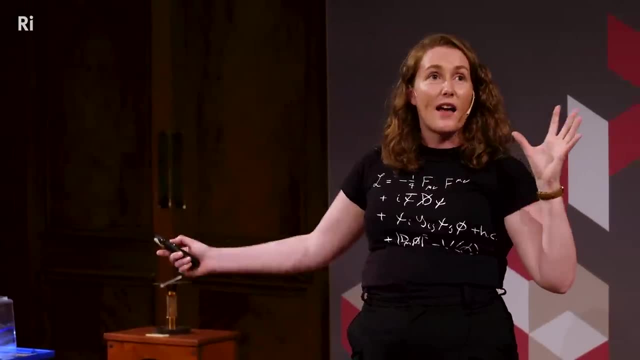 And this is what it looked like. I don't know about you, but I don't want to go in there and do a detailed experiment anywhere near that thing- And there were people all around the world using things like Tesla coils. In Germany they were trying to harness lightning. 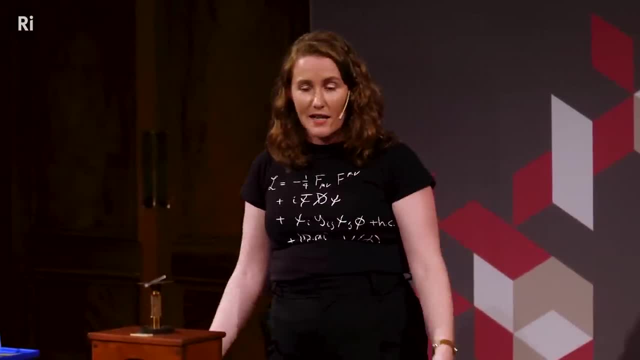 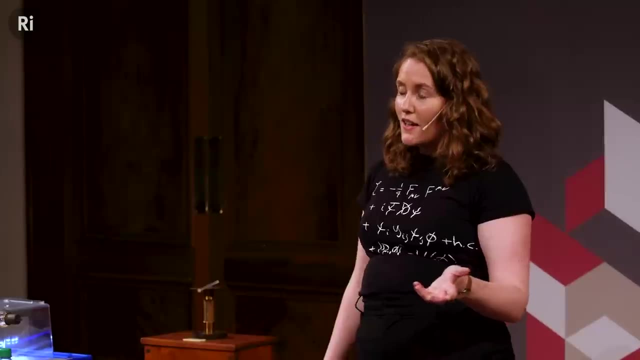 until one of the researchers fell down the ravine that they'd rigged up their experiment in and passed away so that that experiment didn't go any further. And other people were using things like transformers, And there was this race to develop the first machine. 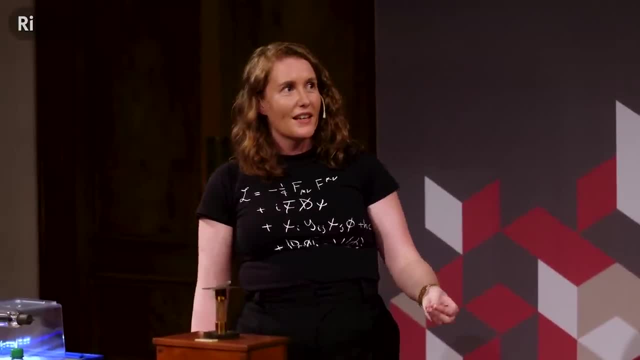 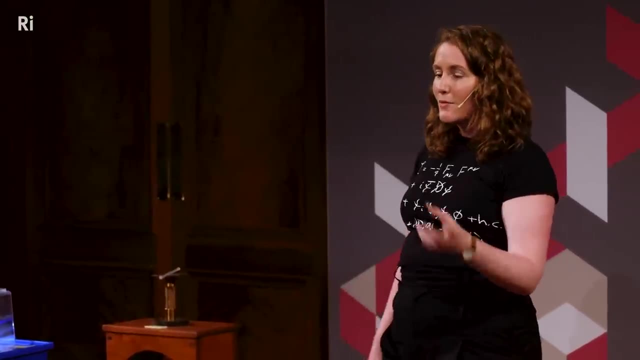 which could get up to a high enough energy to split the atom. And along the way, quantum mechanics changed the game. Because along the way there was a Russian researcher called George Gamow who came along to the Cavendish Laboratory, where Rutherford was working in Cambridge at that time. 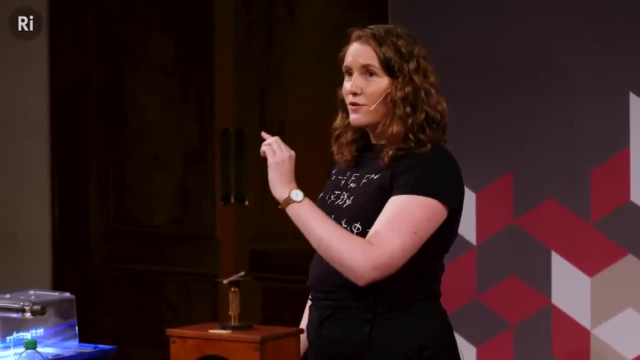 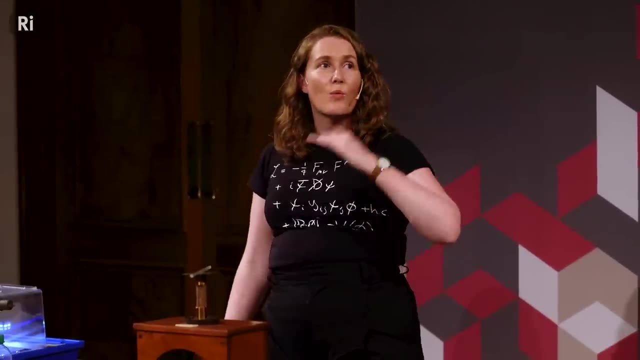 and worked with them, And together they understood that they might not need 10 million volts, They might be able to do it with just a million volts or even lower, And at this time they were well along the way of developing their first particle accelerator. 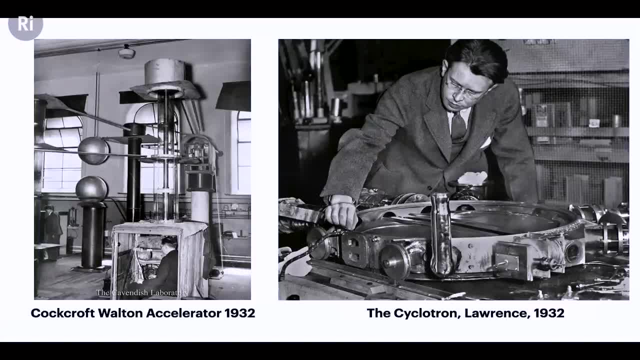 which is the one on the left here, by two main researchers called John Cockcroft and Ernest Walton, And Walton, who was the student, by the way, did most of the actual building and most of the actual work which, for some of my graduate students in the audience. 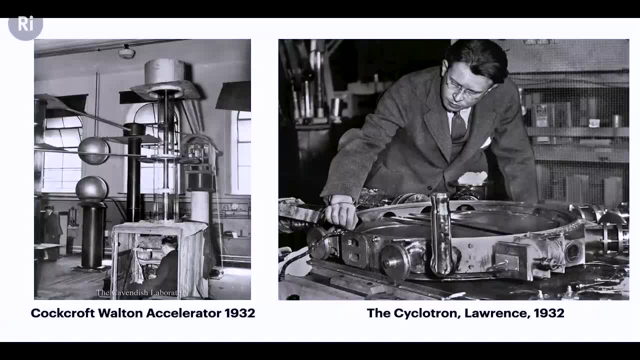 they'll feel a resonance with that experience. And at the same time in the US Ernest Orlando Lawrence was coming up with a different idea for a particle accelerator called a cyclotron. But actually, these guys in Cambridge, they won the race And they split the atom for the first time. 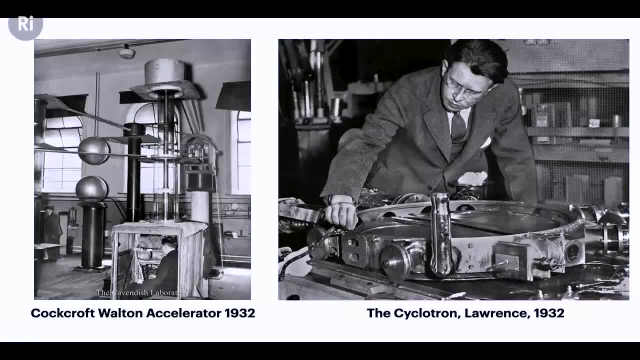 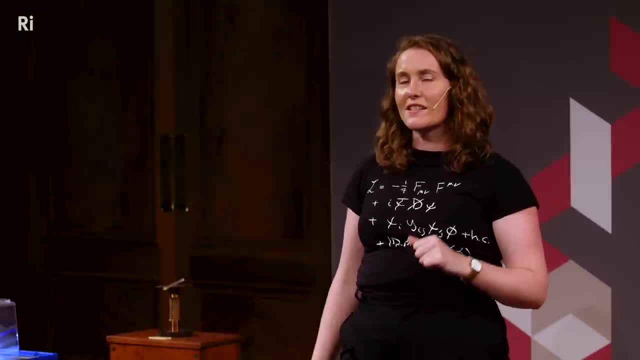 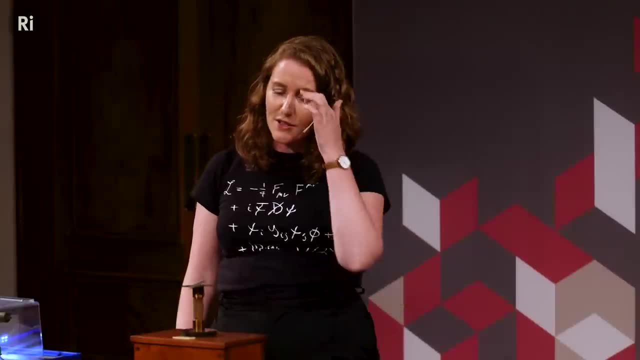 in April 1932, using what is effectively a series of transformers, And I want to point out to you how they did the experiment Because, again, when I learnt about this, it was quite incredible to find out the reality of what experimental life was like in 1932.. 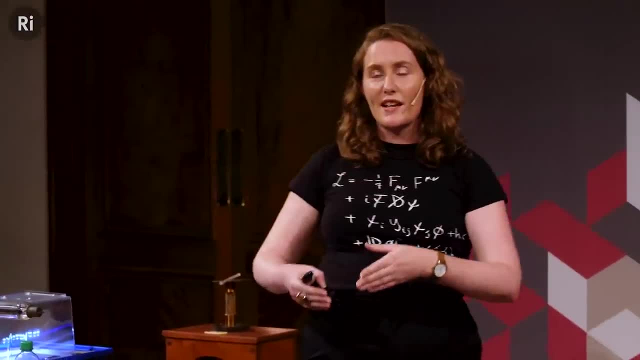 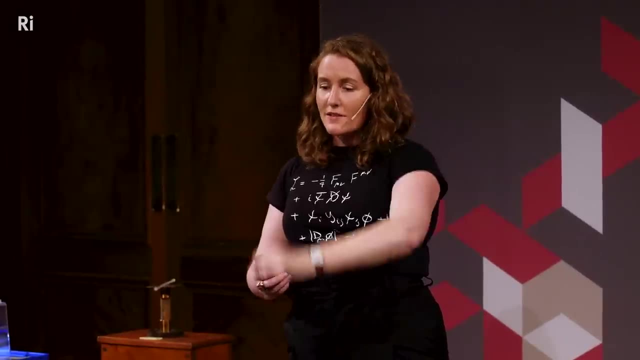 So you can see underneath the vertical tube, which is actually the accelerator, where protons start at the top and they travel down and they go through a voltage in the middle and then they travel down to the bottom where they're meant to hit a target of usually lithium or something like this. 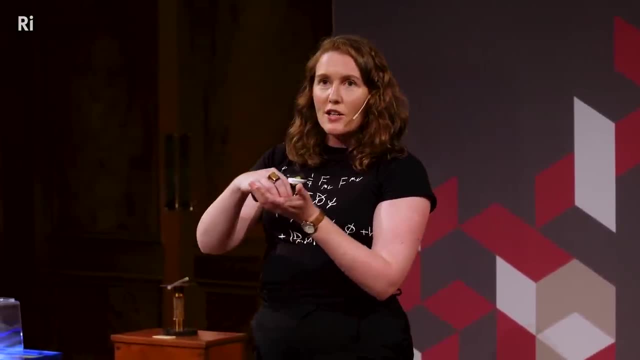 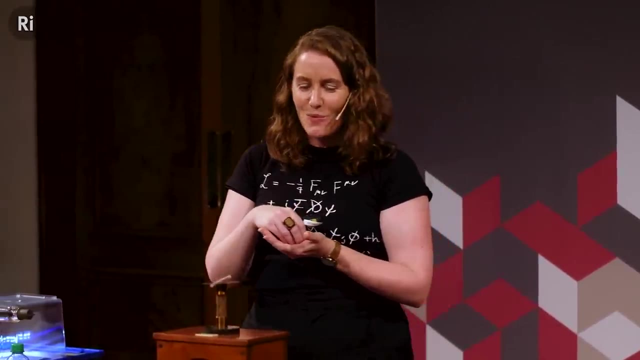 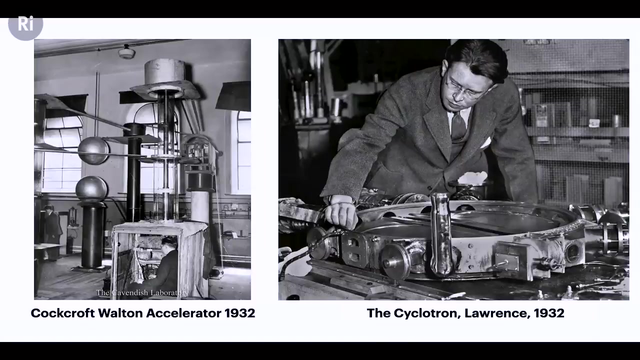 to study whether or not it split the nucleus. And underneath there you can see a detector, otherwise known as a human watching a scintillating screen very similar to the one that Röntgen would have used back in 1896 in his lab to discover X-rays. 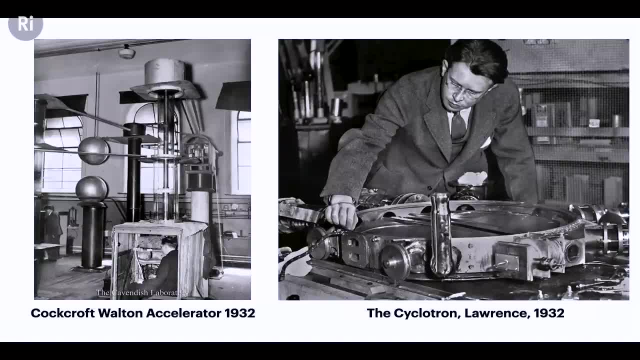 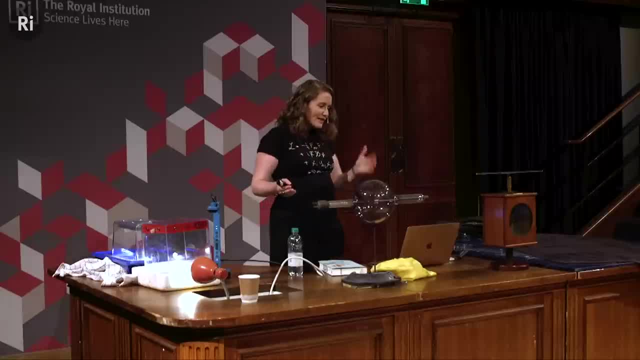 And so one morning, after much trial and things breaking and things not working and them rebuilding the entire machine in a different room- this is four years later, something like that. Walton is alone one morning. He's a student right, So he's warming up the machine. 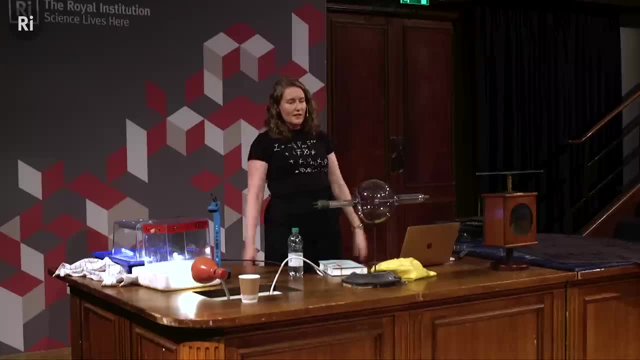 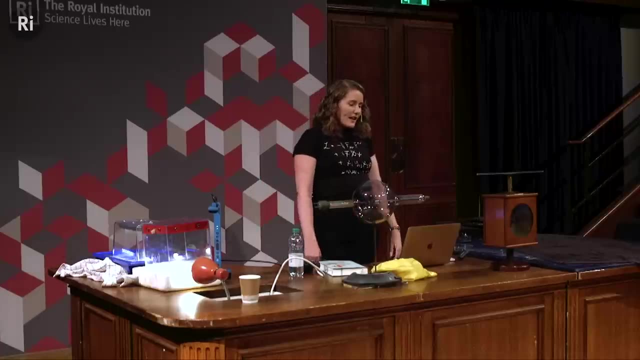 He's at his control desk And the thing gets up to a couple of hundred thousand volts And it seemed pretty stable And Cockcroft was away doing something else because he had a million jobs And Walton thought: OK, well, I'll dial up the machine. 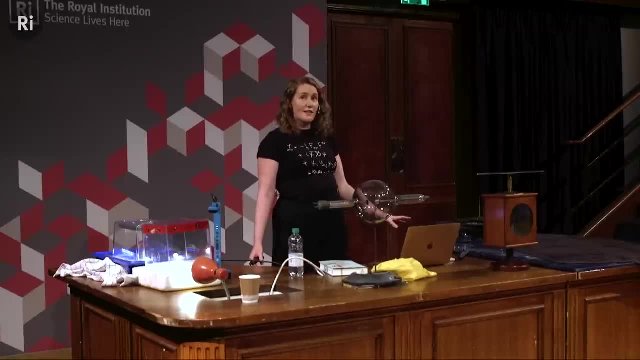 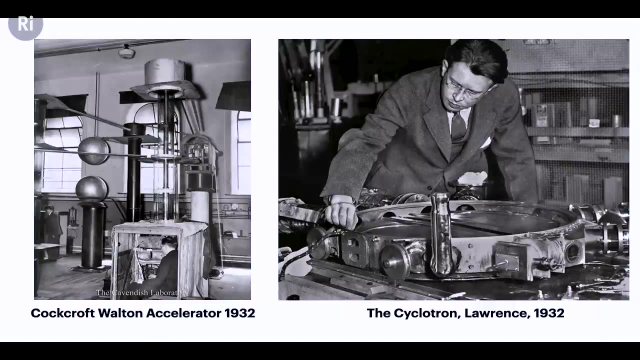 and I'll pop a target in and I'll turn it on and I'll just see if anything's happening. And so he steps away from his control desk and he crawls across the floor. Now there's hundreds of thousands of volts in this room, right? 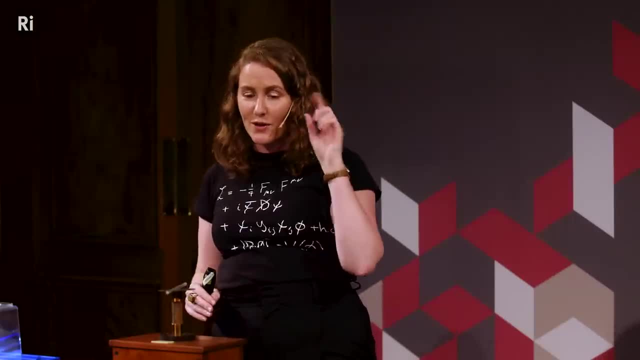 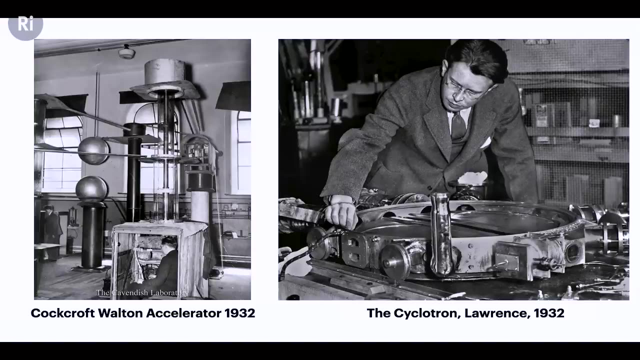 He crawls across the floor and into this little box that he's sitting in in this photograph And he pulls the curtain past him and he sees on the screen flashes, more flashes than he ever thought possible. The screen was lighting up with flashes. 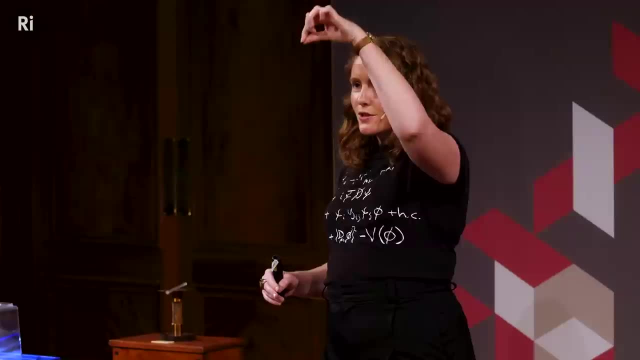 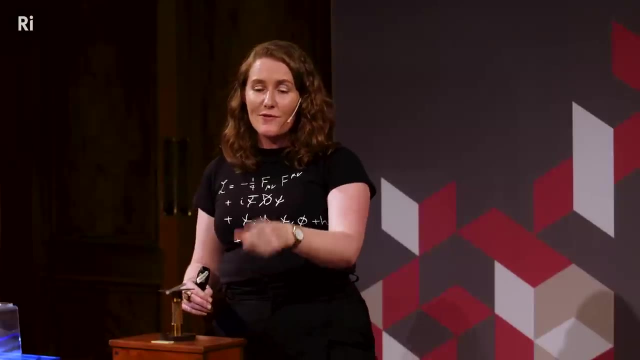 And what that meant was that the protons coming down were hitting lithium and it was splitting apart into alpha particles, And even though he hadn't trained for very long, he could recognise an alpha particle in this box, And so for the first time he was. 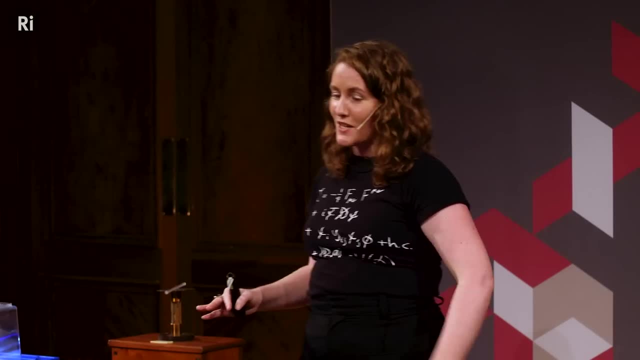 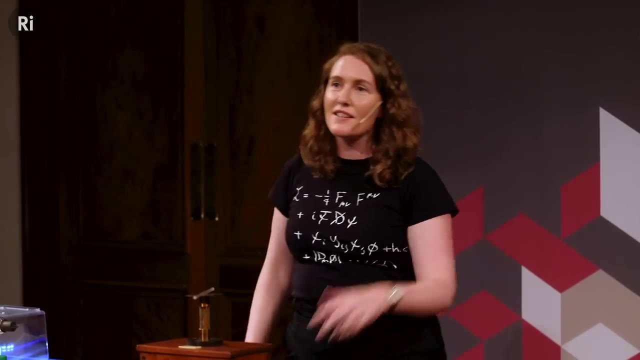 oh, my goodness, what am I seeing? He knew he was seeing something special. He called in Ernest Rutherford and John Cockcroft and others And, Rutherford being the tall guy that he was, he climbs into this box with, like, his knees up around his ears. 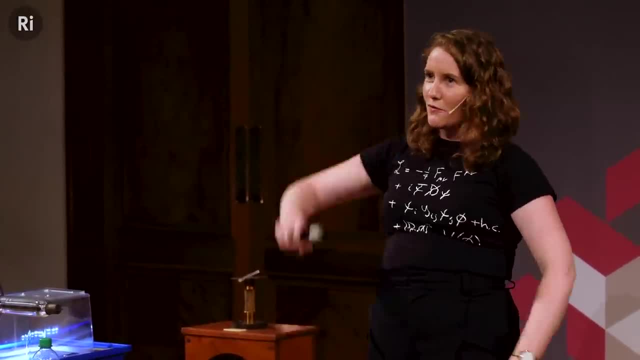 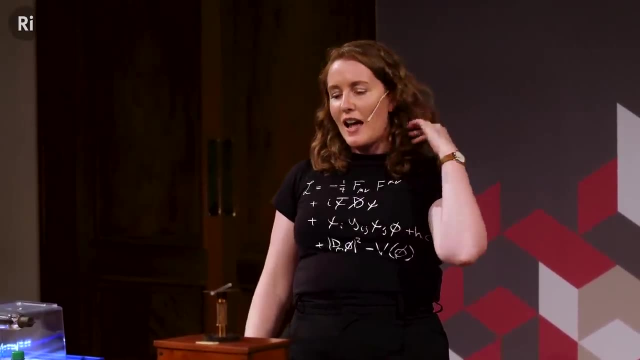 And he watches the screen and he's like those are alpha particles. I should know I was there when they were invented. He basically found them for the first time earlier in his career And so for about a week as they did more experiments and wrote it up. 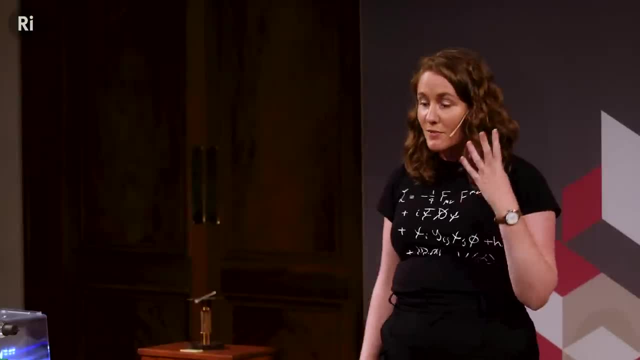 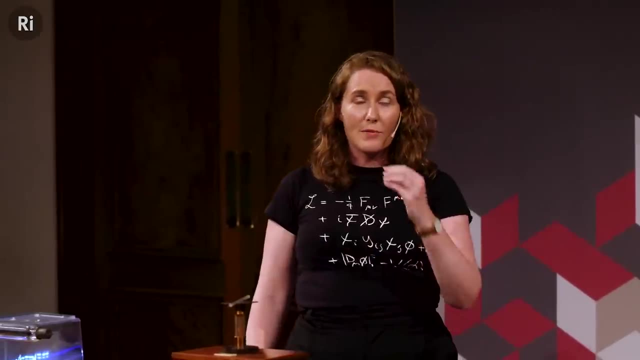 there were only about four people in the world that knew that the atom had been split, And this led to incredible advances, some of which I'll tell you later about the applications of machines like this, of particle accelerators, And some of those applications also happened with Ernest Lawrence. 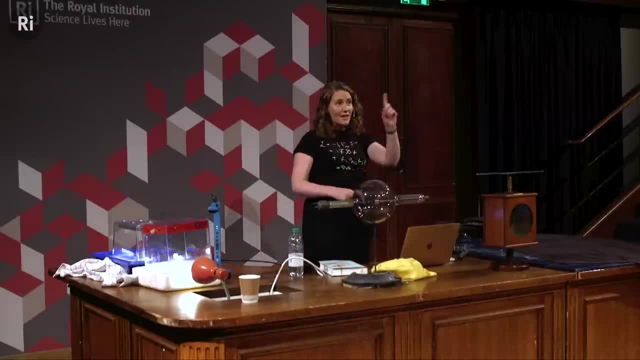 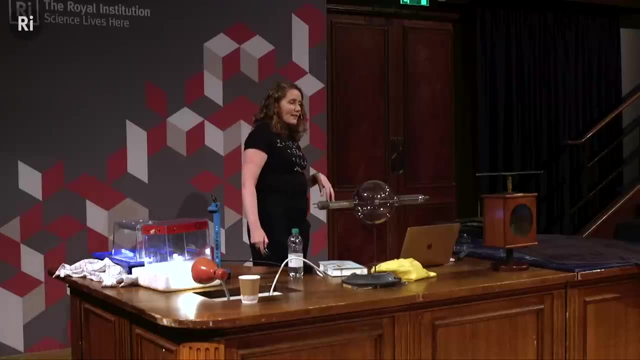 with this other machine, which was circular, which overcame this sort of 10 million volt crazy voltage requirement by reusing a voltage again and again. But despite that, as they worked harder and harder, the machines got larger and larger and larger. 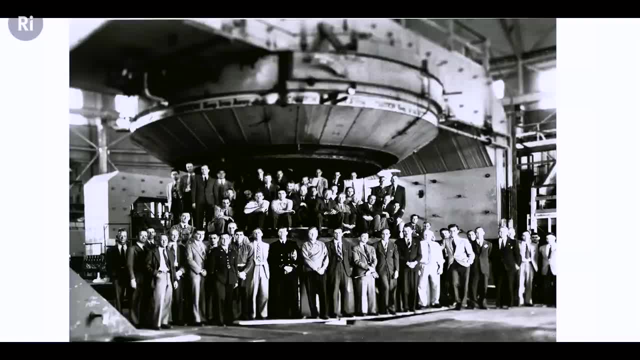 And there were more and more discoveries coming from cosmic rays, But at this point in time particle accelerators were still not really used for anything other than some detailed nuclear physics studies. They hadn't discovered any new particles using an accelerator. And then World War II broke out. 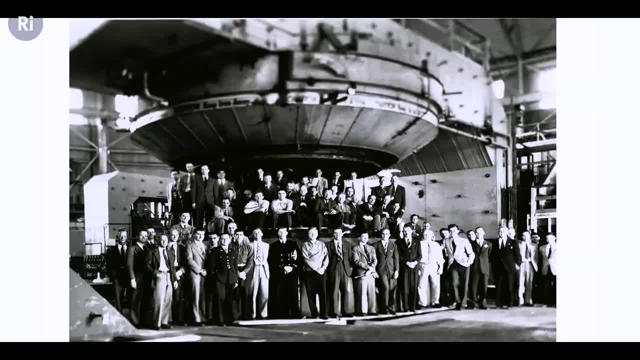 So we get to this point, we get to these big labs. They've started to generate new types of radioactive elements that they could use in medicine, which Ernest Lawrence did with his brother. Everything was sort of going wonderfully, And then the world changes entirely, right? 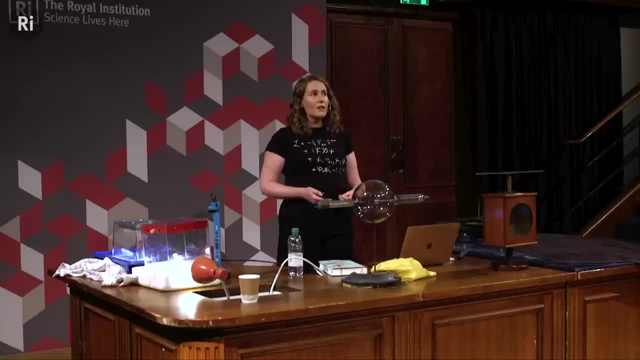 And most of the physicists that I've talked about were involved- especially the US-based ones were involved in the war effort in some way. Many of them were involved in the Manhattan Project And one of the people who was asked to join the Manhattan Project. 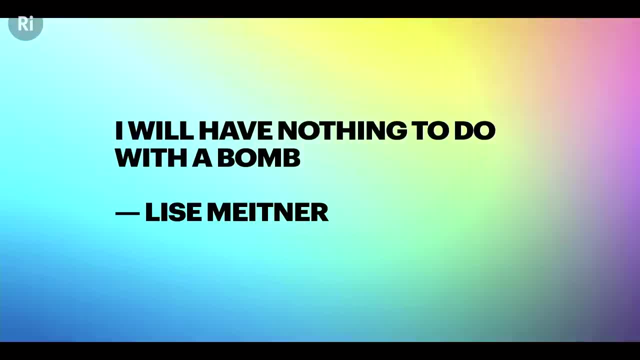 but refused was a woman named Lisa Meitner who, again, you might not have heard of her, but she did some foundational work in understanding nuclear fission. But her name was left off the key paper because she was Jewish and so she had to flee. 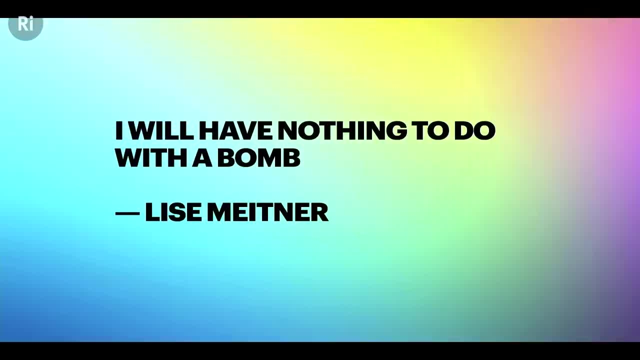 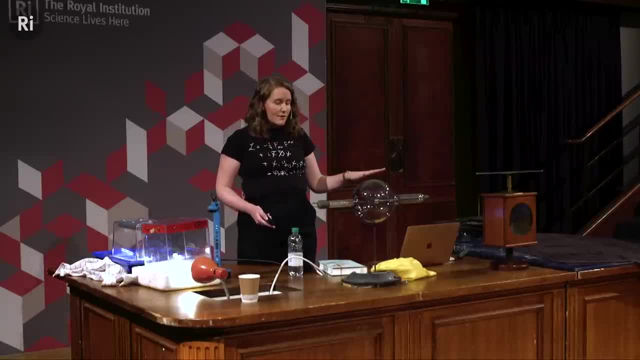 and so her collaborator could not admit that he was working with her, And she refused to join the Manhattan Project. She refused to have anything to do with a bomb. And well, we know what came after that, and we know what physics was capable of. 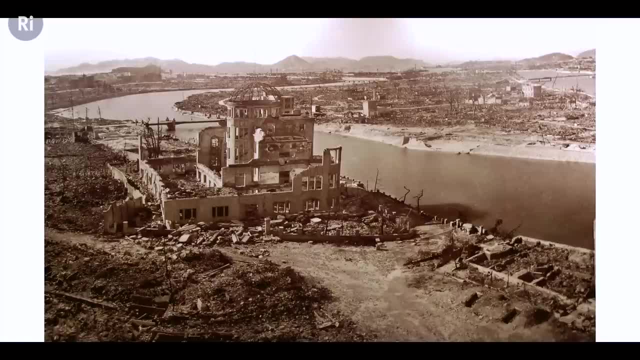 when there was large amounts of resource, and putting all of these people together in one or a number of places with a mission to do something that they did not even know was possible at the time, And I should say many of the physicists who worked on the Atomic Weapons Project. 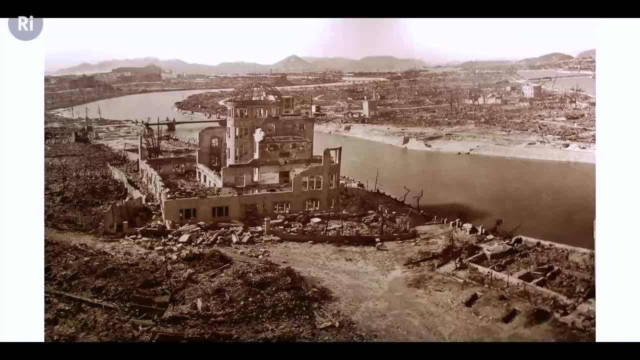 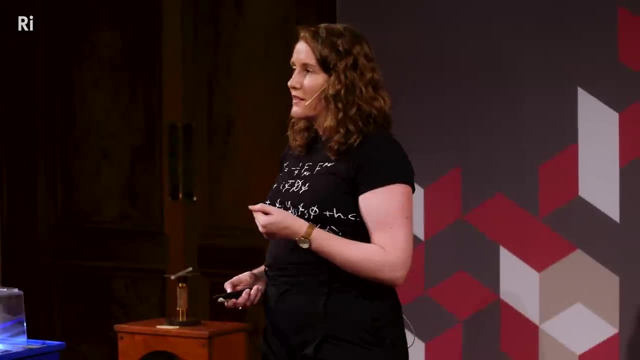 didn't even know really what they were trying to achieve, let alone did they think it was possible. And this changed the world, Obviously, But it dramatically changed how physicists approached what they did. They realised that physics was political right. This was no longer just a search to understand nature. 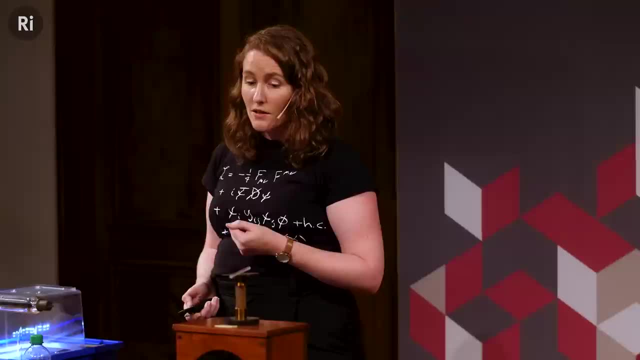 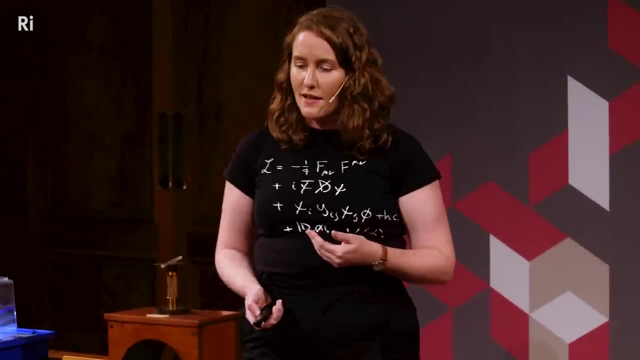 that what they were finding could dramatically change the world for better or for worse, And there's some stories in the book about how that changed the views of some of the physicists, and they're becoming much more pacifistic after the war actually. 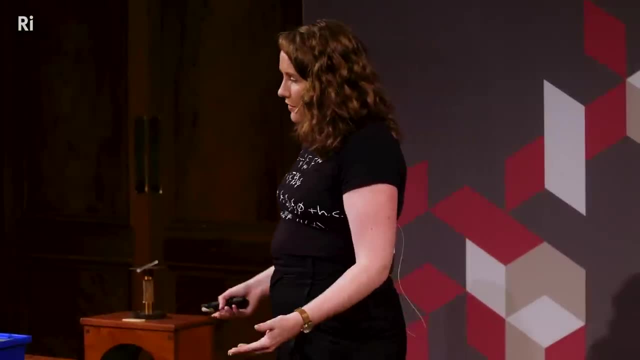 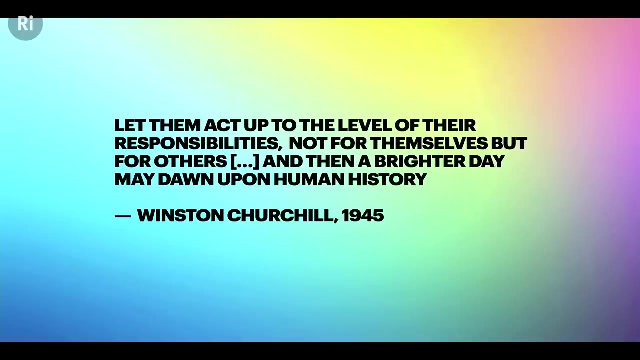 And so, with this knowledge that the US now had, especially, even Winston Churchill was sort of saying: well, the US now is at the forefront of this knowledge. Let them act up to their level of responsibilities, not for themselves, but for others. 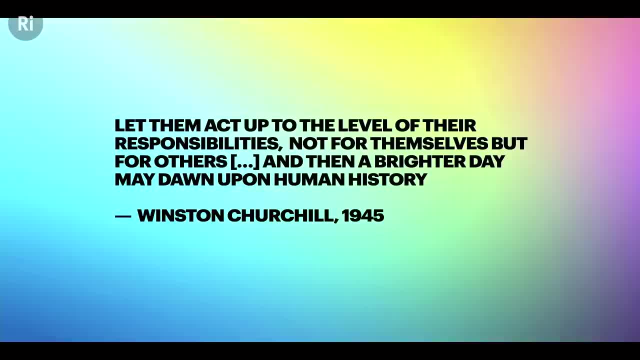 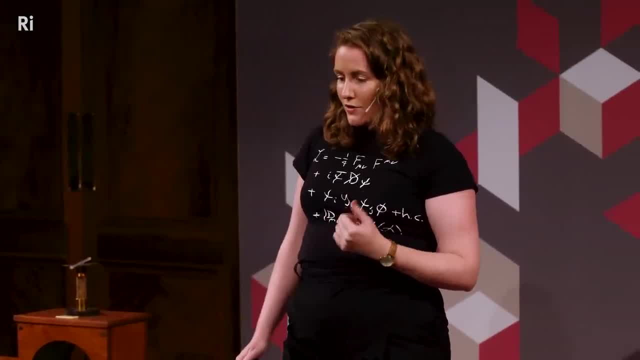 and then a brighter day may dawn upon human history. This is a dark period in the history of physics, so I wish I could allocate more time here. I can't. But it changed the approach entirely. But what did come of it was our understanding that if you put together 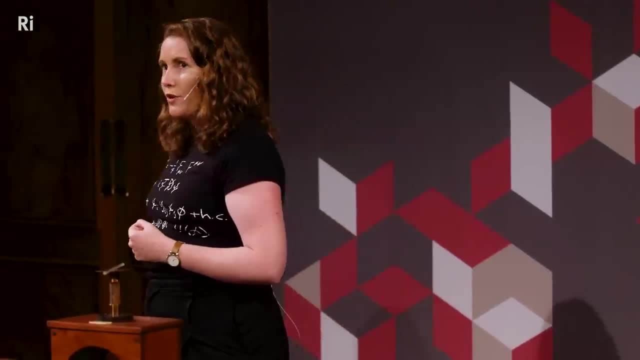 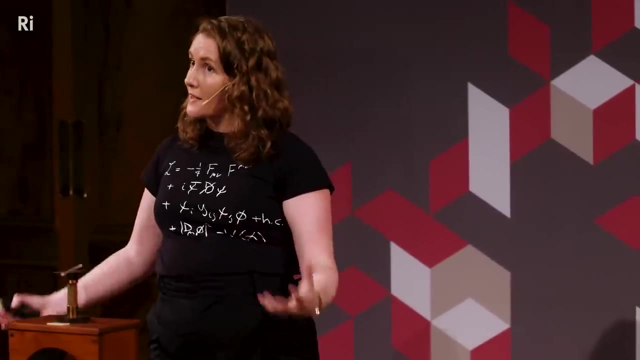 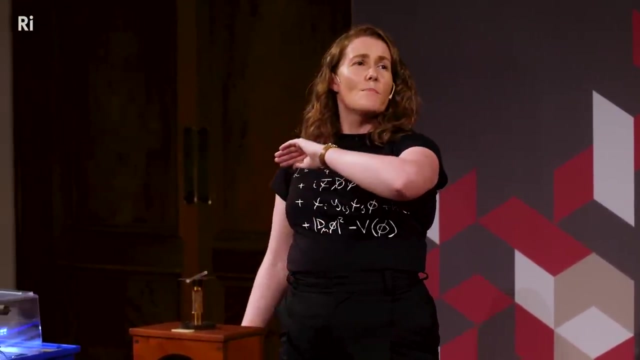 large amounts of smart people and give them a very difficult problem to solve, that they can solve it. And so after World War II we get the emergence of big science, big scientific projects, big scientific laboratories, especially in the US, And that led to discoveries of many new types of particles. 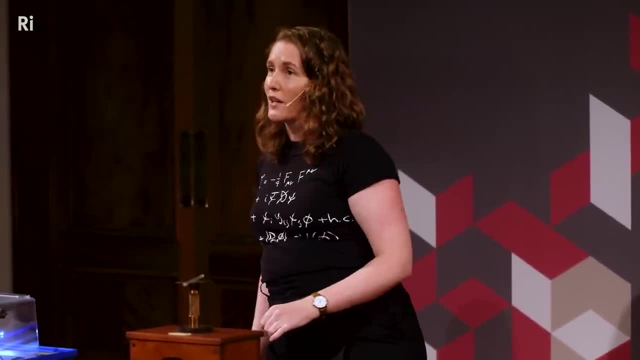 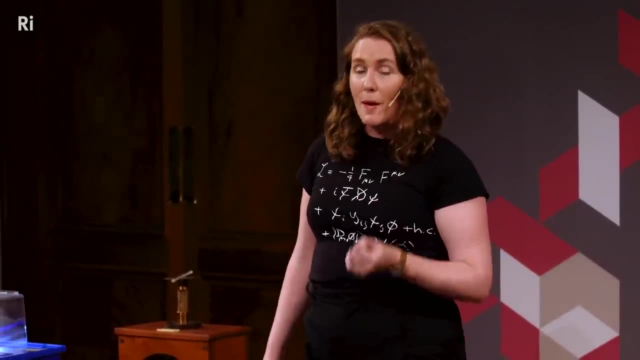 At one point there were about 200 different types of particles that they were struggling to classify and understand how they were fundamental. It wasn't just the weapons that came out of World War II either. One of the other big inventions that came out was radar. 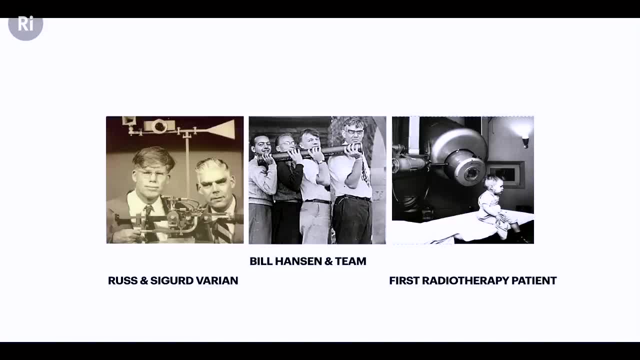 And I don't have time to tell this entire story. but we start with a couple of people trying to invent radar. We get someone who's trying to invent particle accelerators who teaches them how to do it. Yay, we have radar. 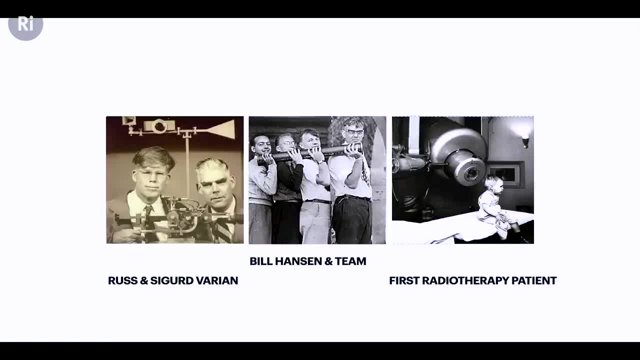 But as a result of this, these two brothers, Russ and Sigurd Varian, team up with Bill Hansen, the accelerator person, and they invent very compact particle accelerators that can then be used for cancer treatment, And so it seems a completely roundabout story. 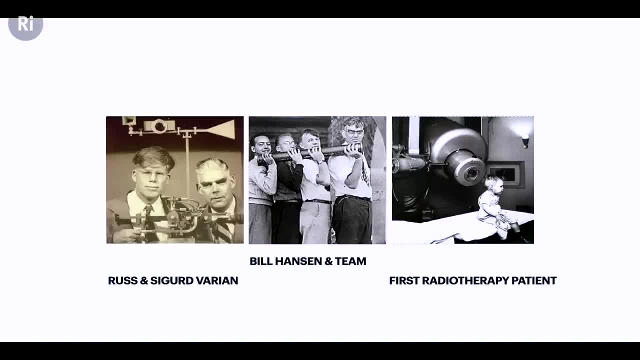 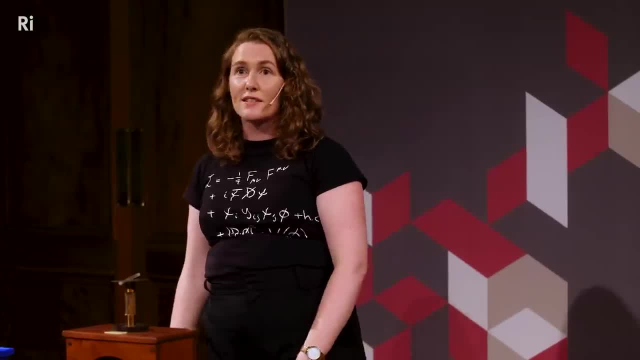 but the whole story is in the book And actually their company, Varian & Co, was the first publicly floated company in Silicon Valley, predating what we would now call Silicon Valley actually, But this activity towards particle accelerators and radar in that area. 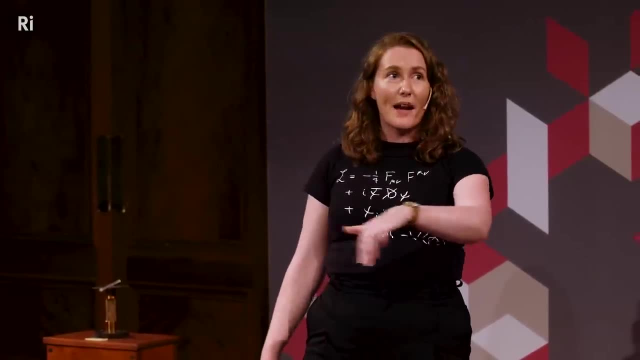 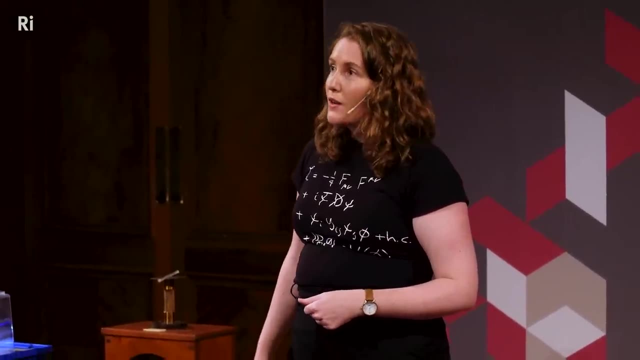 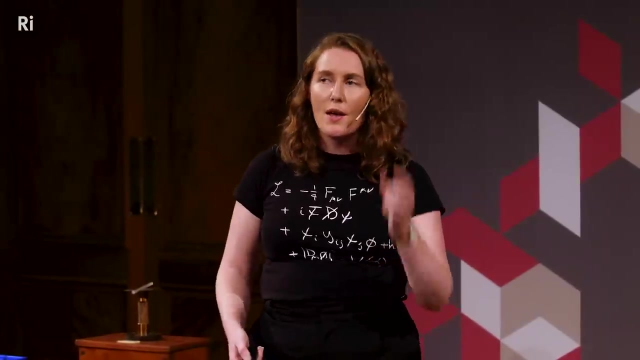 seeded the high technology background and the concentration of highly technical people that would then become Silicon Valley later down the line. And now these machines, these particle accelerators, are used in many different parts of the world for many different applications, But the one you'll probably come across- 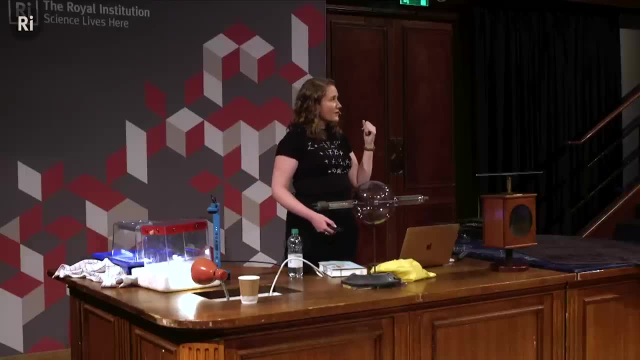 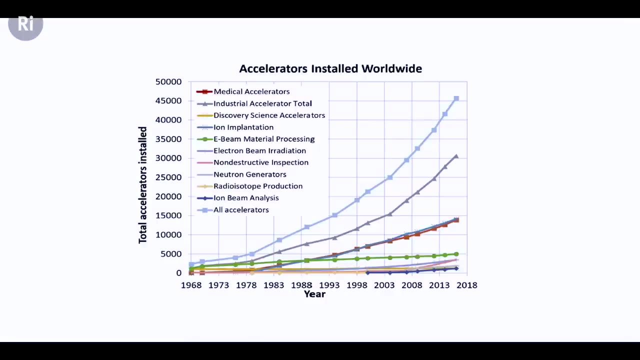 if you ever come across an accelerator is in a hospital for cancer treatment using radiotherapy, And so the growth in the applications of these machines over time is just phenomenal: Everything from the lithography that creates the chips in your smartphones to materials processing to create shrink wrap. 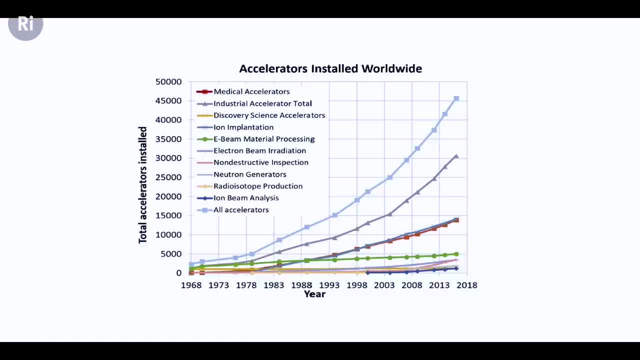 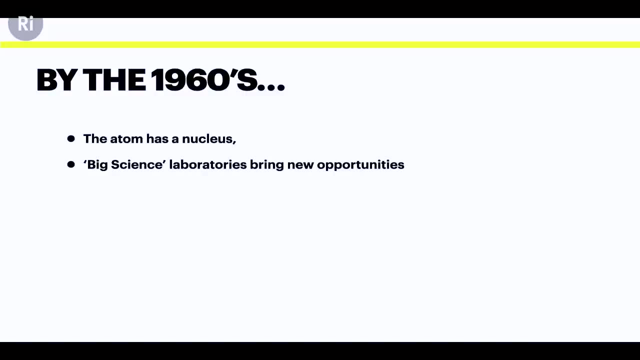 to treating cancer, to understanding the origins of the universe. It is really quite phenomenal. So by the 60s, even we know that the atom has a nucleus, that these big science laboratories are bringing new opportunities, that we can now create isotopes with many uses. 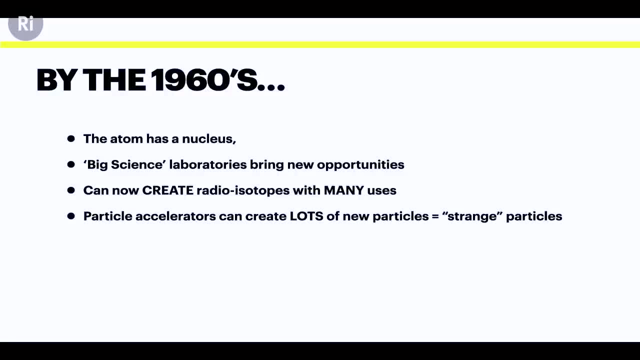 including traces for medical imaging- that these new particle accelerators can create lots of new, different particles that play no role in ordinary matter, And we get these particles called strange particles. that acted in very confusing ways And slowly but surely people started to piece together. 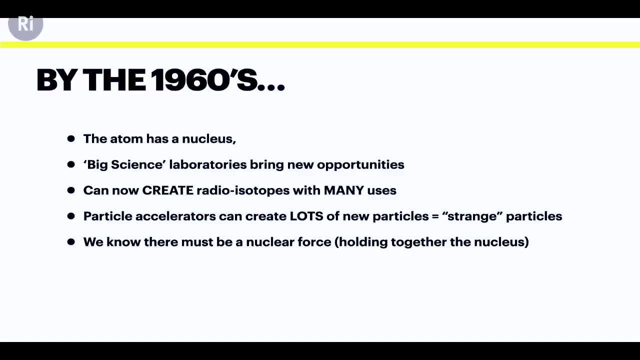 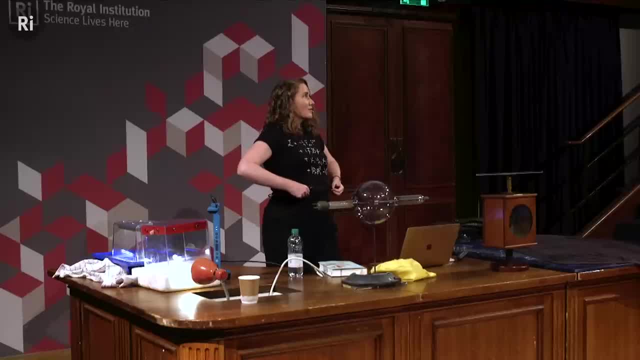 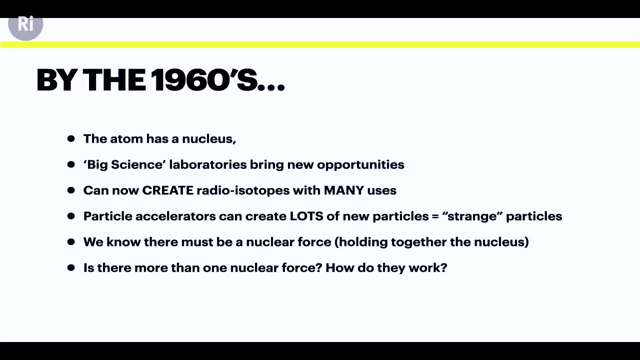 the different particles and forces in the universe through this kind of experiment to generate what we now call the standard model of particle physics, which is so elegant that you can write it on a t-shirt. And of course there were many questions that came along about those nuclear forces. 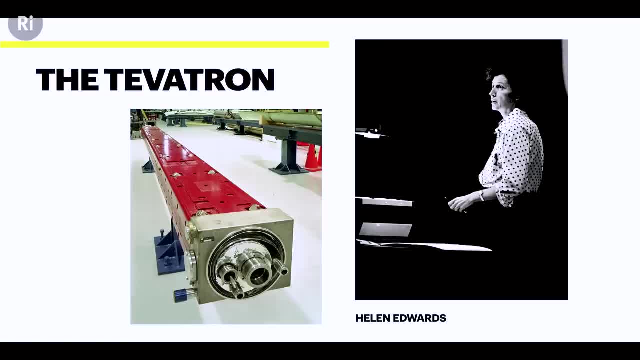 and how they worked. And I just want to highlight one other person- And, if I have time, do one more quick demo- who is part of this story And her name is Helen Edwards. So by the 1970s, 1980s, 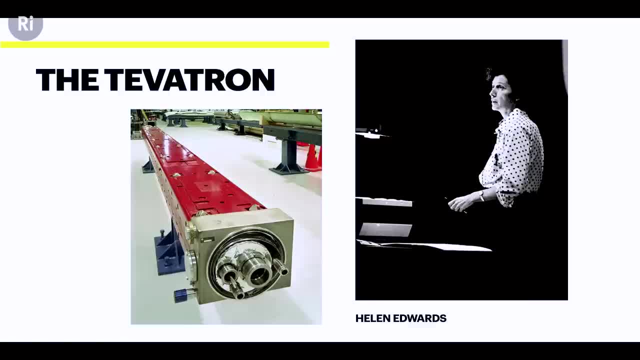 of course women are accepted into physics. They're still not as prevalent as men. But this woman, Helen Edwards, is a remarkable accelerator physicist. She works in my field. She worked in my field. She passed away a few years ago. 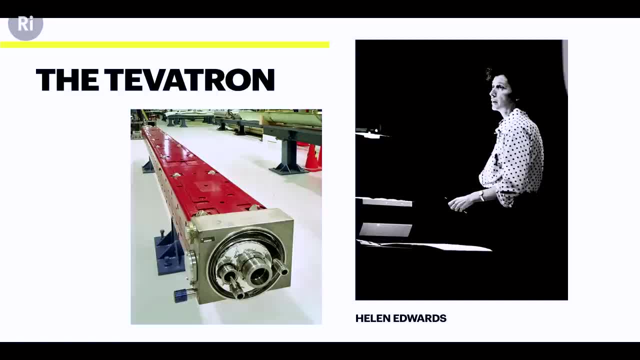 And she was the mastermind behind the biggest accelerator before the Large Hadron Collider, which was called the Tevatron, And what she needed to mastermind was the first superconducting accelerator which we needed, because we needed accelerators to reach higher and higher energy. 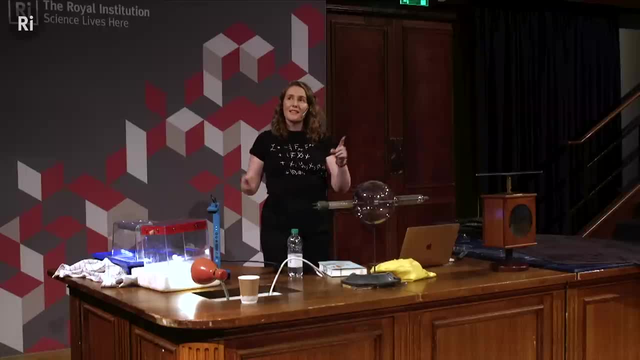 without becoming infinitely large. So to have stronger magnets they had to use an entirely new technology which had to work at liquid helium temperatures in order to produce very strong magnetic fields to confine the particles. And she's someone who sort of oversaw. 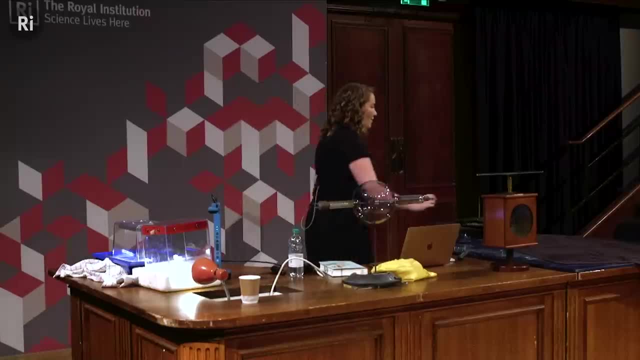 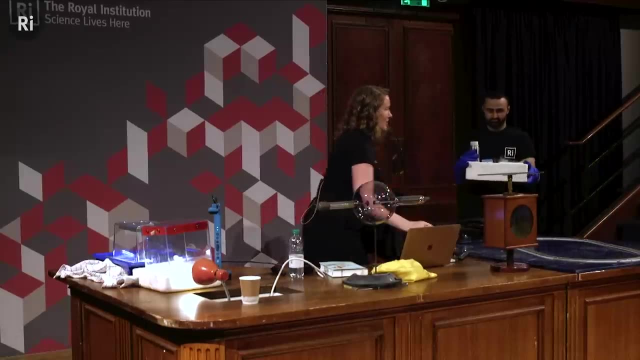 this whole process. So very quickly, if we have time, Tom Tom has been hopefully cooling down a little piece of superconductor which is almost like a ceramic material. It's called yttrium barium copper oxide. 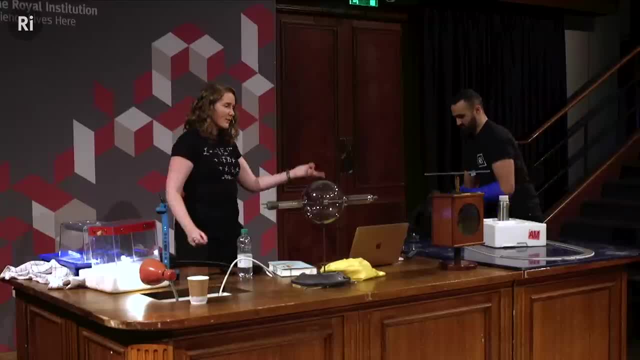 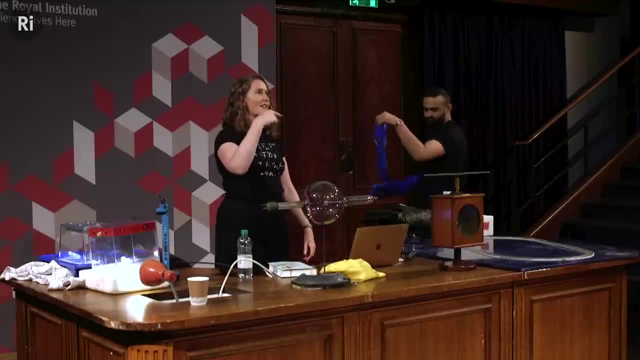 the one we have here today. This one works at liquid nitrogen instead of liquid helium temperatures. The key thing with a superconductor: it's in the name. normal conductors have electrical resistance so they heat up if you try and put a very strong electric current through them. 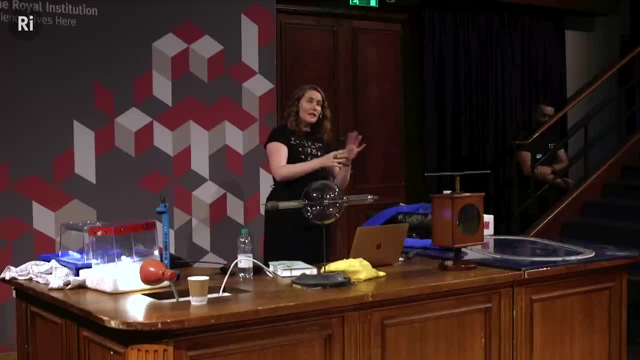 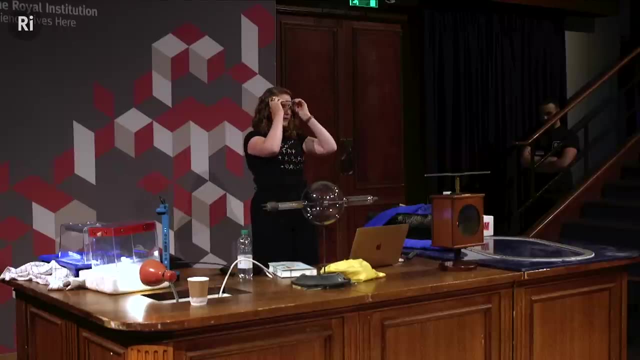 But a superconductor does not. It can be in a state when it's very cold, where it will actually keep electrical currents flowing without pumping in more electricity, And this is both a trick to reaching very high magnetic fields, but it's also the trick. 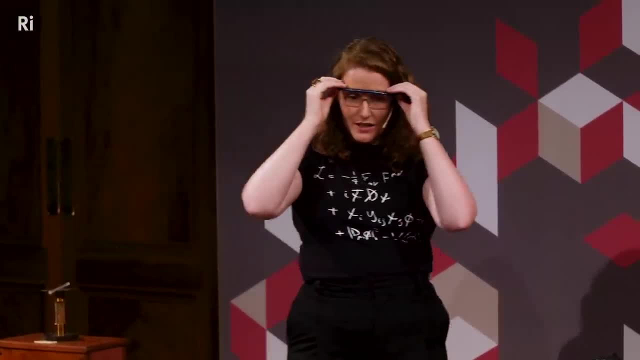 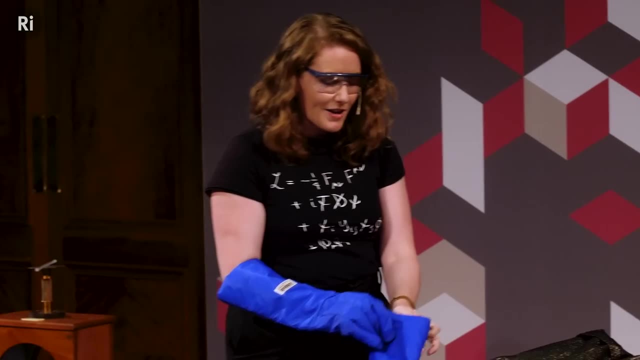 to reducing the energy consumption of these very large particle accelerators, where otherwise the losses would mean. well, I mean, the electricity bills are high enough, right, And when this machine was invented, that was actually a very important thing. So I'm going to get out. 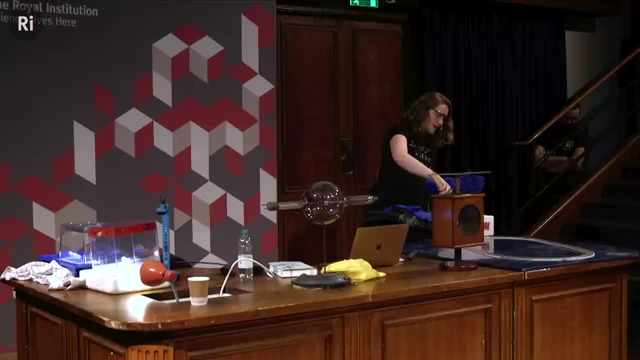 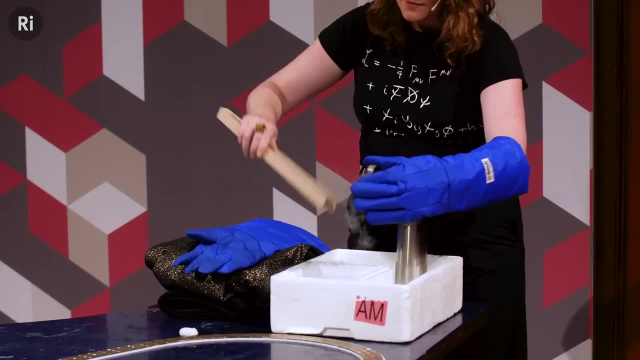 a piece of this superconductor. We've been sitting in liquid nitrogen here. It's been bubbling away And it also. this superconductor also has sort of some slightly strange effects which hopefully I'll be able to show you. 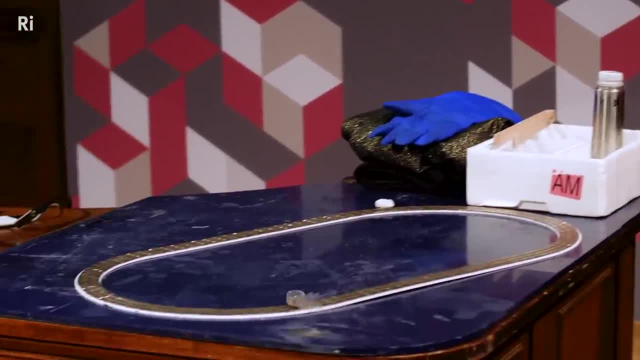 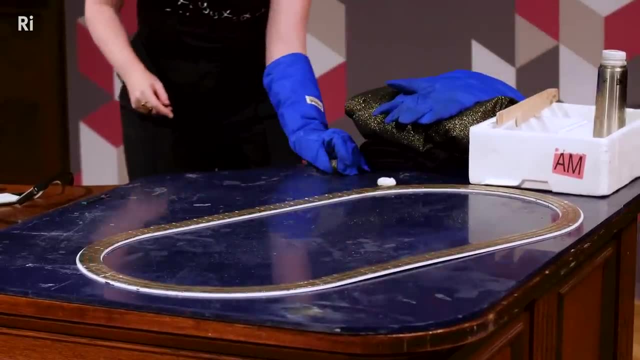 Put it on there. There we go. So because of this weird thing where they can have currents run through them infinitely, if you put them near a magnetic field like this, it creates its own field to push back against the magnets that are on this track. 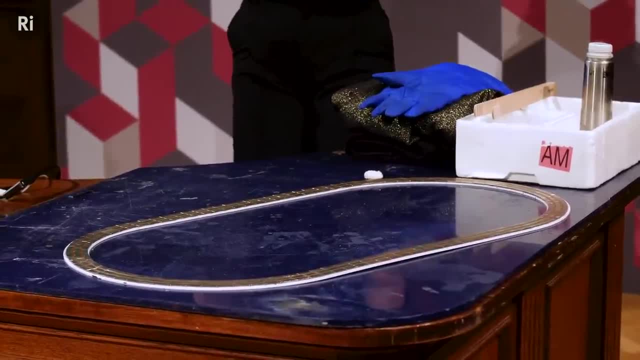 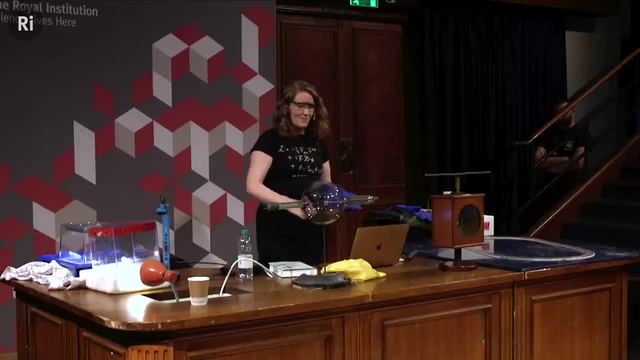 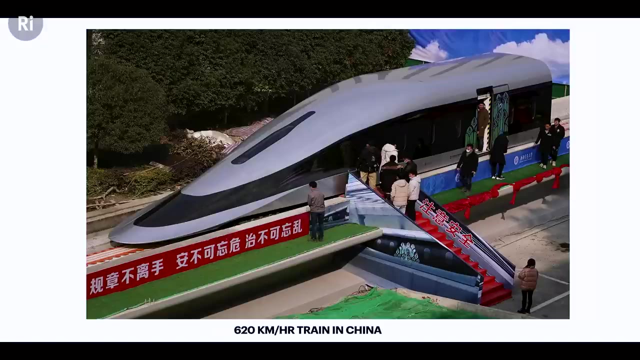 And sort of traps the magnetic field inside in an opposing way to the one I've put it in, And that means it can actually float above the track here, And this, by the way, is something which is really used: Superconductors levitating above tracks. 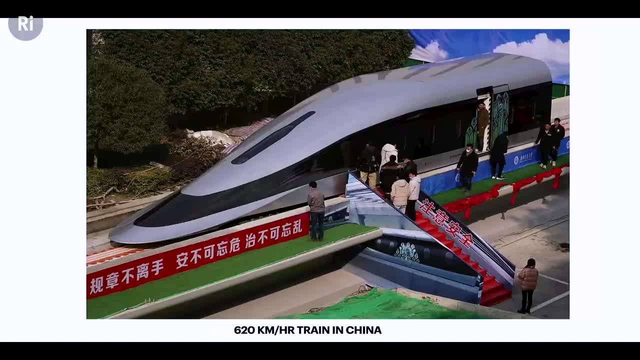 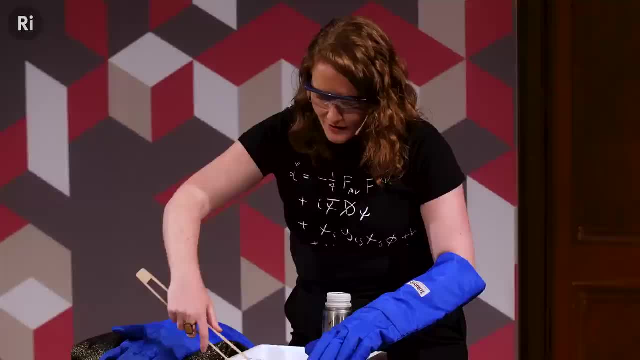 is really a technique which is used for incredibly fast trains because, of course, there's no friction involved. We've got here which Tom has prepared, a little version, which is not a train but it's a boat. I'm going to see if I can. 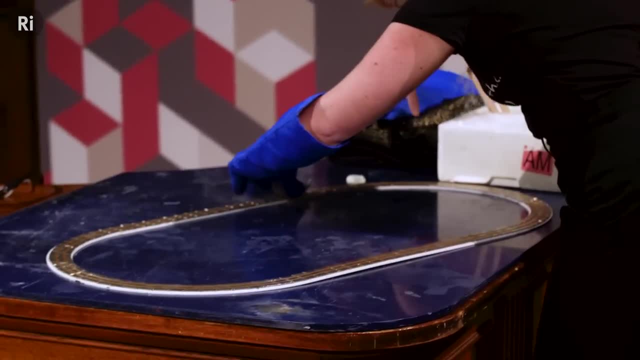 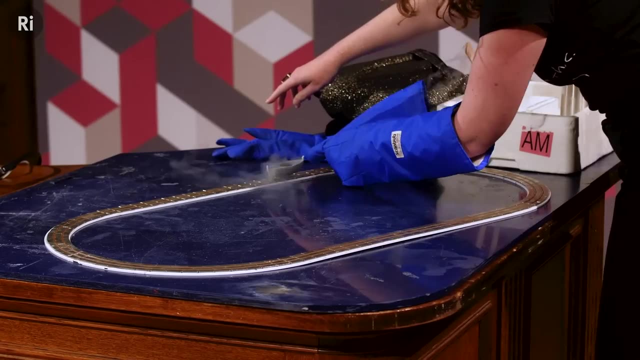 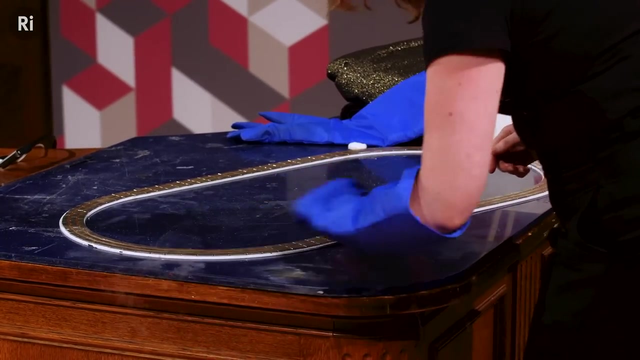 Isn't it sweet. I'm going to see if I can get that one working. Oop, There we go. Hey, Oh, Flipped over. Presumably the trains in China do not do such things. Let's see if I can just get it there a bit more stably. 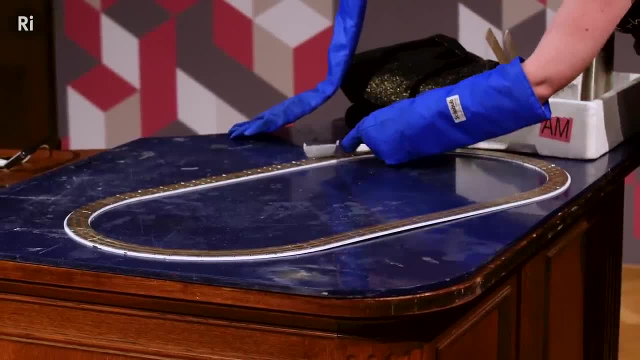 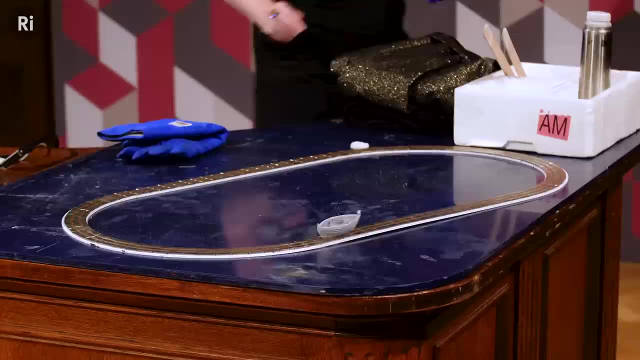 Oop, Of course, friction. There we go. Something on the tracks Leaves on the tracks. People watching me in Australia will have no idea what I'm talking about, but everyone in the UK knows All right, So OK. 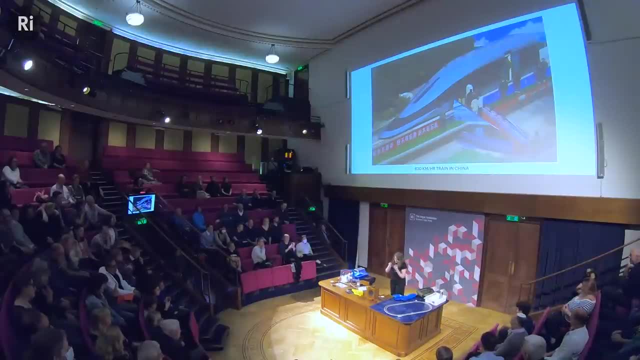 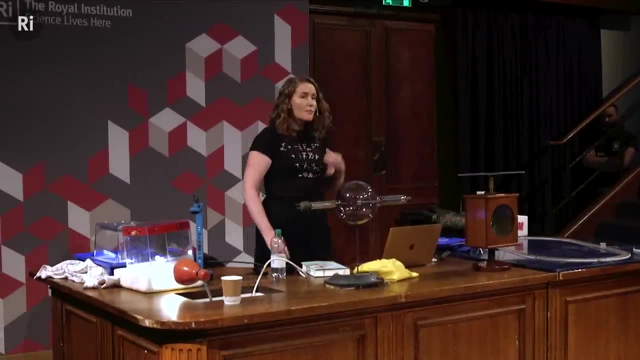 But the point with the Tevatron as the superconductor was that, in order to create this enormous particle collider, they actually had to commercialise this wire technology, And the commercialisation of that that happened through the Tevatron project is the reason why we can now use superconductors. 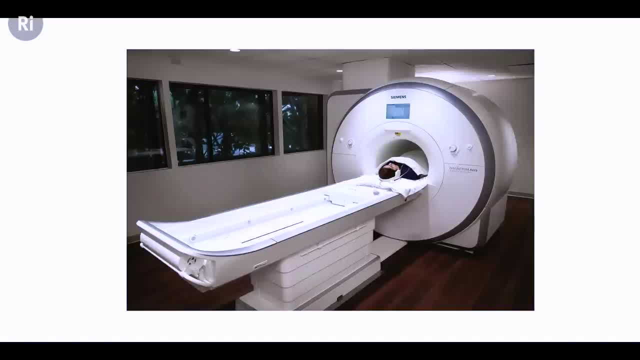 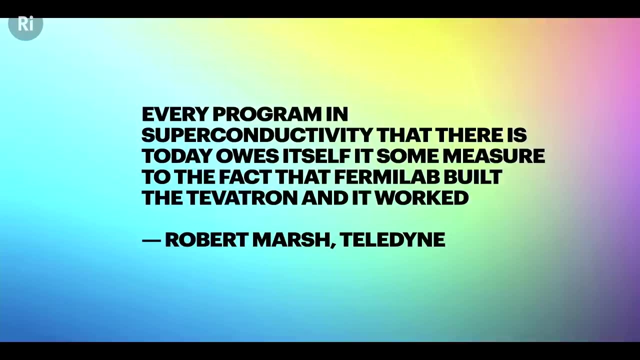 Superconducting magnets in other applications, including trains, MRI scanners- which is a huge one and potentially infusion reactors in the future, And the biggest manufacturer of superconducting wire and magnets in the world- Teledyne their CTO- I think it is Robert Marsh. 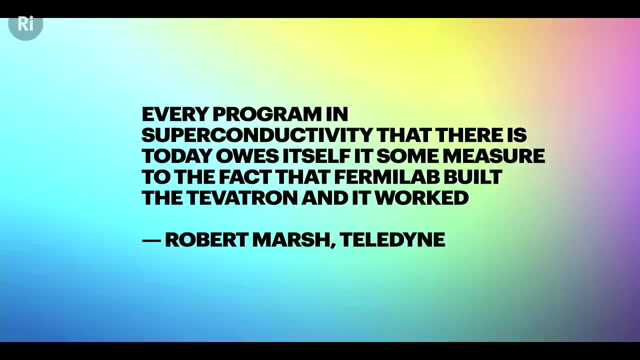 says that every programme in superconductivity that there is today owes itself in some measure to the fact that Fermilab built the Tevatron and it worked, And it is quite incredible. And the Tevatron also helped us understand the different pieces. 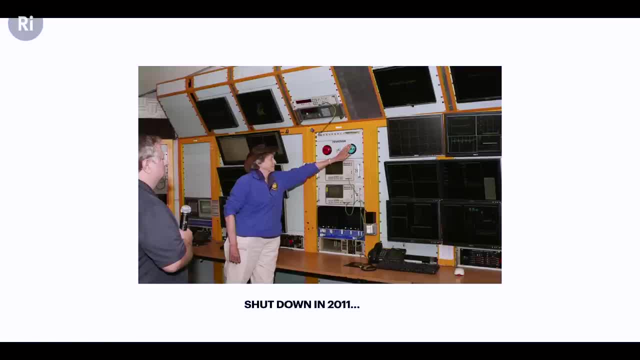 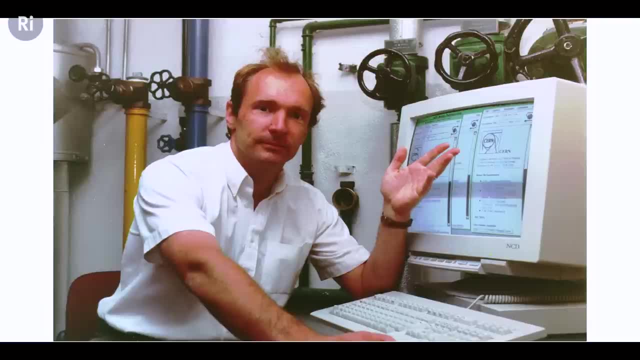 of the standard model of particle physics, at the end of which, in 2011,, Helen Edwards was the one who switched the machine off. Now, for the sake of time, I'm going to rush through to the end here, but there's so many other ways. 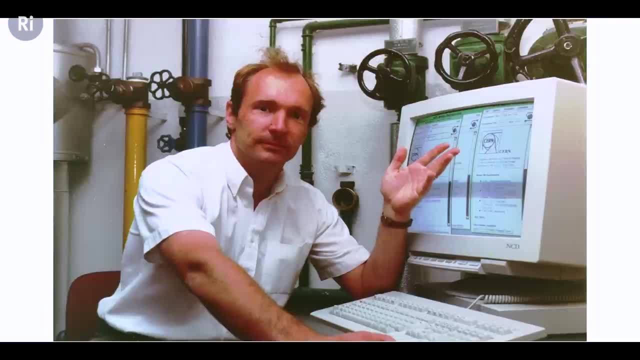 in which these enormous experiments have affected our world, And there's one that I would be remiss not to mention, which is that Tim Berners-Lee, working at CERN- the predecessor to the Large Hadron Collider- was the one who actually invented the World Wide Web. 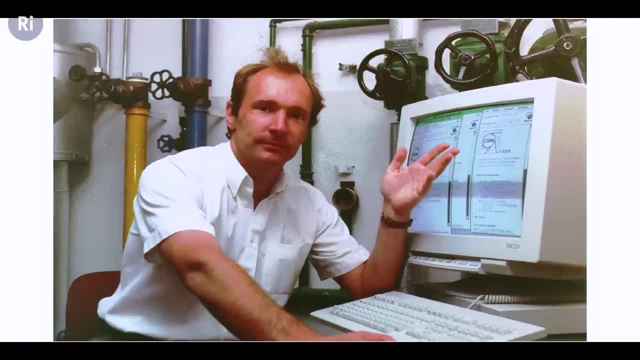 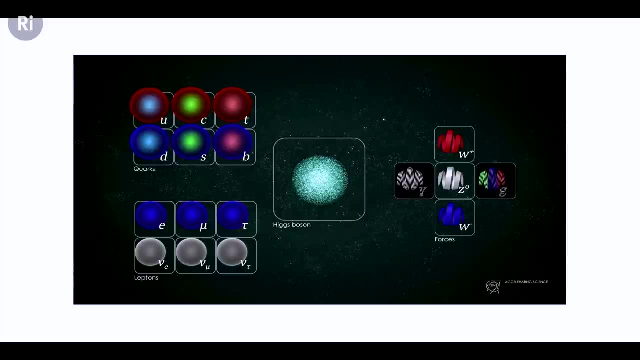 which, if we now talk about using the internet, we actually talk about using his inventions. So hopefully you can see that by bringing together this collection of fundamental particles and these equations, which we now understand to be how our universe works, on a fundamental scale of particle physics, 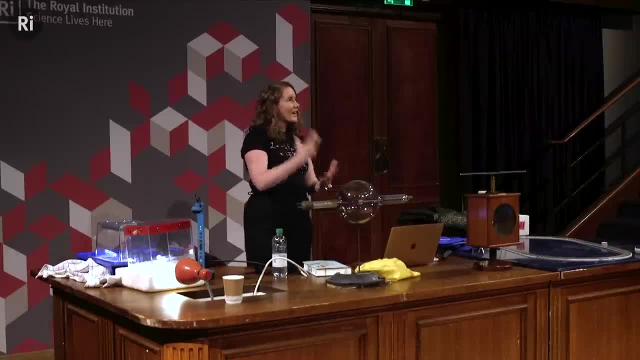 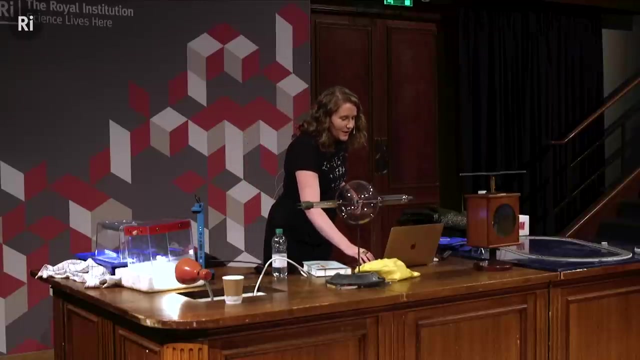 we've also been working on the cutting edge of technology And, as a result, even though what we're doing with no application in mind, is very much curiosity-driven, it's had an enormous impact in society, And that culminated most recently. 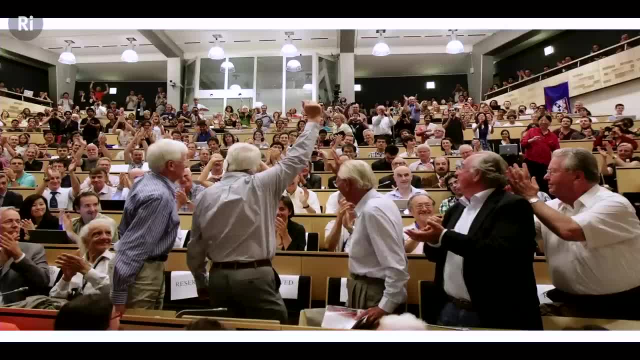 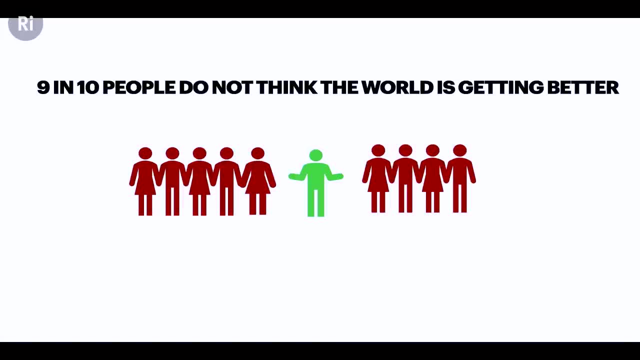 in 2012, with the discovery of the final piece of the puzzle, which was the Higgs boson. But despite all of this, nine in ten people do not think the world is getting better, And this was before Trump and COVID and everything else right. 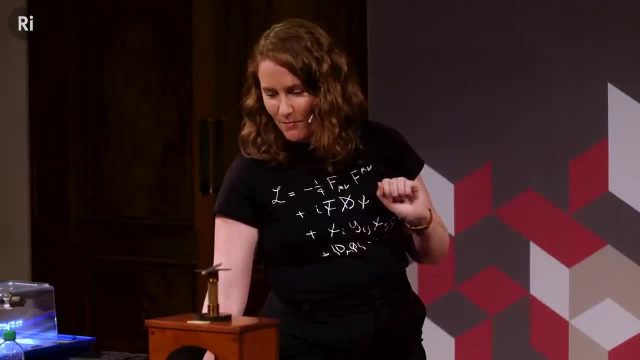 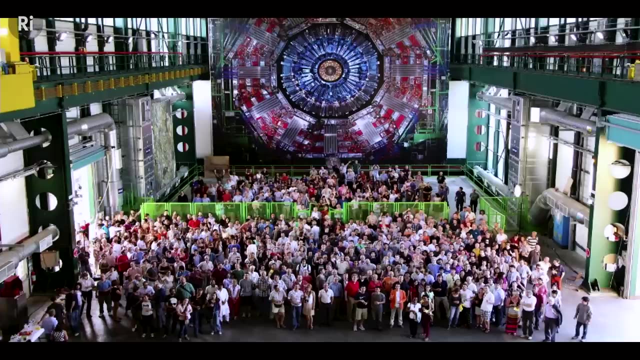 And I'm just going to skip over that one. but one of the key things I learnt through interviewing all of my colleagues in the field about this is when I asked them what people could learn from this experience of particle physicists working together to overcome these enormous barriers. 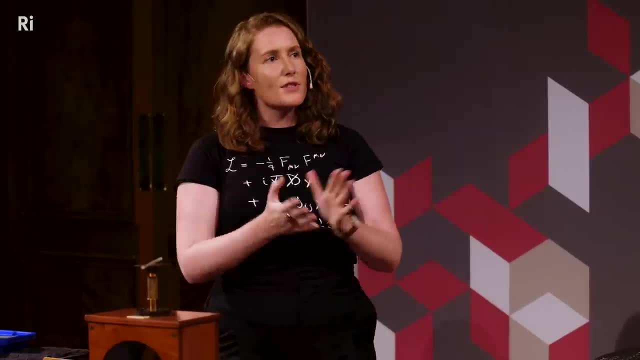 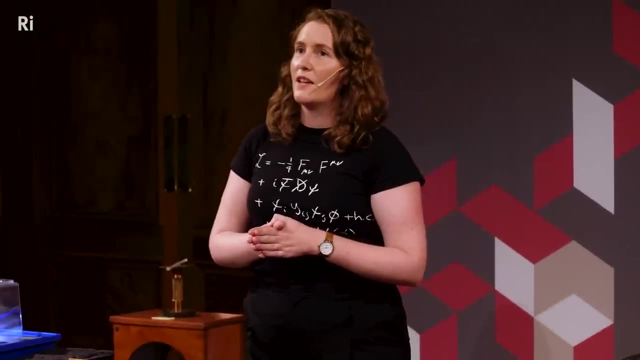 and these enormous experiments. I expected them to say lots of different things, And they all said the same thing. They all said that people can learn how to collaborate, And I think, therefore, what I didn't realise when I was writing this book. 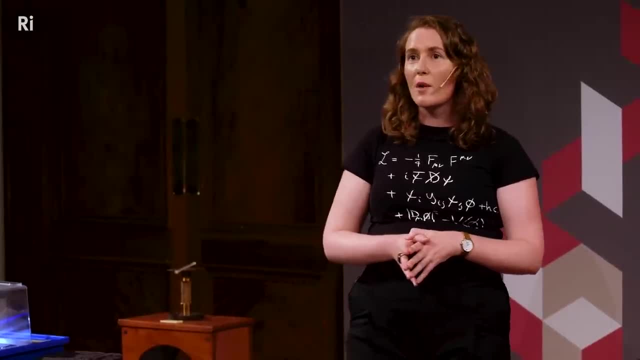 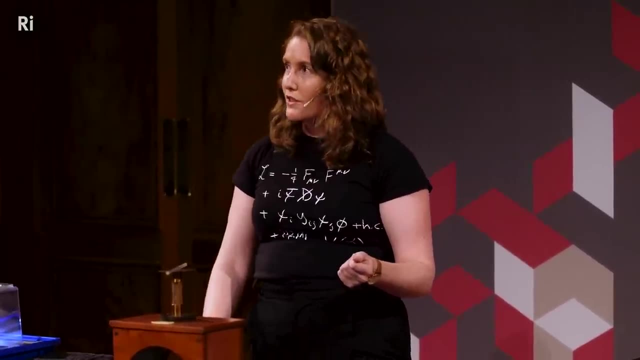 is that I was writing a book about hope of how we might be able to work together in the future to overcome the enormous challenges that now face us, And in studying collaboration, these are the key things that come up about what works. 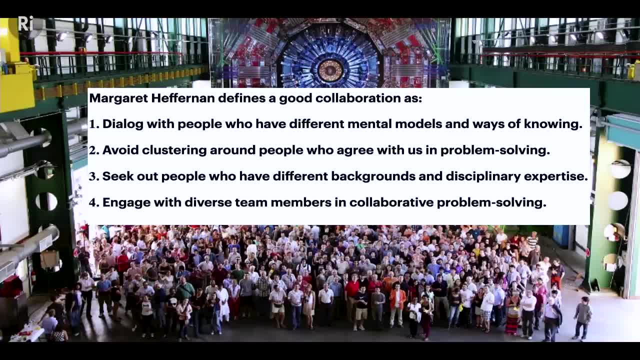 And so these are some takeaways for you, which is to talk to people who have different mental models or ways of knowing. to avoid clustering around people who agree with us, especially in problem solving, but also- that probably applies to social media- to seek out people. 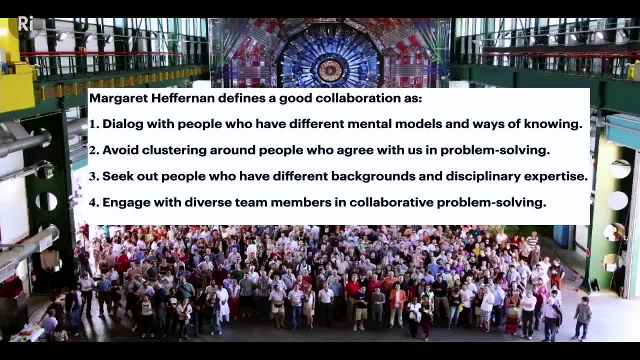 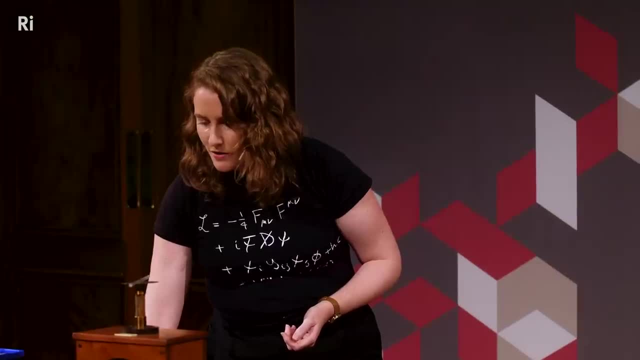 who have different backgrounds and disciplinary expertise. so multidisciplinary, interdisciplinary work is key to good collaboration and to engage with diverse team members in collaboration and problem solving. And so some of the three. Well, I really distilled all these experiments over 120 years down to three key things. 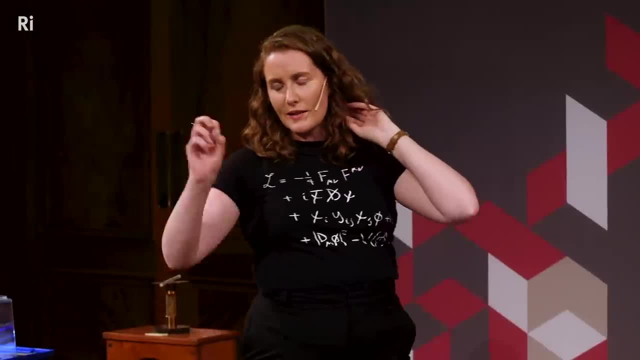 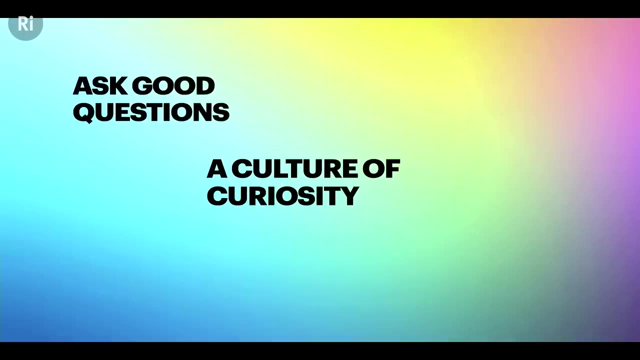 that I think all of us can take away about how we can use this search for knowledge to change the world going forward. And one is to ask good questions. The other one is to build a culture of curiosity where people are allowed to ask these questions. 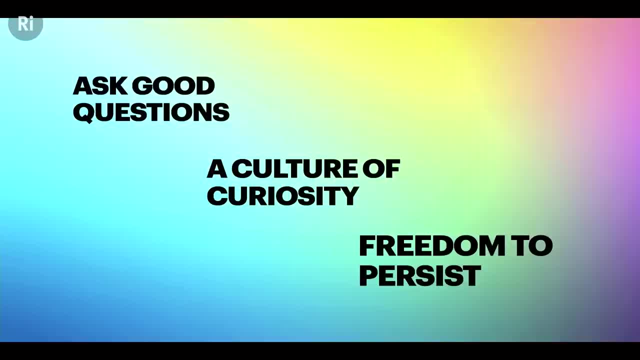 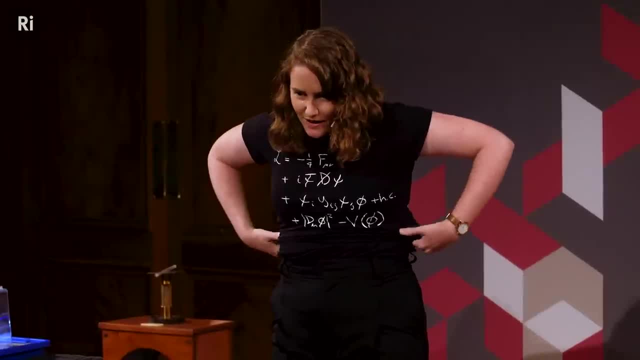 and are supported in it, and the freedom to persist. Now, I know I'm standing here wearing a T-shirt with particle physics equations on it, but I think, especially given the week we've had in the UK with all sorts of comments about girls and physics- 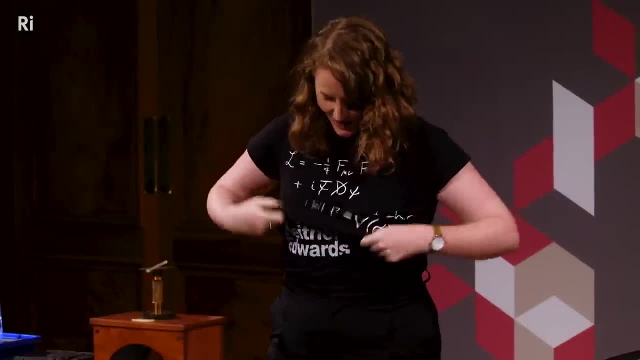 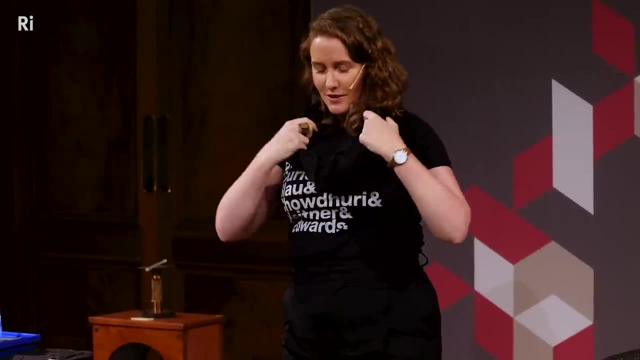 and all this rubbish. what I want us to acknowledge and remember is that there's more than meets the eye in terms of these experiments, right? So I want to show you. I was going to do this out the back, but for the sake of time, I've done it live on stage. 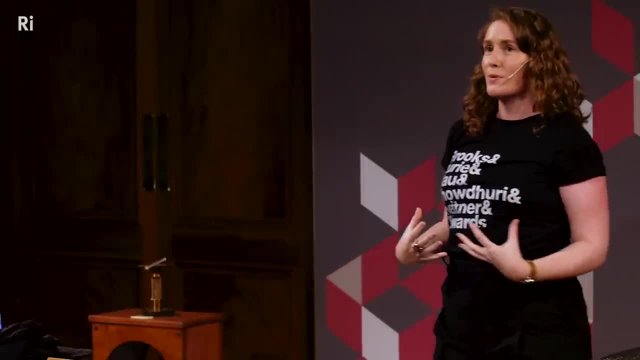 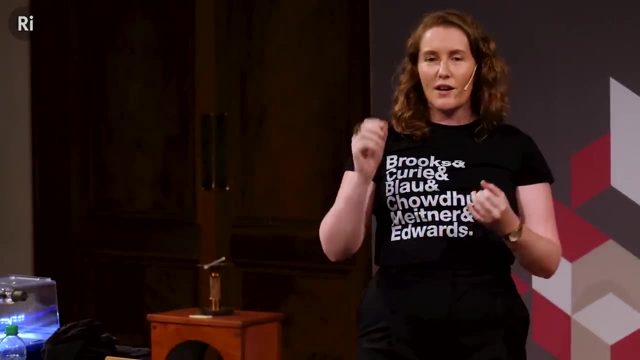 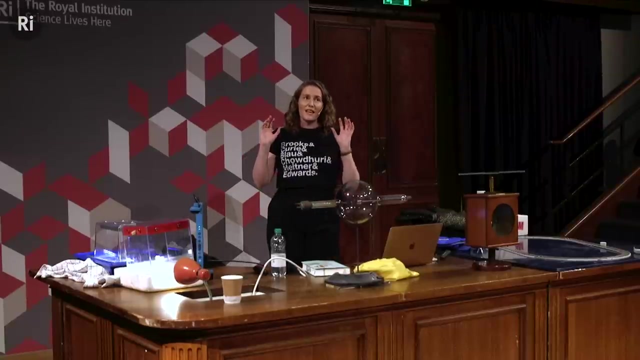 This T-shirt that I've made, which highlights these people, these women, who I've talked about mostly in this talk, who were behind this story of discovery. So creating environments where people can thrive, all people can thrive, I think, is really going to be the key. 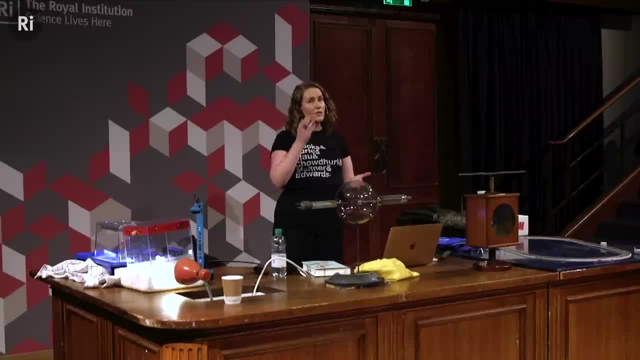 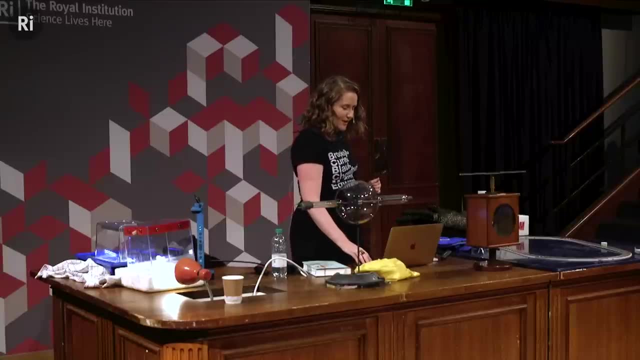 to unlocking those future discoveries which are going to change our world in ways that we cannot even yet imagine in the next hundred years. And I will finish there because I'm over time and take some questions. Thank you so much for your attention.